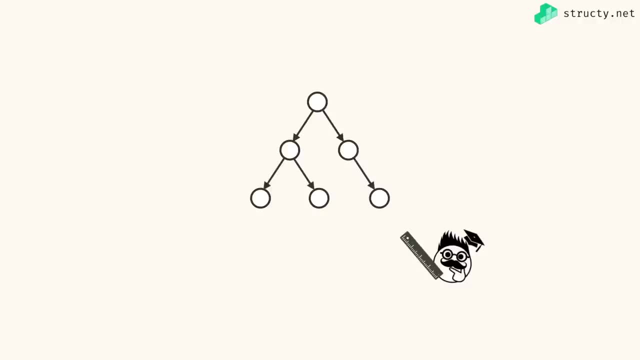 it does show that you have proficiency dealing with the data structure. we could store values within the nodes of our tree. For now I'm just going to put some letters. When it comes to your programs, you can store any type you want. you can store integers, numbers or even other objects. So because 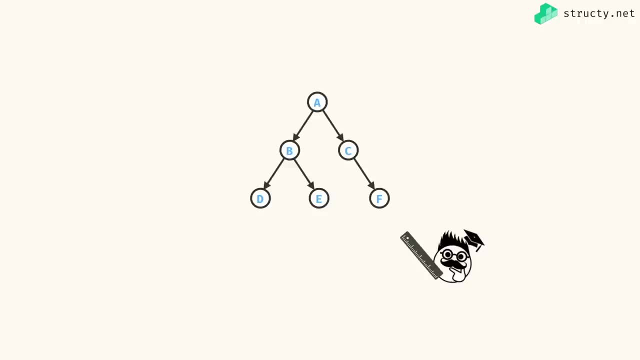 we have a tree we like to use familial relationships, In other words I think of like a family tree, right? So if I look at node B, let's say I call them the parent. If B is the parent, I know the children of B are just the D and E nodes. right, parent and child is like a. 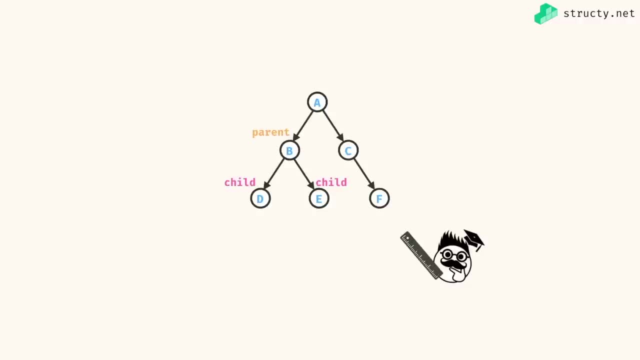 relative relationship. Let's say I kind of changed my frame of reference And let's say I looked at a as the parent. Well, in that scenario then, B and C are the children of a right. For the case of the C node, if I think of CS and parent, it only has one child, its lone child being the F. 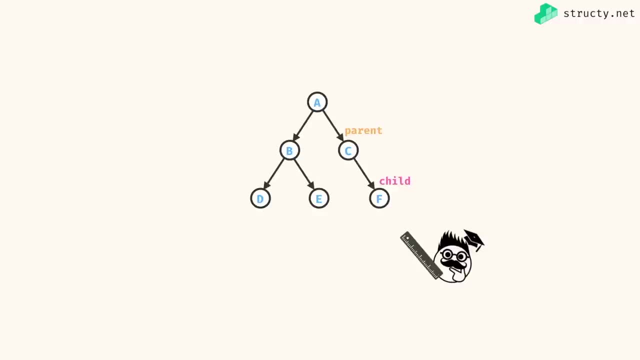 node, So feel free to use that parent- child relationship when describing the relationship among nodes within a tree. Another term we'll use a lot in the context of trees is the word root right. So a root is going to be a node that has no parent. So in this tree, a is 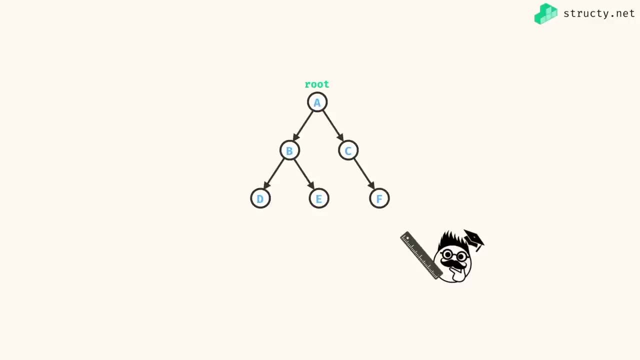 the root, because a has no parent right. There are no arrows going into the A node. On the flip side of that, if I look at the nodes D and F, we call them leaf nodes. a leaf node is a node that has no children right. So 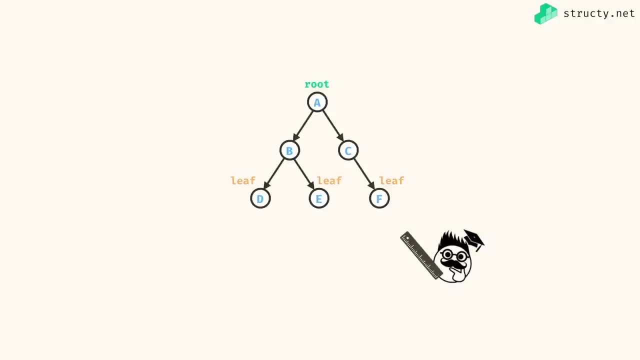 D and F have no outgoing arrows. Typically in a binary tree we're going to have a single root. we could have many leaves. One thing you'll want to be sure to do is make sure you generalize your understanding of a leaf right. So in this particular example, looks. 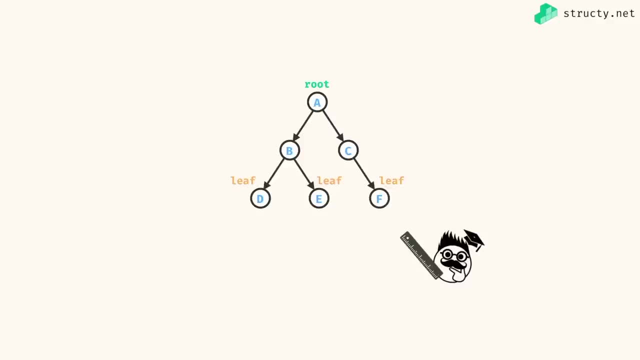 like, every leaf is two edges away from the root, counting the number of arrows from the root to any leaf. It could be the case that my leaves occur at different levels, right? So I removed that F node, which case C is now a leaf, right, Although a C is on like a different level. 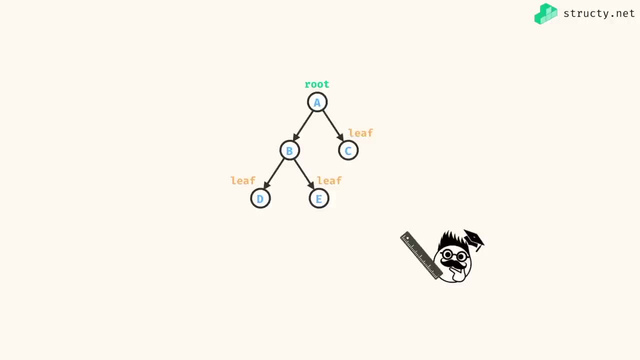 than D and E. it's not the bottom most level. it is a case that it's still a leaf right. A leaf node is just a node that has zero children, Alright. so with all of those terms out of the way, let's hone in on the real topic here. right, I talked a lot about trees, But really, 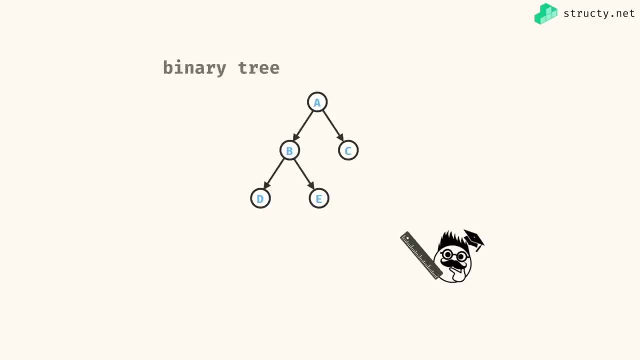 in this course I want to go over the basics of binary trees, right? So let's look at that binary part to begin with. So let's look at that binary part to begin with. right So let's look at that binary part to begin with. that's really a dead giveaway. We know binary. 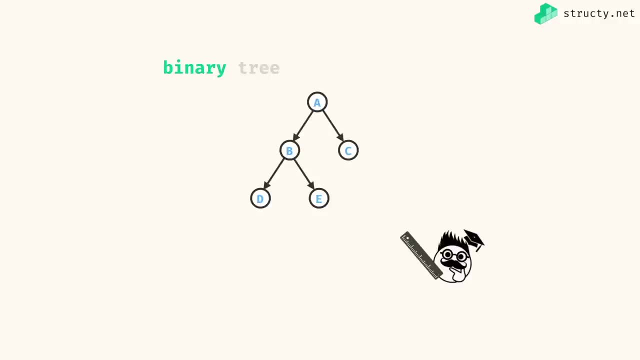 has to do with the number two. a binary trees, a tree where every node has at most two children, right? So currently on the screen I have a binary tree. if I gave a another child, let's say a third node over here of F, this would be a tree but not a binary tree, right? 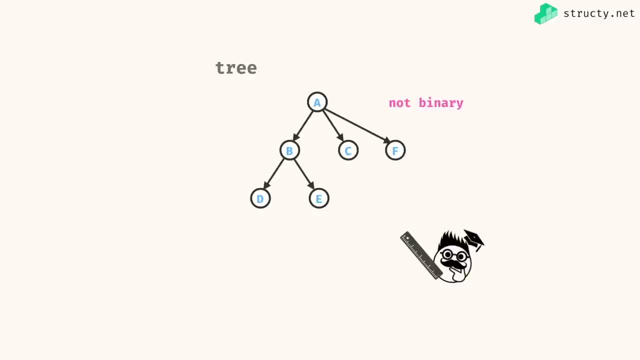 would be like a ternary tree because I have at most three children. So let's say I kind of remove that extra note. Now it's back to a binary tree And it could be the case that a node has less than two children, but still be a binary tree, right? So if I gave C just 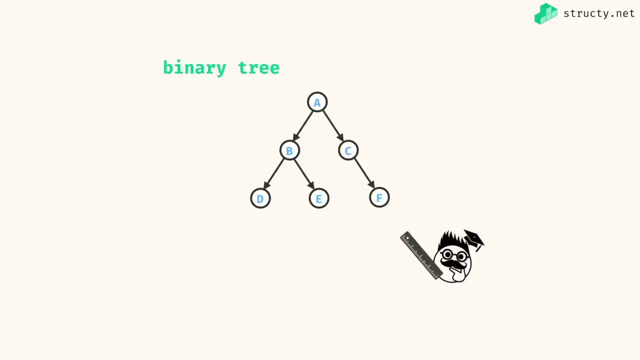 a child of F. this is still a binary tree, And so if I look at any node within my tree, that node will have zero, one or two children, and no one has more than two children, right? So you'll want to be sure to remember that a node in a binary tree could have less than 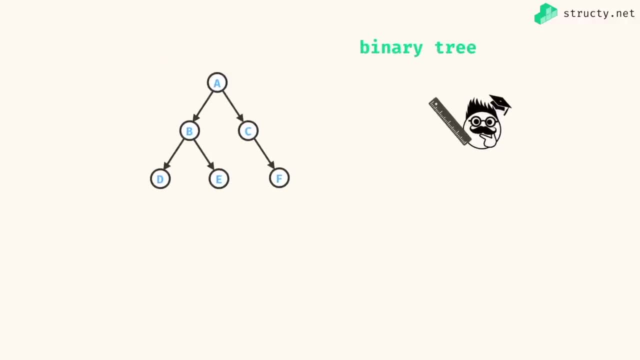 two children Alright. so that'll be the first criteria for understanding what a binary tree is right. It's probably the easiest criteria: at most two children per node. We'll also want to be sure to add into our definition: to have a robust understanding is to also 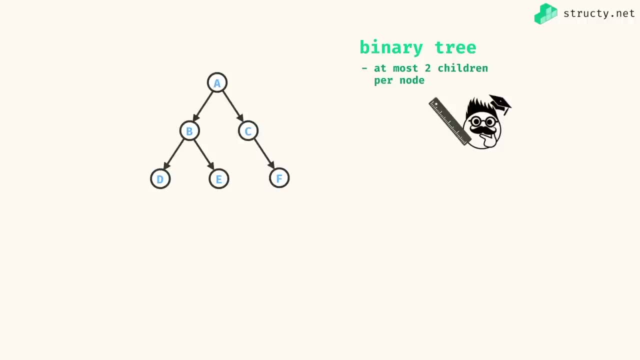 remember that, at least for us in computer science. we think of our binary trees as having exactly one root, meaning there should be only a single node that has no parent right. Typically, when we draw it it would be like the top most node. So right now this is definitely. 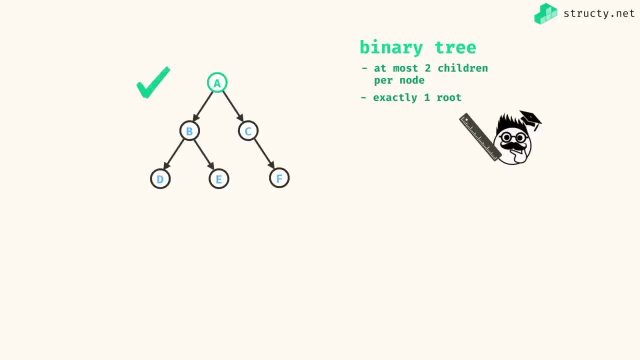 so far a binary tree. If I had some other node in this drawing like G- right, G also has no parents- I would no longer consider this a classic binary tree, right? So watch out for that. Let's go on to our final criteria. We also need one more ingredient, And that's exactly. 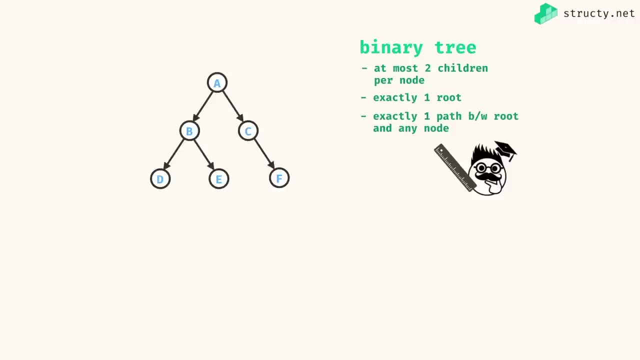 one path between the root and any node right. So looking at my example to the left, this is indeed a binary tree that meets all three criteria And let's say I chose the root and any node. obviously there's only one route, So we're definitely considering the a node. 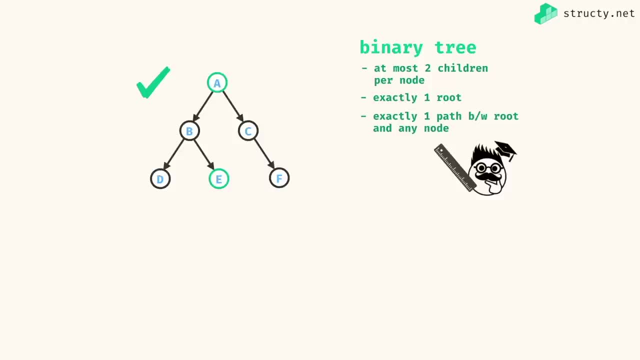 let's say I chose some random node like E. this is really a binary tree- then we're guaranteed to have only a single path that connects A to E. a path is really just a series of connected nodes I can travel through right. So to get from the root A to the node E, I can go. 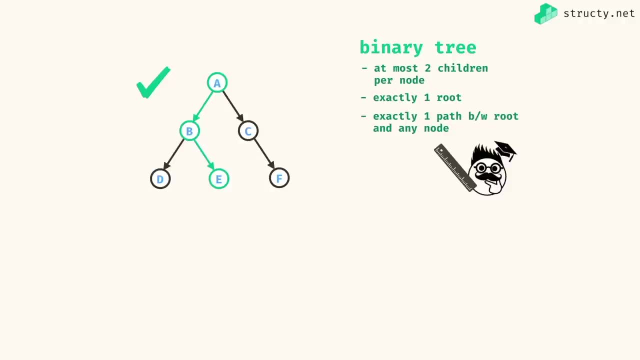 from A to B to E, And that would be one path, And that's the only way to get from A to E. That's what I mean by exactly one path. Let's say I chose another node, like F. there is also exactly one way to get from the root to F, And that's just ACF. that would be the 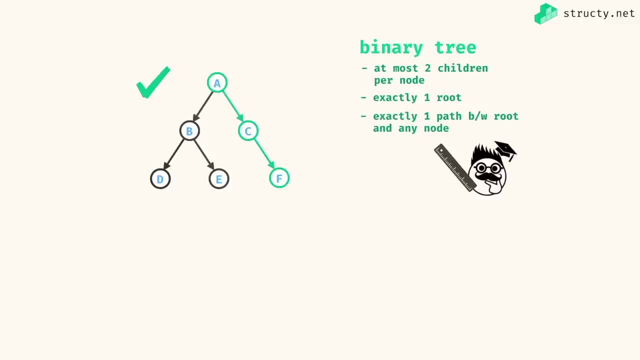 only path. If I added some additional connections or edges within my tree, I can get a scenario like this. this would no longer be a binary tree For one. we can see that B has three children but also does not have a unique path between. 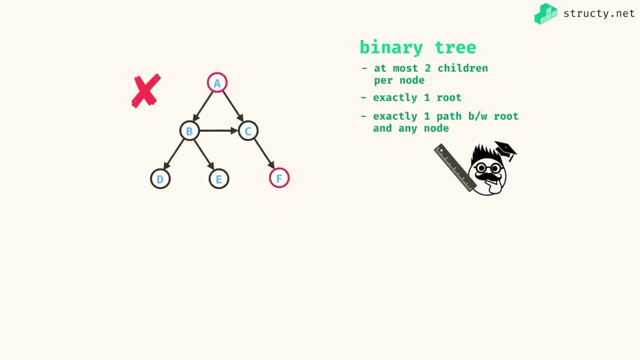 the root in any node. For example, if I chose the root of A and the node of F, one way to get there is by going ACF, But another way to get there would be ABCF, Right, And so do watch out for all three criteria when you're considering a binary tree. Awesome. 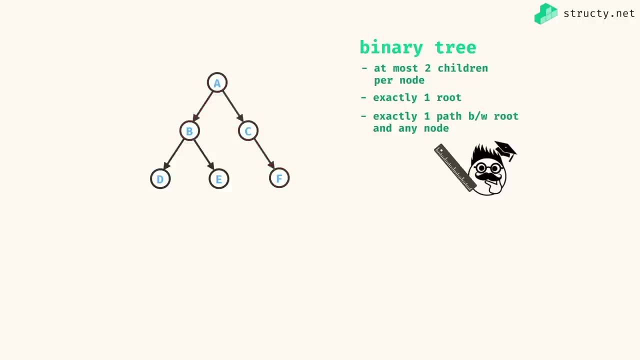 So let's look at some smaller examples, And this is where I think some students tend to struggle with their understanding of binary trees. So if I took out some nodes over here, this would definitely still be a binary tree, right? just looking at our different rules. 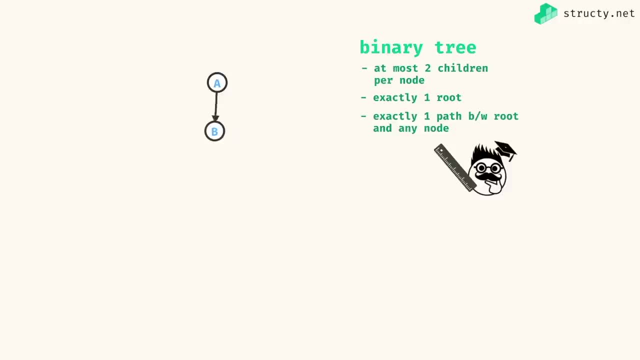 Right. Let's say the root, node A only had one child would still be a binary tree, right, Because the binary tree only demands that we have at most two children. we still have one root and we still have only one path from root to any node. Let's say I have the 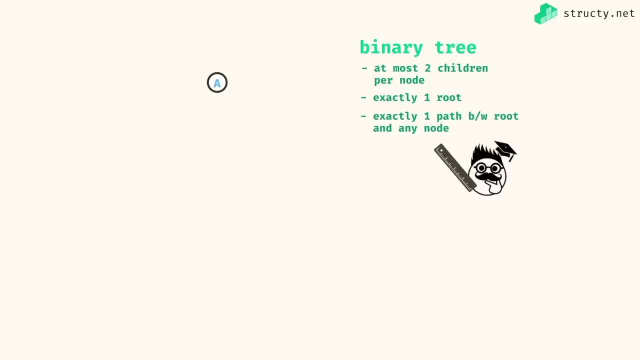 smallest tree that has a node, which would be the singleton tree. this is still considered a binary tree. right has one root. there's not really any paths to be had here except itself, And every node does have at most two children. here we have zero children, right. 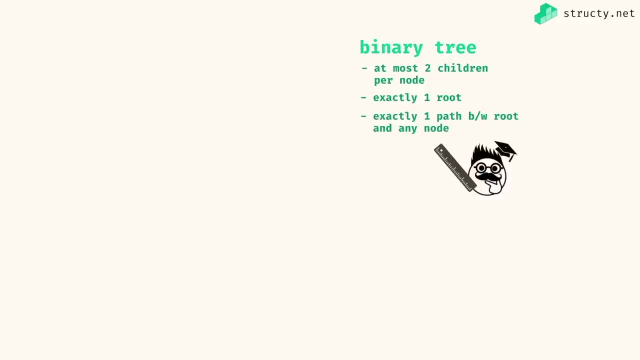 The final edge case we want to think about is what happens when we have no nodes right. we consider this as the empty tree. this is a very special case And we should consider any empty tree as actually being a binary tree. that's going to be very useful when 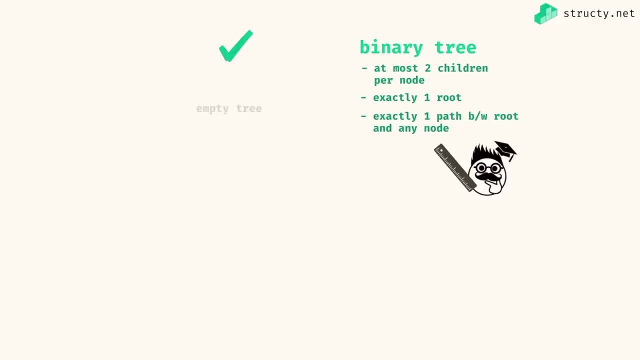 we come up with some algorithms later on, right? So a common edge case I have to consider is what happens when we have an empty tree, that's, a tree with zero nodes, right? Let's look at another example. Let's say I had this structure. to take a moment, look at it and see if this meets. 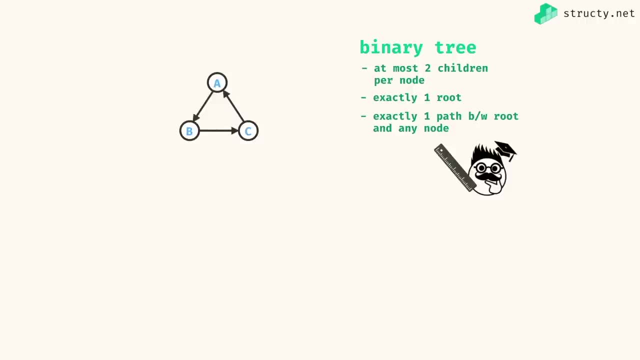 our criteria This would not be considered a binary tree. So if you look at your different criteria, looking at the first one, it does have at most two children per node, so that's okay. But we can't identify exactly one root here. Remember that a root node is a node. 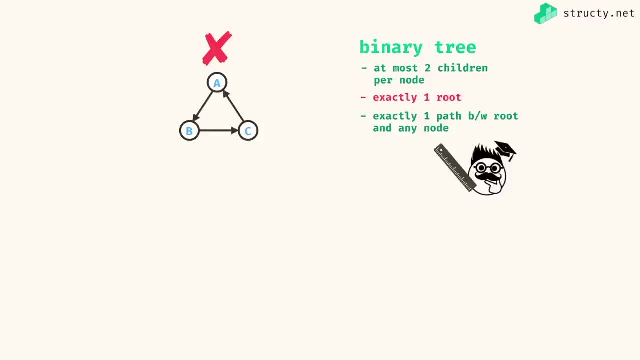 that has no parent right. If you look at every node in this picture, every node has exactly one ingoing arrow. So that means every node has at least one parent Right. So it doesn't meet that criteria And furthermore, there is not exactly one. 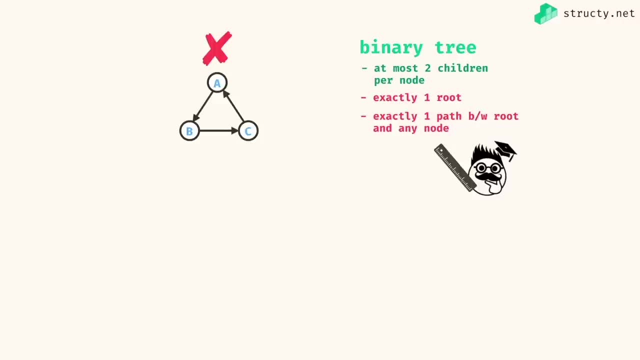 path between the root and any node, because we have a cycle within the structure. So, for example, let's say I was starting at a right and I wanted to travel to see. one way to get there would be to go A, B, C. that would be one path, But I could also have another path. 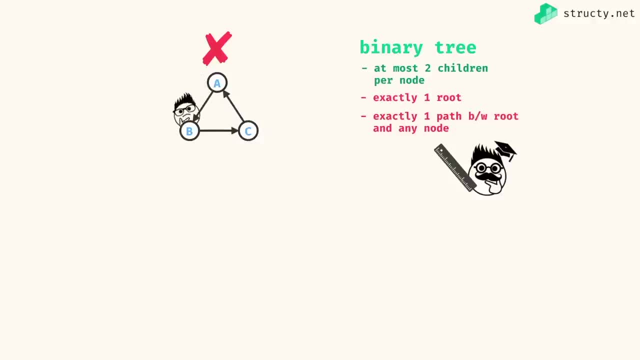 where I just go around twice and go A, B, C again. there would actually be an infinite number of paths in this scenario. Because of that, this is definitely not a binary tree. So let's look at another example. So let's say I have an empty tree and I want to take a moment to look at this one. So let's say I have an empty tree and I want to take a moment to look at this one. So let's say I have an empty tree and I think it looks like it's an empty tree where I can see it in any node. 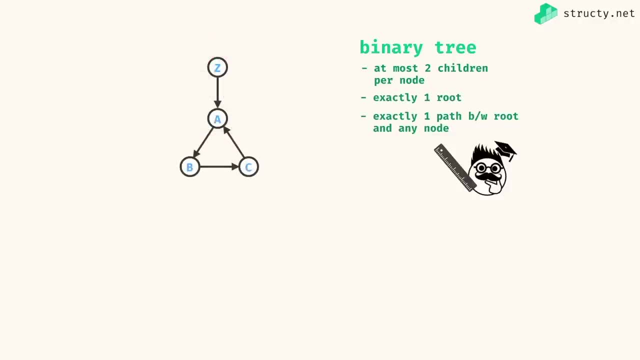 And finally we've got a binary tree, And there are kind of many reasons for that. Had a different example. Looking at this one Now, I meet criteria one and two right. I have at most two children for every node, but I also still have exactly one root node. 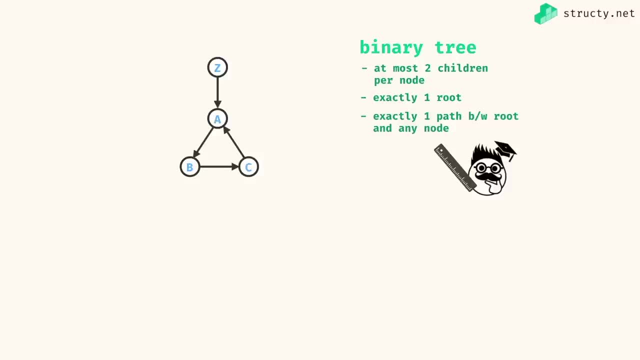 here I will consider Z, the root node. However, there is not one path between the roots in any node and because I have that cycle, So these rules are really worth remembering. they're really going to help you solve on much more difficult binary tree problems. 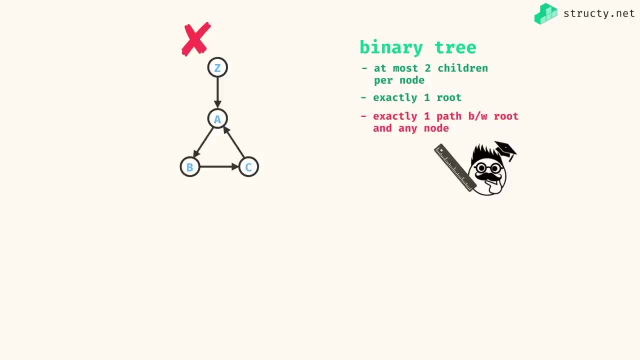 And if you remember these three rules, you can identify a different problems in a binary tree-enticed binary tree, And here's how fun it is, So let's Good job there. we are binary tree framework, In other words, the hardest problems that you'll encounter in. 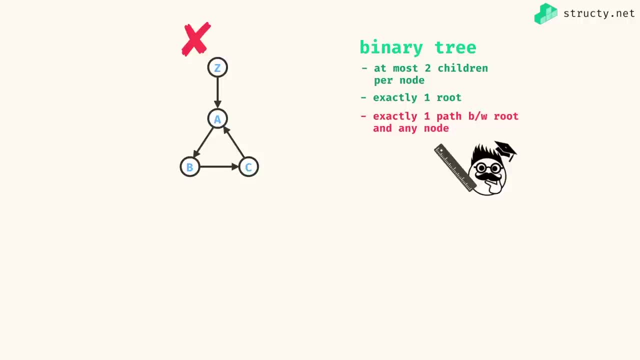 your interviews are problems where they don't tell you straight up what data structure you're dealing with. you're gonna have to notice the pattern. In other words, what if I gave you some structure like this? take a moment and figure out if this is a binary tree, If 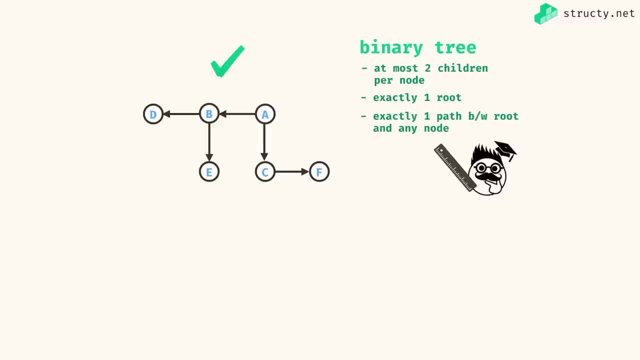 you look closely, this does meet all of the three criteria to be a binary tree. I can just treat a as a root because it has no parent. I can treat nodes D, E and F as the leaves because they have no children. I just drew this in a pretty interesting way, right, If? 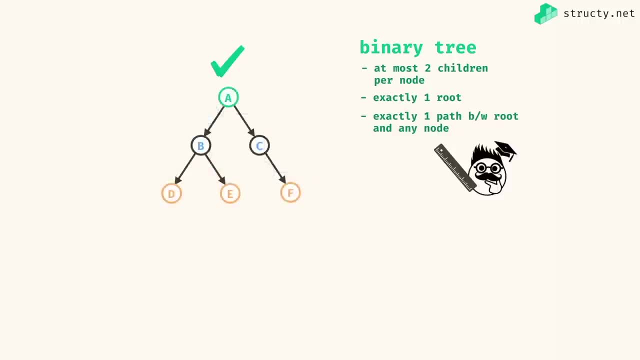 you rearrange things in a classical binary tree sense would look like this: More importantly, this has the same relationships as the previous drawing. I just drew it in a top down fashion, right? So, no matter what, do understand these three rules for a binary tree, right? Because 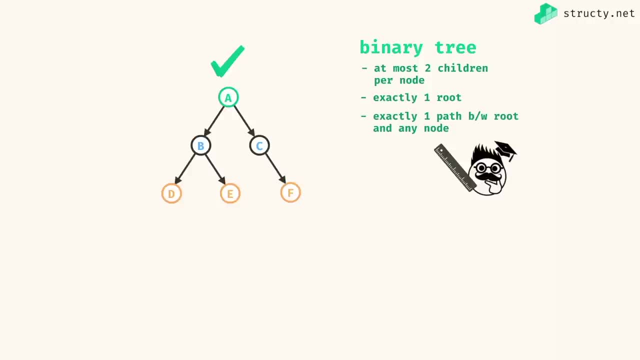 sometimes may not be as explicit as a nice triangular shape drawing, Awesome. So we talked a lot about the theory of how to you know, look at and reason through some binary tree definitions. Let's go ahead and start to talk about how we could. 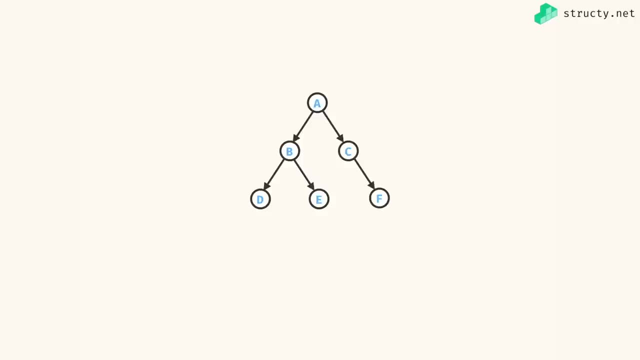 represent a binary tree programmatically. In other words, how can we do this in some code? Well, no matter your programming language of choice, I think you're going to represent these as objects. In other words, every node here is going to be some objects, So it could. 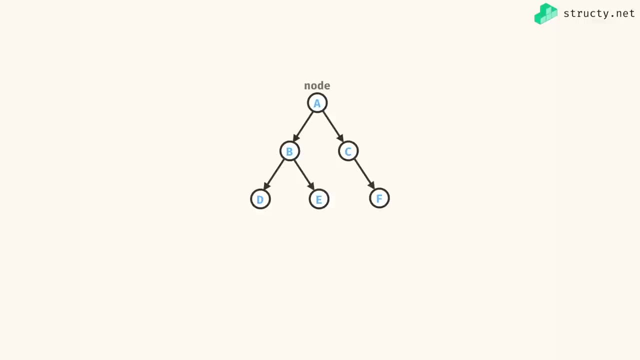 be like an instance of a class. the properties only to store within this object would be the current value. So I need something to store like the A of my current node. But I also need to refer to some children, So we'll also need some left and right pointers to 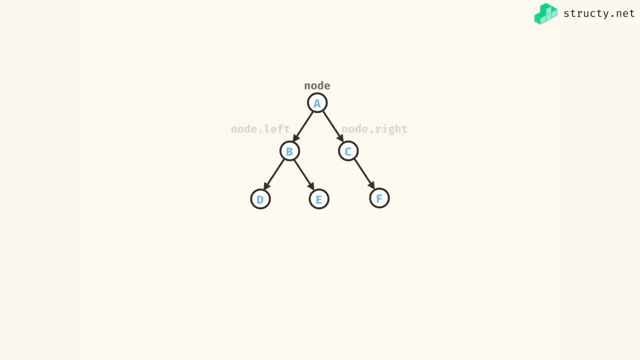 the children right. Those are just going to be some properties on that object And a classic binary tree is very common to refer to the two children using a left and right direction. Notice that some nodes here, like the C node, they're only going to have one. 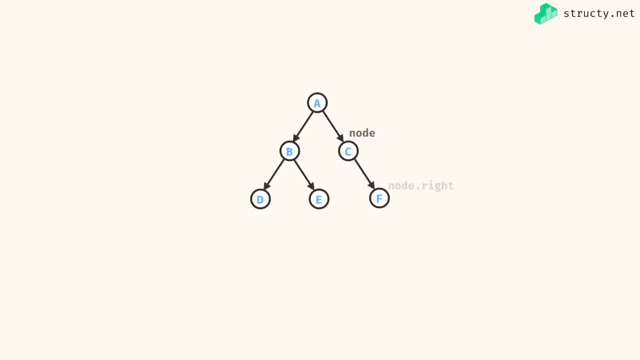 child right C only has a node dot right. it does not have a left. So we're gonna have to use some empty value like null or undefined to represent a child that doesn't exist right, Especially for a node like he. he has no left and also no right, So what we'll do, let's. go ahead and hop into my text editor and I'll show you how you can do that. So let's go ahead and hop into my text editor And I'll show you how you can do that. So let's go ahead and click on the left and right pointer, And then you can see that the child is not. 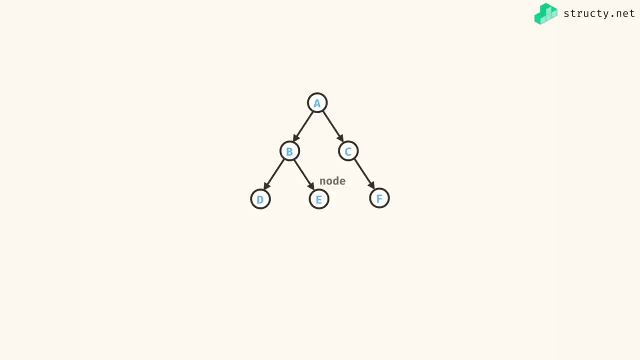 a child. So let's go ahead and click on the right pointer And then you can see that the child is taken. so let's go ahead and click on the left pointer And then you can see that the child is taken. so let's jump into my text editor And I'll show you how you could represent a binary. 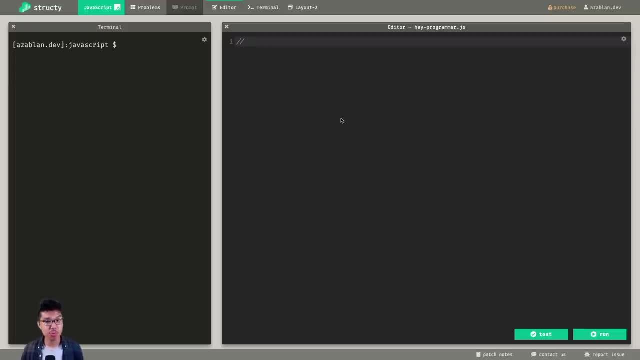 tree programmatically. So transition. here we are in my text editor. Let's start by creating our node class right, So you'll be able to follow along any language that you choose. I'm going to do mine in JavaScript, right, So I think the best way to represent a node 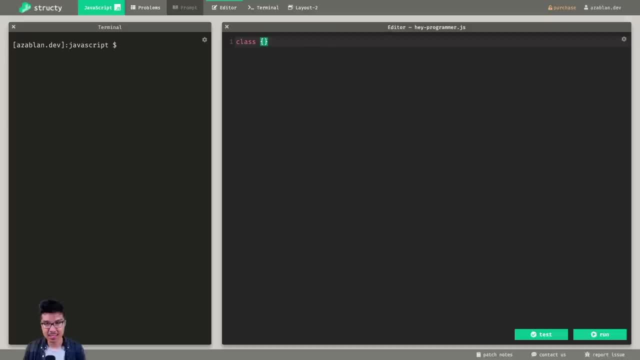 is just to use some class. So hopefully you're familiar with some classic class syntax. let's create a node class. I'm just going to need a quick constructor And I think would be valuable to take in the initial value that's going to. 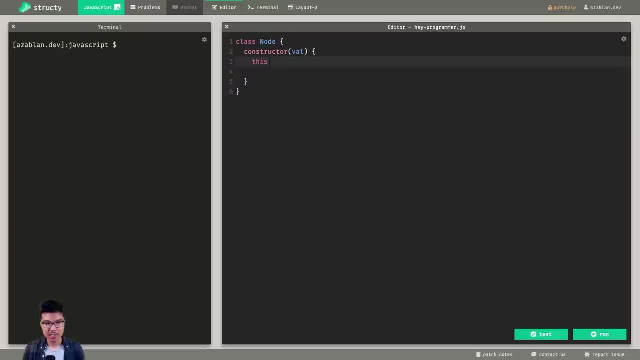 be stored with a node class And I think that would be valuable to take in the initial the node. So I'll take the in as a constructor argument. I can just set this dot val to that value And also need two more properties, one for my left, so I can say this dot left. 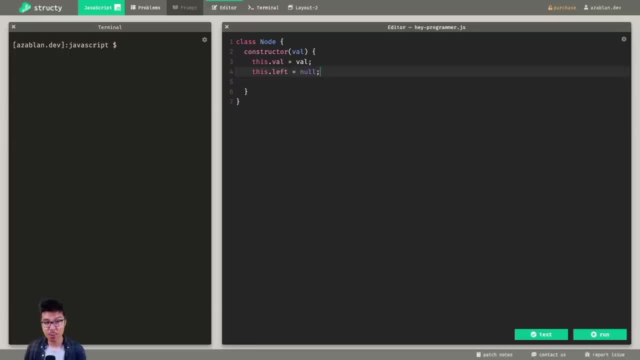 I'm going to initialize it to null. that means, by default, a node will have no left child. the same way, by default, a node will have no right child right. So I'm going to use null to represent children that don't exist over here. Awesome, That's all you need to create, you know? 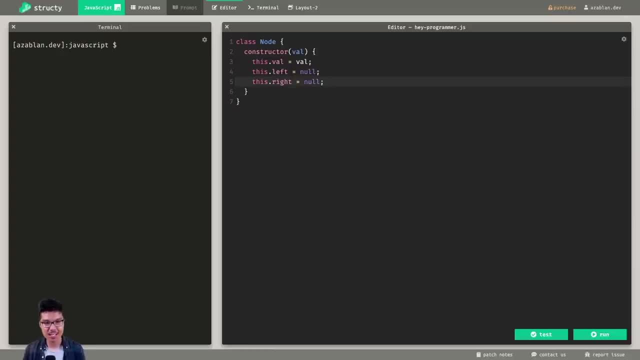 a baseline binary tree, right? We're going to use this class a lot during the course to test our algorithms. So how can you create a node and eventually wire up a tree? Well, I'll just call my constructor a few times. I'll create different nodes, I'll just store them to some variable names. 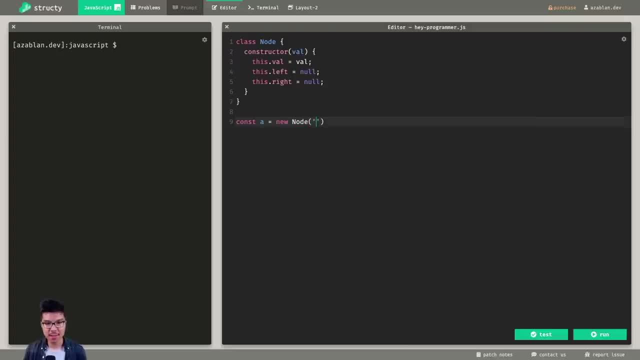 And, of course, say new node, to create a new instance of node, And I'll store some value inside, I'm going to store some characters inside, I'll create a bunch of these different nodes. What we'll want to be sure to do is make sure that you also set their pointers properly. 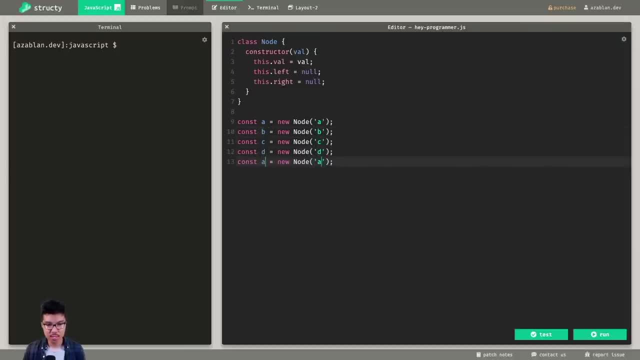 So I'll give each of these some different values- A, B, C, D, E, also do F- And then I'll just manually, for now, set their pointers properly. So what if I did syntax like this, like: since I'm in JavaScript, I can easily assign these. 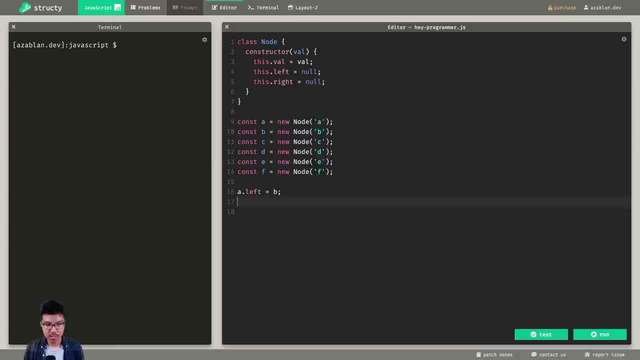 pointers. I can say A's left is going to be B. I can say A's right is C and also say B's left is D And then B's right is E And maybe finally I can say C's right is F. 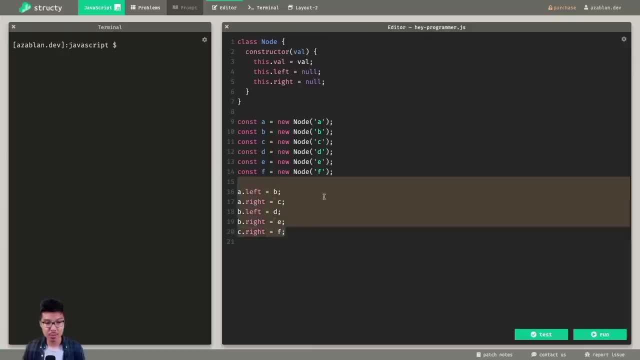 So by doing these assignments I'm connecting some nodes together. I should end up with a structure like this: right Have a as a root, because nothing points day. A has no parent, But A has two children of B and C, And then, along with that, B has two children of D and E. 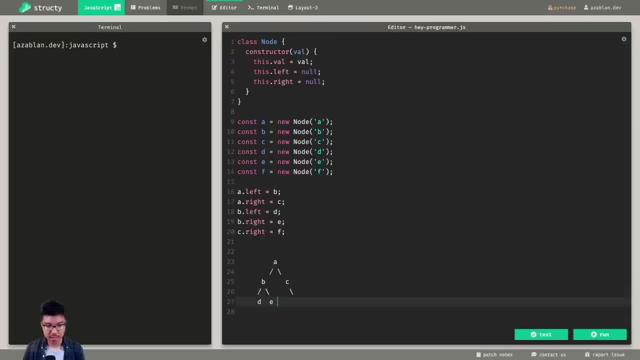 Finally, C just has a right child of F. This is actually the same tree that we looked at a lot during the whiteboard session, right? And this is how you can represent that same tree programmatically, right? So I always think it's valuable to also try to visualize your trees, right. Obviously, we create this. 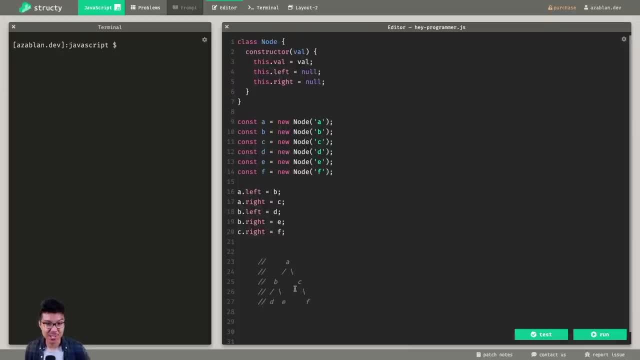 tree in a very manual way. probably in the long run we'll create applications to just maintain and create trees dynamically during some input, But for now we'll start by creating all of our trees in this very kind of static way. Right, And so with that, now that we 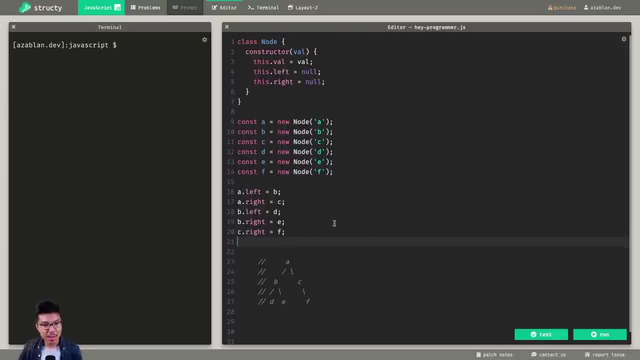 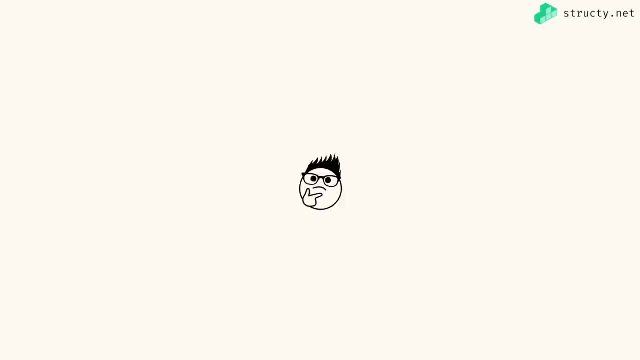 have an understanding of how to represent a binary tree, let's go ahead back to the whiteboard And I can show us our very first algorithm. Hey, programmers, Alvin, here, right now I want to go over this depth first values problem. 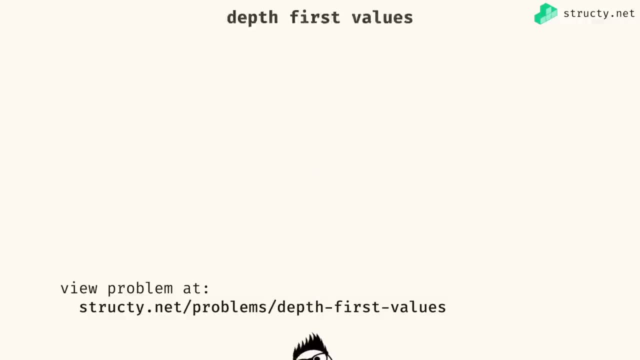 This will be a good review of the depth first traversal algorithm. So what do you want to do in this problem? Well, what we want to do is take in a binary tree. in particular, your function is going to take in the root of the binary tree, And just recall that given. 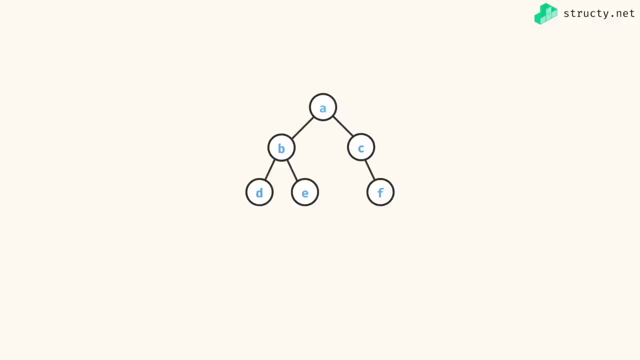 the root node of a binary tree. we know that that node is going to have pointers to its left and right children, which may point to other nodes. However, let's say a node does not have a left or right child, then it's point is going to be: 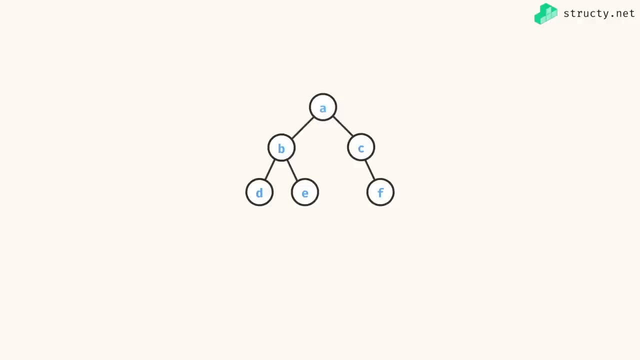 set to null. So that's how we represent our binary tree programmatically. But for now let's just stick to the visual representation of our tree. So for a depth first traversal we could start with the root node of a. what we'll do is: we'll just add that to some collection. 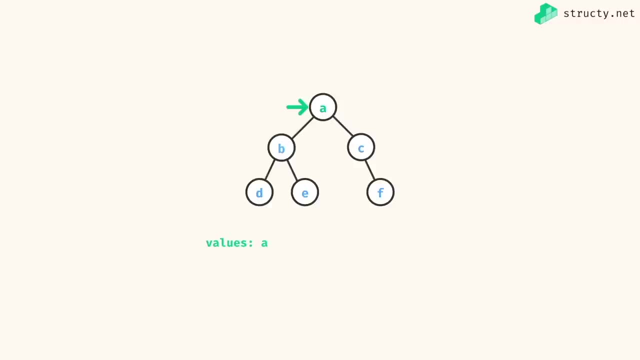 And we're going to have to maintain these in a very particular order. Then from there, according to a depth, first traversal, I could go to B, And here's where we make our really important decision right: we can either go to C or D. 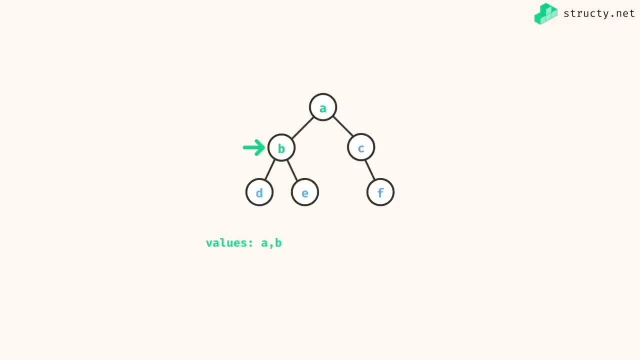 If I'm doing a depth first traversal, I need to go deeper in the tree before I move laterally. So that means I go from B to D, And once I bought them out at D, there's nowhere deeper I can go from D, And so now I move laterally to the E node, And this pattern continues. 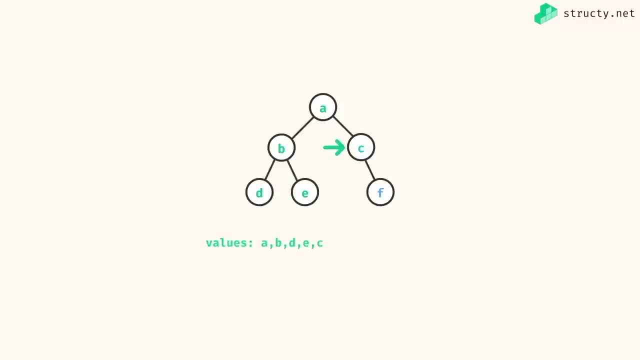 right, I don't have anything deeper from E, So now I go to C And then from C I go to F. So this would be a depth first traversal on this binary tree. Notice that it goes ABD, ECF, And the characteristic is we must go deeper in the tree until we can't anymore, And then 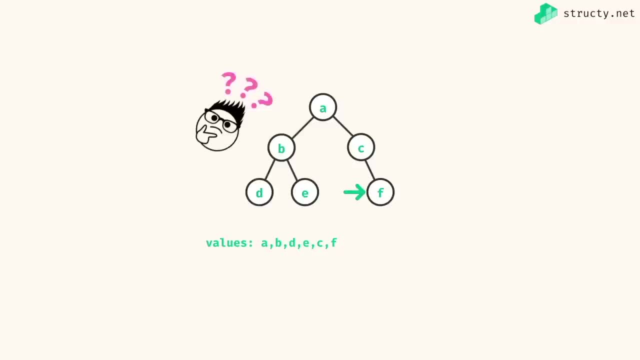 we can go across the tree. That being said, how can we actually manage to implement this algorithm? If you're familiar with depth first, traditionally, then we know that it's going to use a data structure like a stack. So let's get situated over here, So we'll trace through. 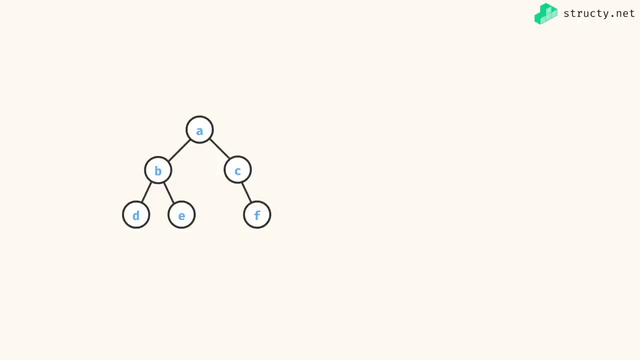 that again, But this time taking a really close look at how we can use a stack to accomplish that direct order. And so just recall that a stack is a sequential data structure where we can only add things to the top of the stack and remove things from the top of the stack. 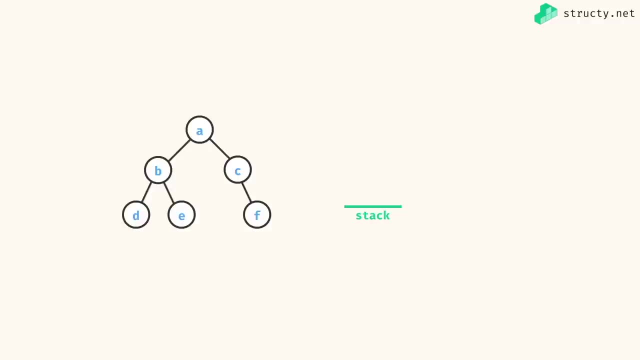 So really important characteristic is we can't really insert or remove elements from anywhere but the top of the stack. So when I add things to the stack, I was added to the top, like this. When I remove things, it's also from the top, like this: Alright, so when 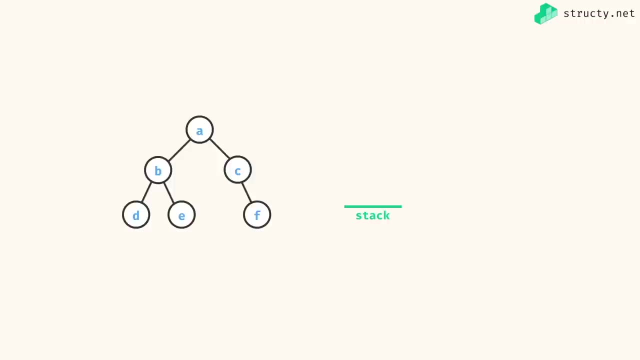 I begin at this depth. first, traversal algorithm. I'm going to start with the root node of A And by default I really just take that root node, I just store it on my stack And I'm going to start by removing or popping the top element on my stack. So it's the only thing. 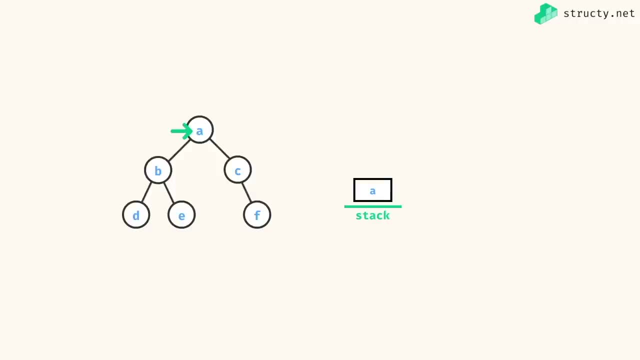 on my stack. right now I'll use these rectangles represent my different stack frames And really in my program that would just mean storing the actual instance of node or some pointer to it. Cool, And then from there I actually begin my main algorithm. So the main flow. 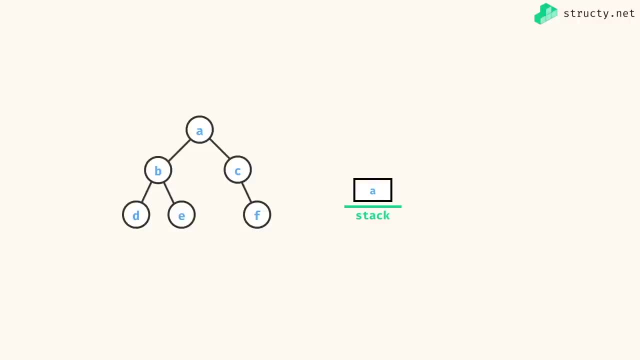 of a depth. first reversal will check if the stack is empty. Right now, the stack is not empty because I have at least one element, And so what I do is I start by removing or popping the top element of my stack. So I'm going to remove a and I'll label that as my current node being explored, And when. 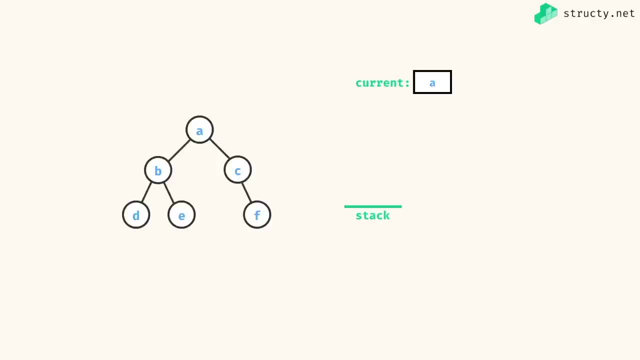 something leaves the stack, then I can consider it being visited right now. So I need to list out my values, because that's the whole point of this problem, right? So by now I've just visited the A node At this point I can look at that. nodes children now. So look at the. 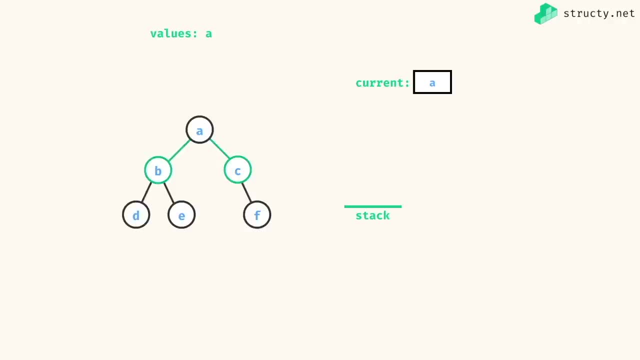 A node in the tree And I see that it has a B child on its left and a C child on its right And from there I push or add those two children to my stack. So I'm going to put B afterwards And notice if I push my right child first, followed by my left child. 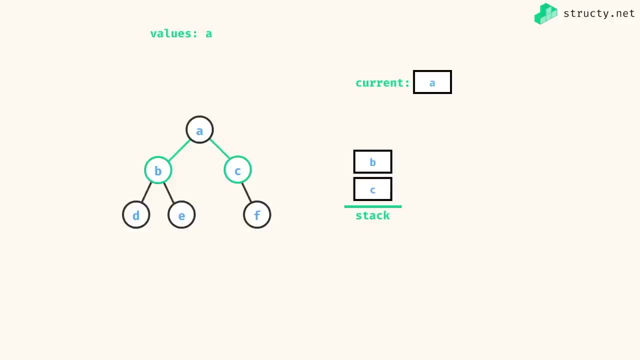 that makes it such that my left child to the top of my stack, which means that I would hit them next. And that actually ends on my first iteration of this depth, first reversal. And now I asked that same question: is my stack empty? It's not, So I remove the top. 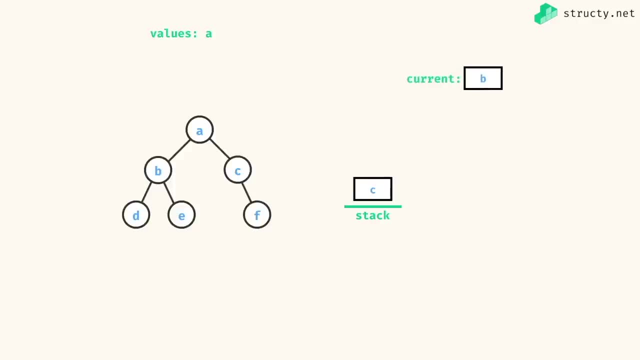 of my stack. I'll call it be my current, which means I could print it out or insert it into my values list. Nice, From there I can consider B's children. B has two children, So I add them both. I push e, followed by. 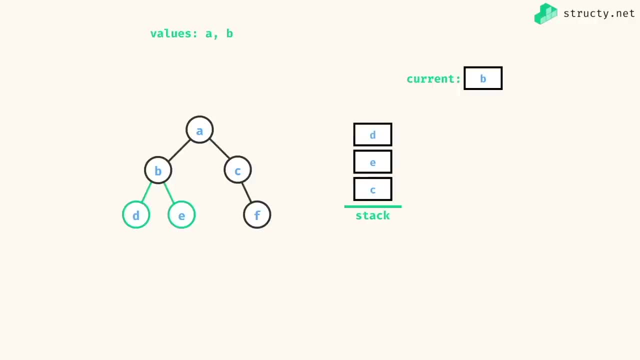 pushing D. That ends that iteration. Now something interesting happens. My stack is still not empty, So I know I removed the top, So I call D my current. I add D to my list of values, But if I look at these children, it actually has no children right, And so there's nothing. 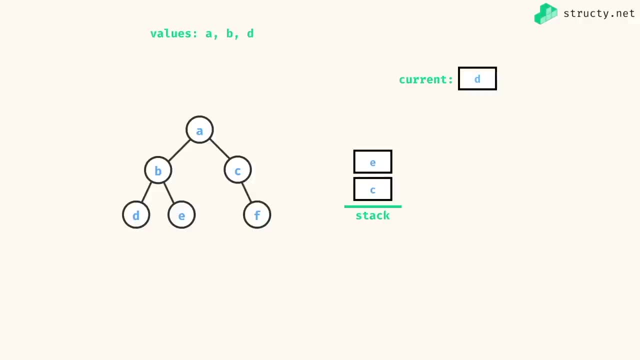 to add to the stack from here And so technically I finished this iteration And now I still have stuff on myself stack. So now I pop E off the top of my stack. Same thing as before, right, I add E to my. 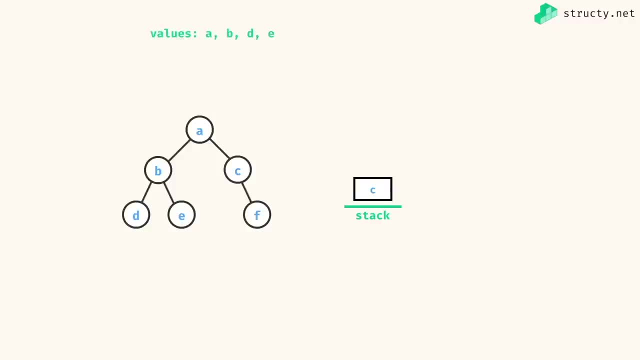 values. he has no children. So I'm done with that iteration. Finally I have C, I move C from the stack and I print it out in my values And then at this point I see that the C node only has one child. So I'm just going to push the children. that exists. So 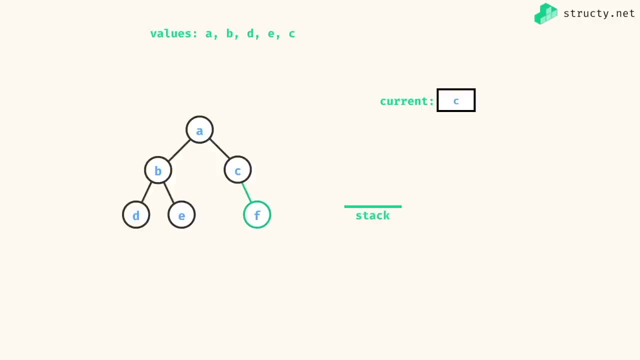 I would push the F node onto my stack, And that's a really important thing to remember when it comes to implementing your depth first traversal, you're going to have to check if your children exist before you add them to your stack. And now, on the final, final iteration, 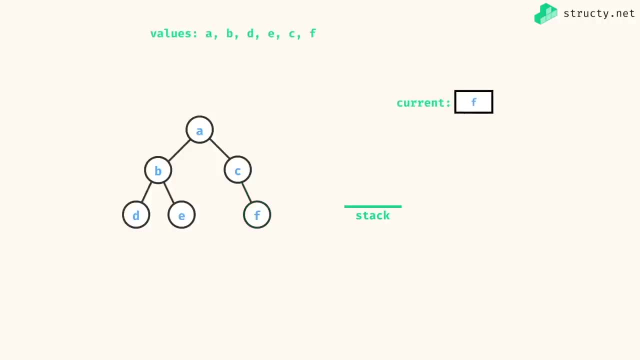 we have the F node, we remove it from the stack, we add it to our list of values. f has no children, And so I finished this iteration And now my stack is empty, And I would just exit right once the stack is empty. I know that I've must have traveled through the entire. 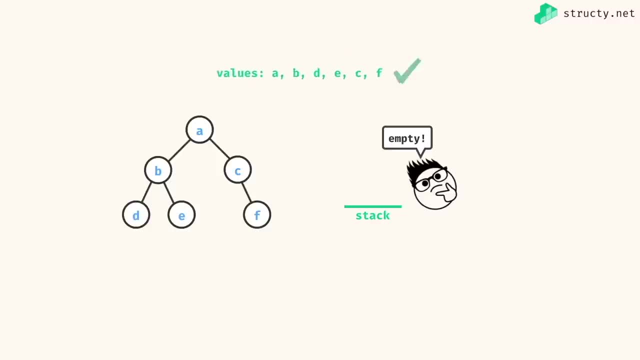 binary tree. So there we have it, And we do get the correct output over here. So just by using a stack and just obeying the rules of the stack- that is, we push to the top and remove from the top- we will get the correct order. Important thing to. 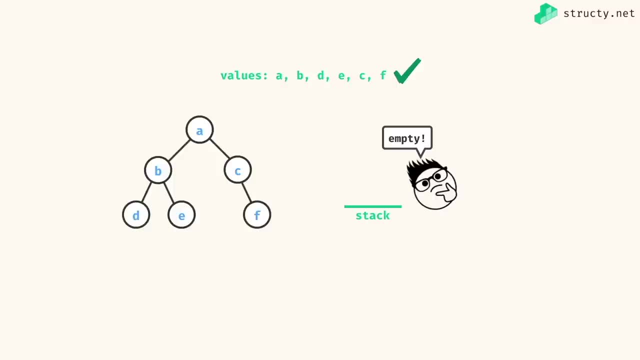 remember is you should add your values into your like values list whenever something leaves the stack. That being said, what can we say about the time and space complexity of this algorithm? Well, it's actually a pretty straightforward. Let's say we define n as 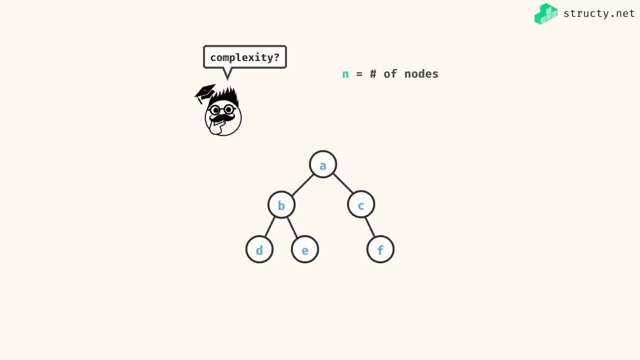 the number of nodes in this binary tree. then we can say that the time complexity of this is O of n. And why do I say that? Well, we're just going to add every node eventually to our stack And that node is also going to leave the stack, exactly. 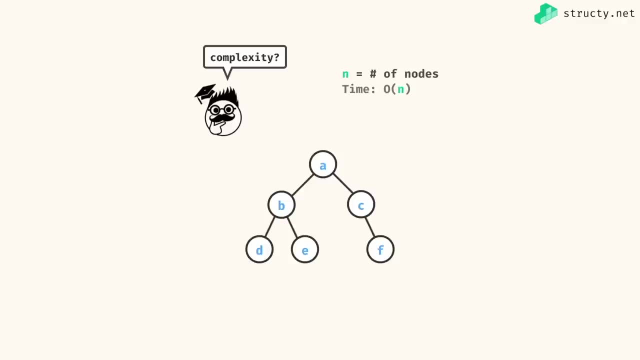 once. So it's not like we're double visiting any of the nodes. So I'm guaranteed to just run in O of n steps. In a similar way, we can see that the space complexity is O of n. the only thing we stored was really the stack, which is a linear data structure, And 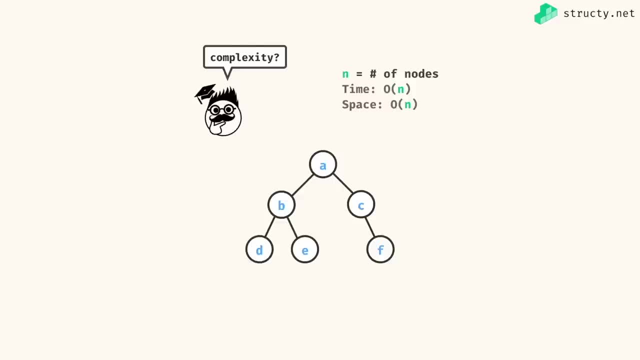 we know that we're not going to put ever more than n things on the stack. So overall, we have a linear time and space solution for this depth first traversal problem. All right, I think we have a good understanding about the approach for a depth first traversal. 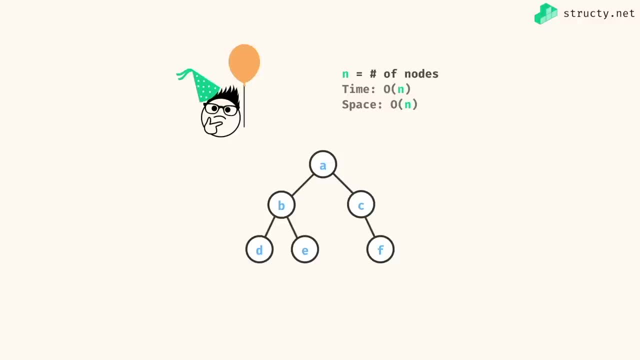 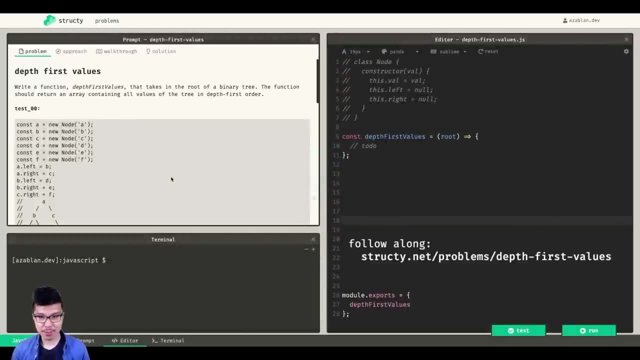 Now let's go ahead to the walkthrough video, And we'll implement this one in a few ways together. Hey programmers, Alvin here, right, and I want to go over a JavaScript solution for this depth first values problem, And so we're going to do here is really just implement. 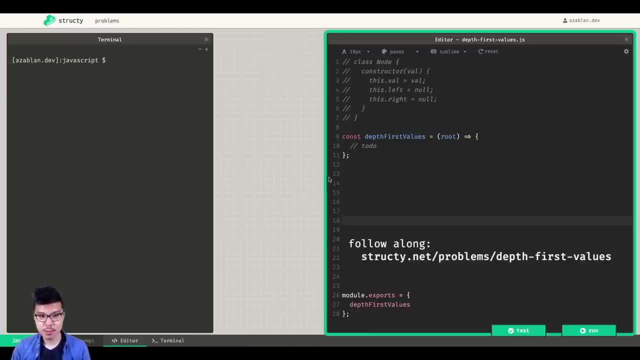 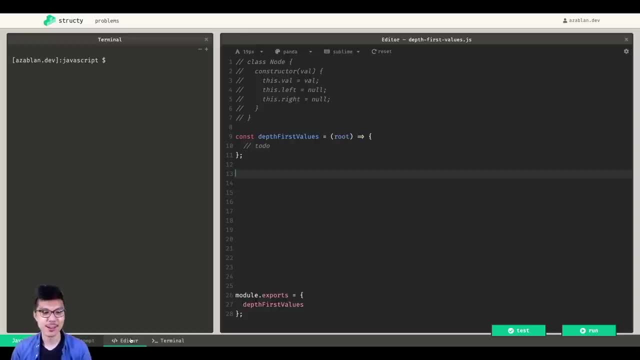 that same strategy that we traced through in the approach video, pretty much to the T, And we'll start with the iterative version, And that means, of course, we will solve this a one in two different ways. right, we're going to solve it. 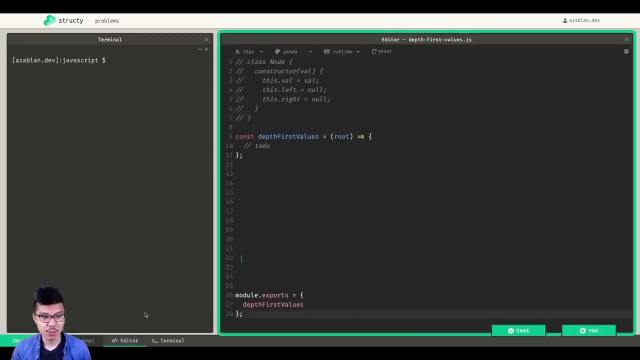 iteratively first and then afterwards, we'll go ahead and solve it recursively. Alright, so let's jump right in over here. Like we said in the approach video, we know that the iterative version really relies on us creating a stack And for most of your programming, 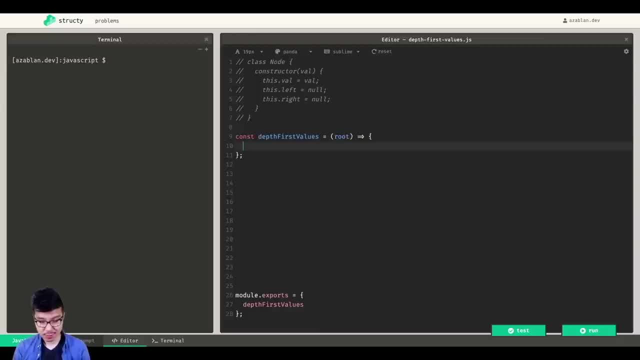 languages. you can just go ahead and use your like array data structure for that, So I'm going to use just a plain old JavaScript array. I'll go ahead and name this one stack And we can just use an array to represent a stack, as long as we stick to two particular methods. 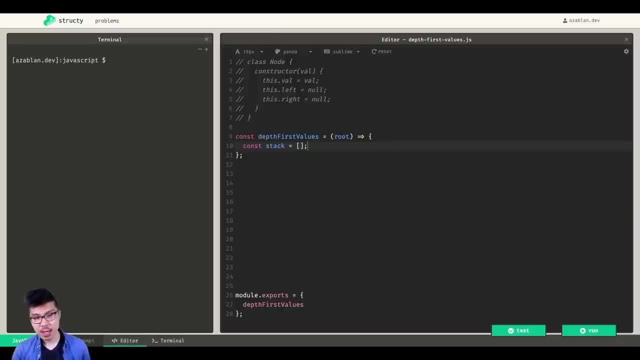 right, I'm going to use array push, which adds to the end of an array, and also array pop, which removes from the end of the array as well. So I'm going to consider the end of my array to represent the top of my stack. 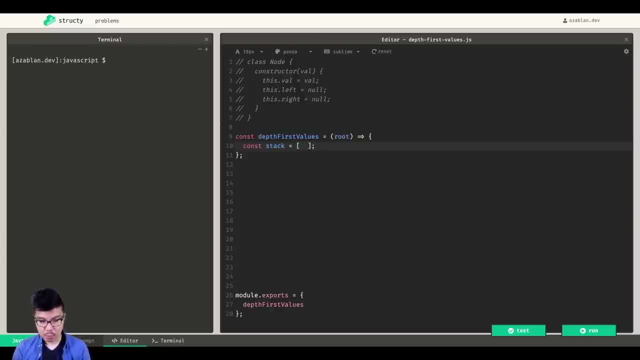 Cool, we'll go ahead and do is initialize the stack with the root node on top of it. Nice, Then I can have my main loop for the algorithm. So we know that we need to keep running the algorithm while there's stuff on our stack, So I can just check while stack. 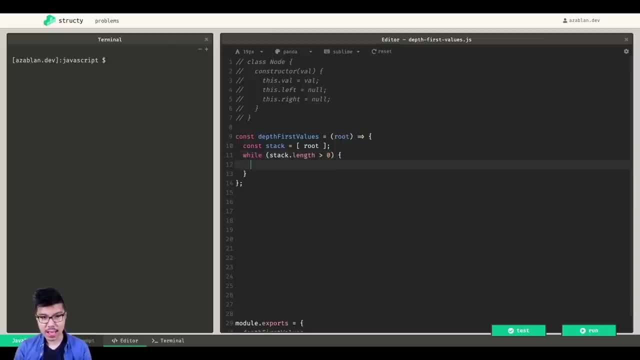 dot length is greater than zero. So while I have at least one element on my stack, I'm going to have my stack. there is some work to be done here And that will step through a single iteration of this algorithm. we know that we start iteration by just removing the 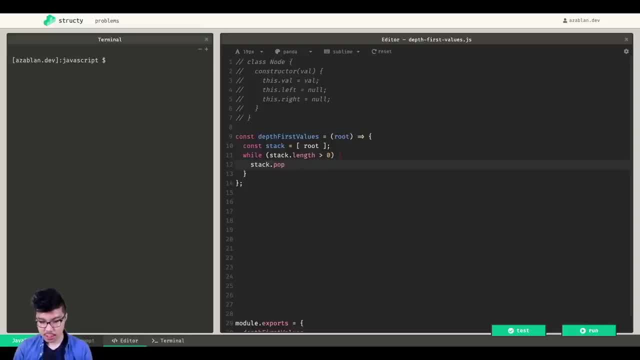 top of our stack, In other words, stack dot pop in JavaScript. that will also return us the element that we just removed. So I'll call that my current, current, And that is going to be an instance of nodes. it's going to be one of these objects, Cool. So now that 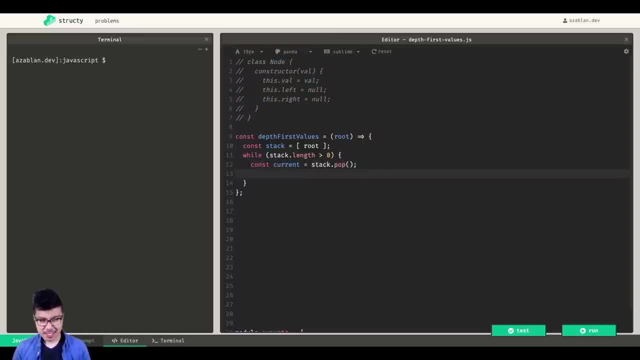 I remove this element from the top of my stack. let's say, for now I just- I don't know- print it out. maybe we'll kind of debug this one as we go. So, console dot log, current dot Val, because I know that every instance of 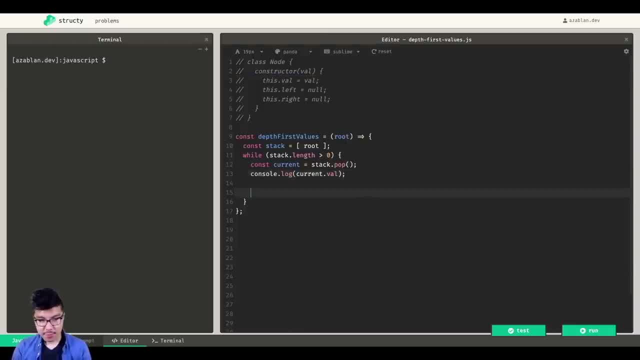 node has a dot Val prop on the inside And then from there- I need to add this- nodes children. So you might go ahead and guess that to do that we can just do stack dot push. I'm going to push the left child. what's going on here? So node or current dot left. 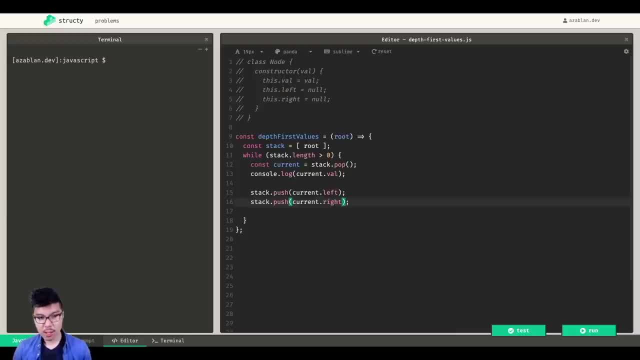 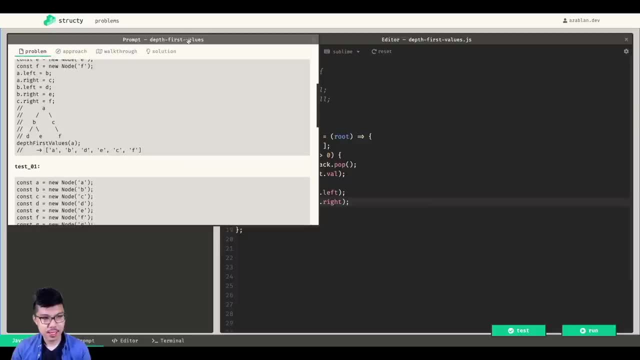 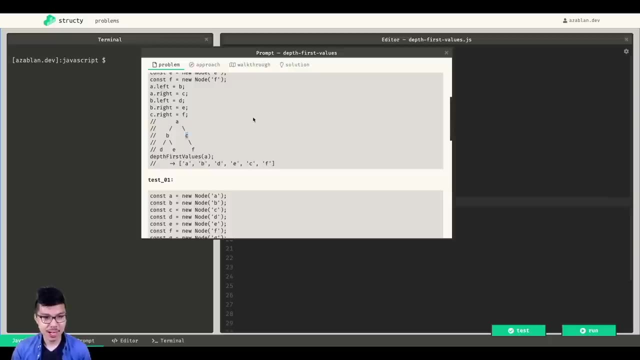 followed by the right child. But we also need to make sure that these children exist right. If you look at the prompt, there could be instances, for example, like this C node over here. this C node only has a right child but has no left child right. So what I don't want to do is push C's left because 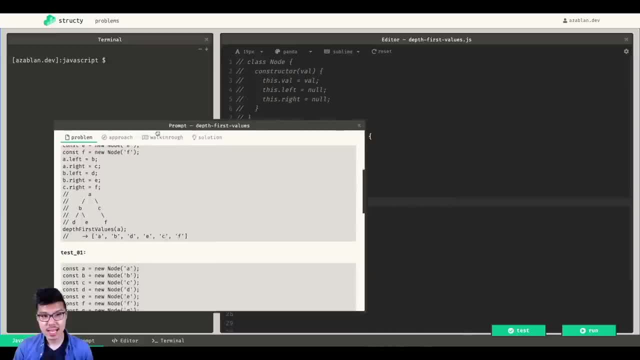 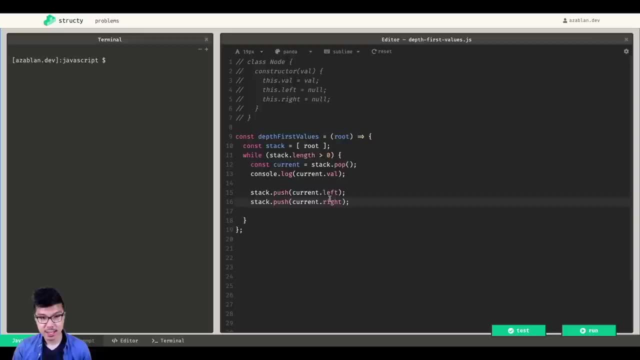 I'd be pushing null onto my stack, which would give me an error later on, Right. So I want to only push the children if they exist And I need to individually check. if the left exists, then push the children, And then I need to individually check. if the left exists, then 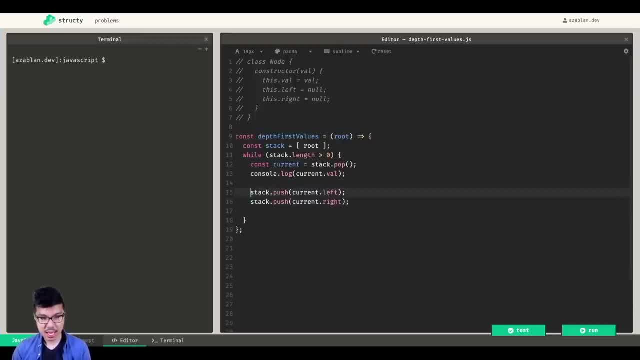 push it. And also, if the right exists, then push it. So we're just going to add some guard statements for both of these. So we'll go ahead and we'll insert. we'll say, all right, if the current has a left and right, it looks like current dot left And I'll adjust this for the 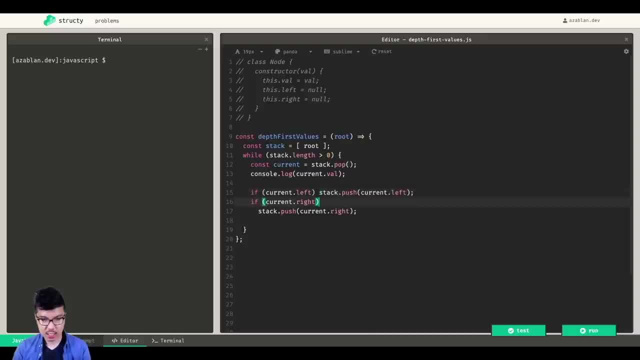 right hand side. Cool, maybe we can inline this if you prefer. Alright, so I'm going to only push the children if they exist, And that should actually be the heart of our depth first algorithm. So we're not putting our values inside of an array, like the problem asks, but we should at least be able. 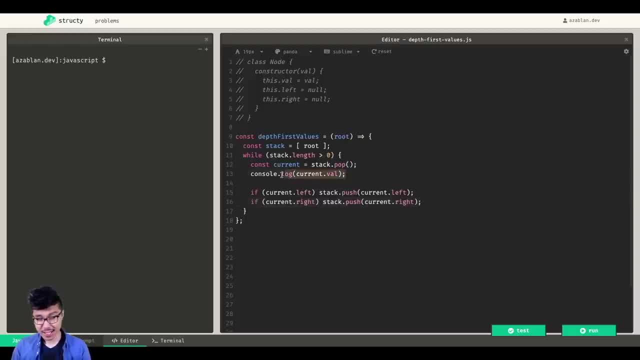 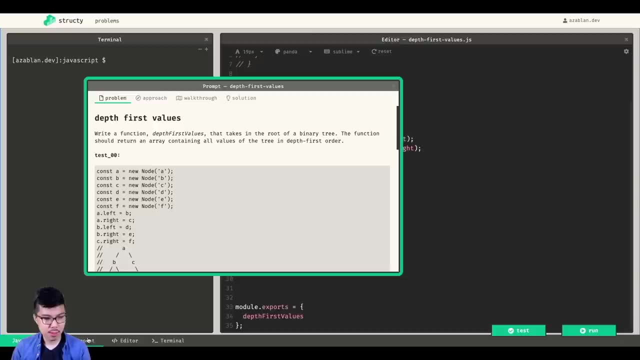 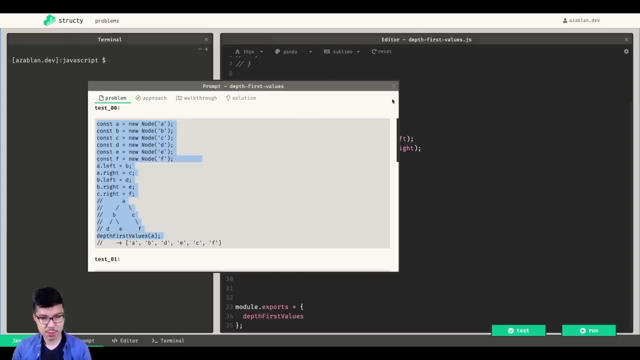 to see the correct order of printing here, because I'm going to print a node's value as soon as it is removed from my stack. So I'll go ahead and actually maybe bring in maybe one literal test case, So I could just steal this little stub over here And this will just print out the values. 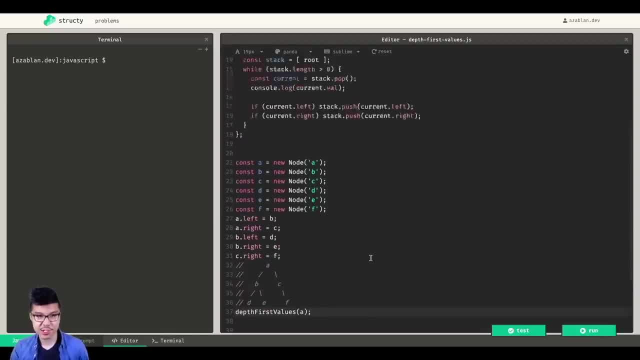 Right, so I'll test this. I can hit Run. If I hit, run is just going to execute this file, just like a a script. So it's not going to run any automatic test cases, just going to run my file as is So. 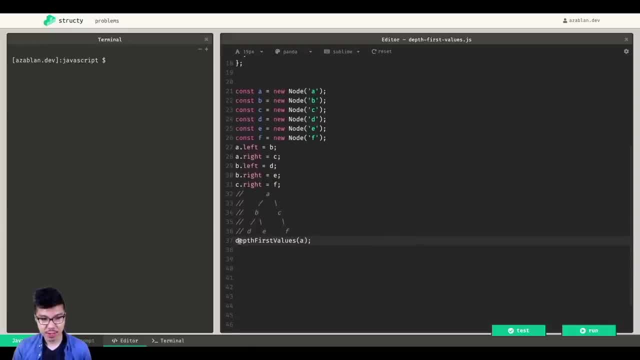 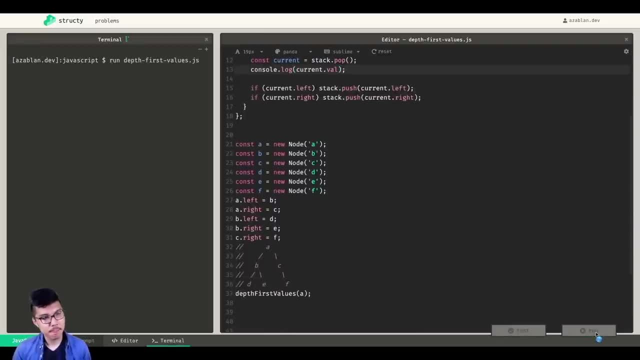 if you want to test it in this way, kind of in a manual way, you're gonna have to be sure to call your function. I do have a console dot log on the inside, So I'll just run this manually And when I do that should see some output here. Looks like node is not defined because I forgot to bring in. 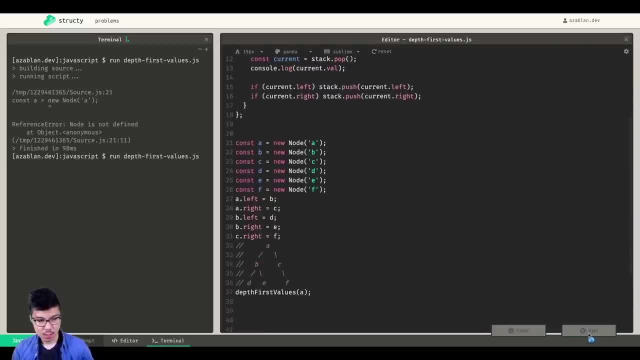 my class definition. So I'll do that. Give that a go, Alright. so, looking at our output, we didn't get our exact depth first traversal like we expected, right? I got ACF BED. if you take a look at what we really printed out, we technically did print out a depth first print. 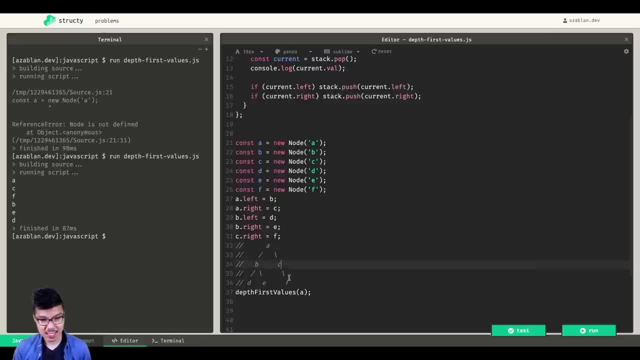 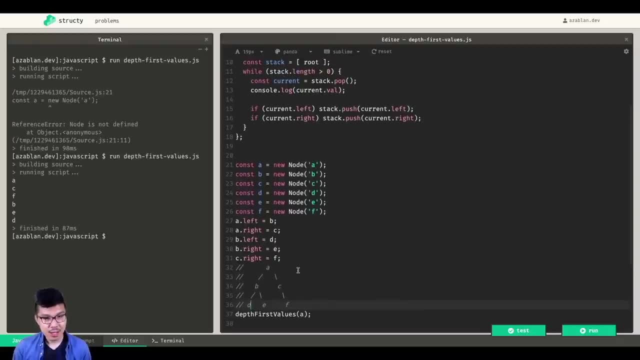 But we favored the right hand side, So we did ACF and then BED. So let's say we really wanted the left to right version of this And all you have to do is flip the order that you push the children right. It should be clear by looking at these two lines right, When I add my children. 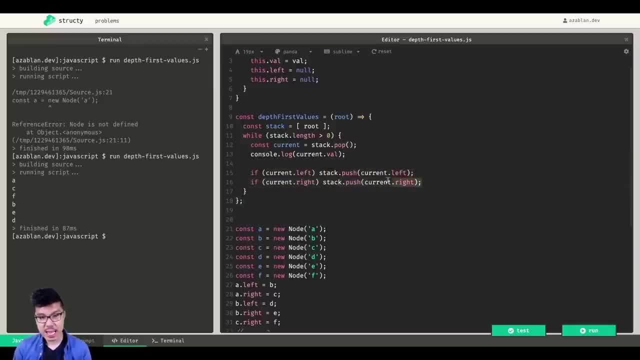 looks like I push the left child and then the right child. If you push the left child first and then you push the right child afterwards, that means that the right child is going to be on top for the next iteration. So if you do it like this, this will favor the right hand side and 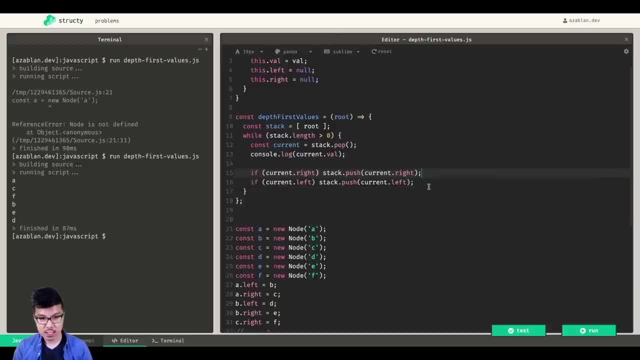 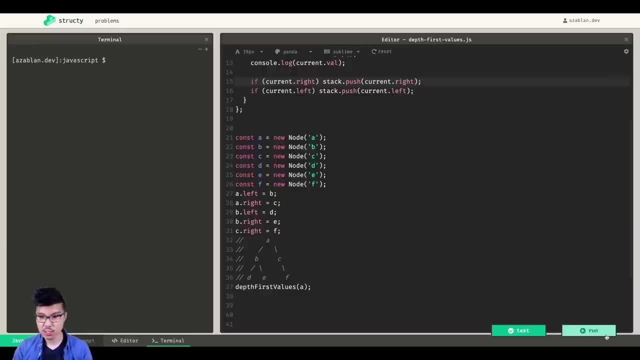 travel through it first. But if you did it like this now, you'd be actually iterating to the left branch first, toward the right. So with that small change, let's just see what our print is, And there I have a nice ABD ECF. However, in this problem, they want us to actually return. 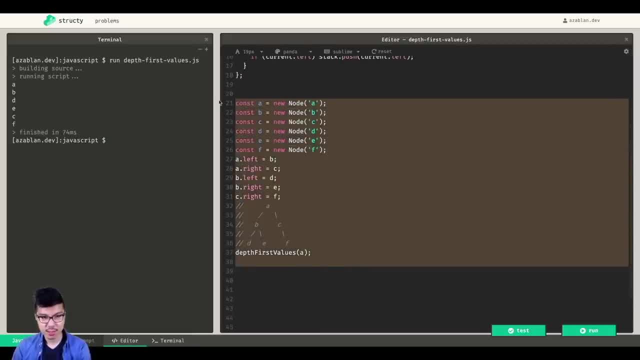 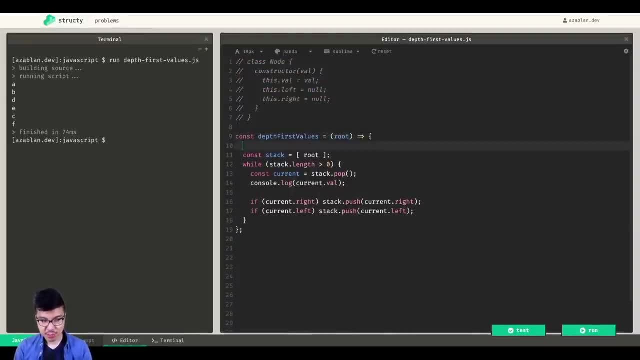 those values in an array. So I can kind of get rid of this little manual test over here. I don't need this class definition anymore Now. instead I'll just gather up all of my values in some results array. So I'll say: I don't know, maybe result over here starts as an empty array. 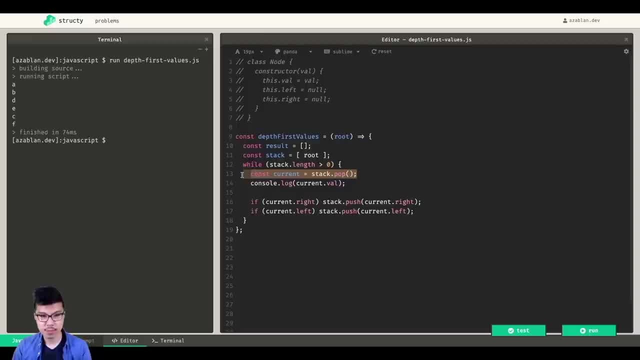 And then, as I pop elements from the top of my stack, instead of logging them, I'll go ahead and do result dot push, and then it open up and it'll say: Well, she, she bed doesn't have this class herself. you know that's gonna be fine, but that's possibly not. Another thing is it also doesn't. 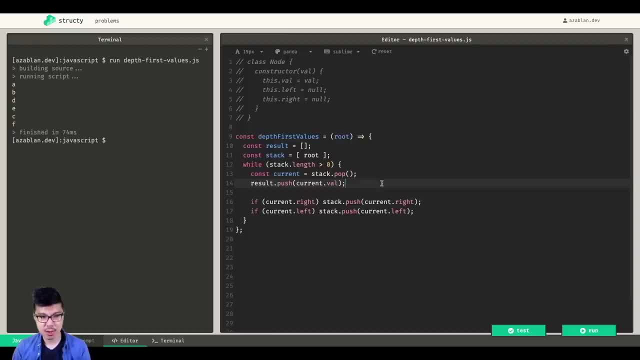 tell her around a lot of our firsts necessary info is our next set pairs Right and that just doesn't fit right. So push, and I'll push that value into the result array Once I'm done with this while loop. 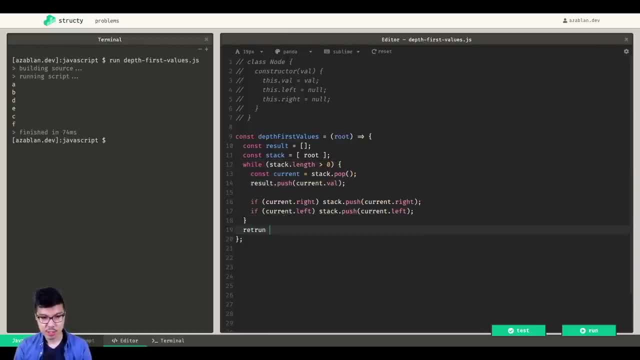 that means my entire tree has been explored, in which case I can return. make sure you spell it right. return my results. Cool, So this should be a nice solution. It's actually run the test cases on this. Give that a go, So it looks like we're doing pretty good. 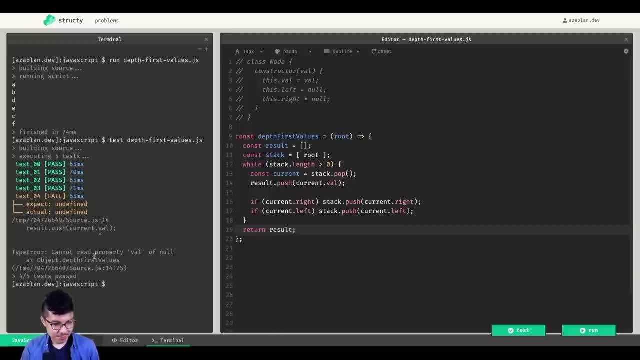 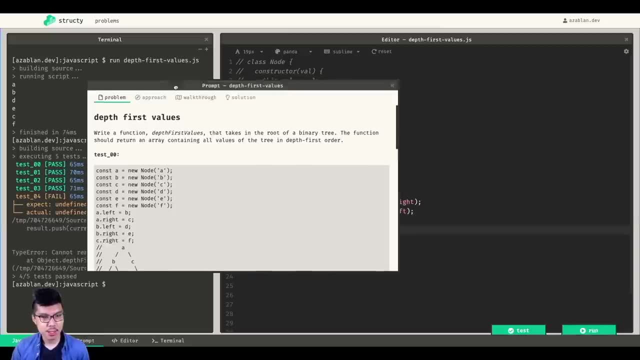 But for this very last example looks like we're getting can't read property Val of null And that's running test case 04.. So if you actually go into the prompt, those test cases are actually laid out explicitly over here. So I want to go to 04.. It looks like a 04. 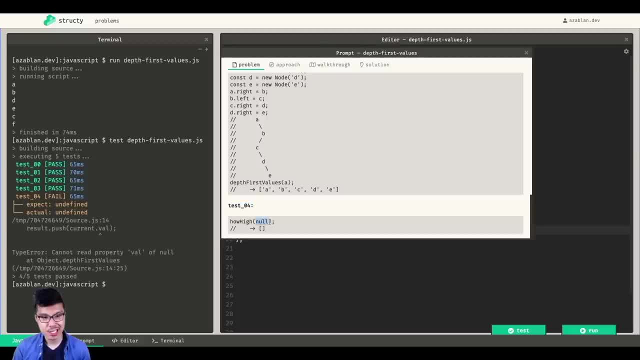 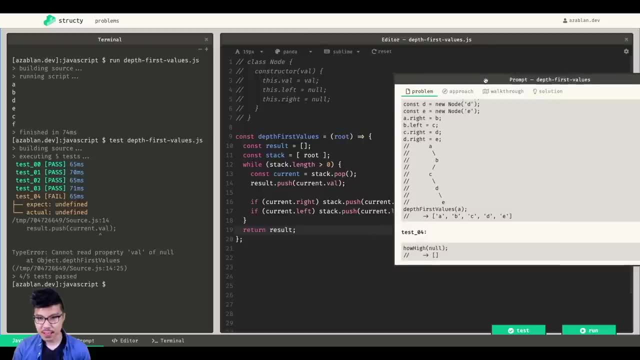 test case. they go ahead and they pass my function null, right kind of representing like an empty tree or an empty node And we can kind of trace it. what happens here? for our code, Let's say that root was null. That means when we initialize our stack, our stack. 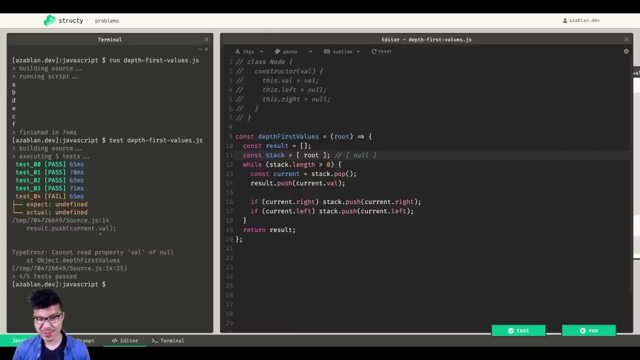 literally contains like a null value. So it's not even an instance of no, it's just null. So that means, when I enter this while I'm going to check, you know, do I have anything in my stack? and I do because my 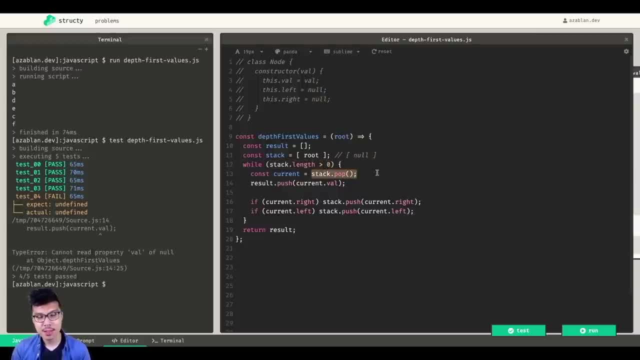 stack length is one, And then when I pop, the top element of my stack current is going to be null. And then on this line 14, it says null dot Val. And that's actually where our code explodes, right on line 14.. Right, You can't reference property Val of null. And 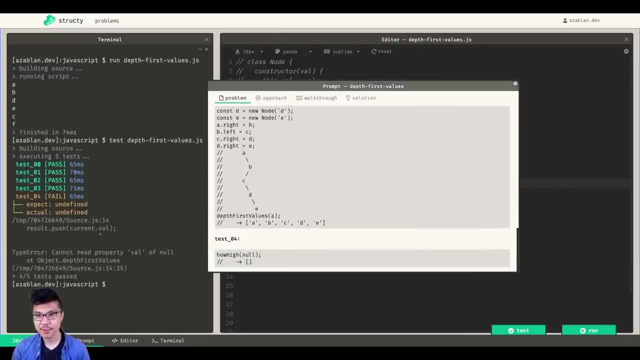 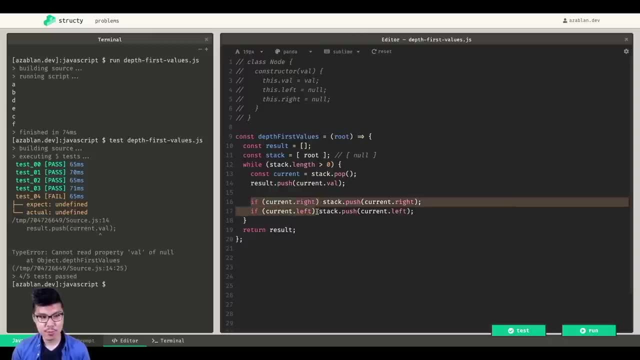 so to handle this scenario, we want to make sure that we actually never allow anything null to enter the stack. It's kind of why we had this guard over here, And that should also be true for even the top level root, in case they give us the empty tree, kind of seems. 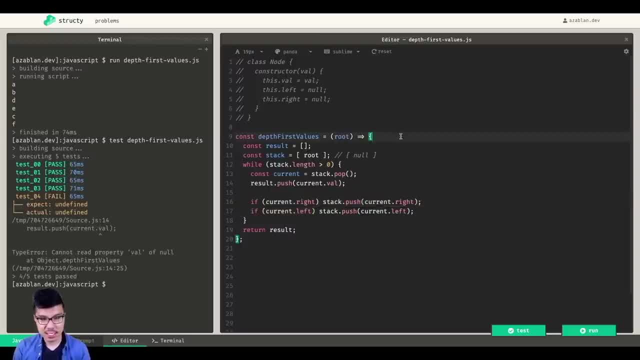 like a corny you know edge case, But this is a pretty common one. when you actually go into your interviews, right, What happens when you have an empty input? And so I'll just guard that explicitly, I'll go ahead and check. hey, if my root, so if my entire. 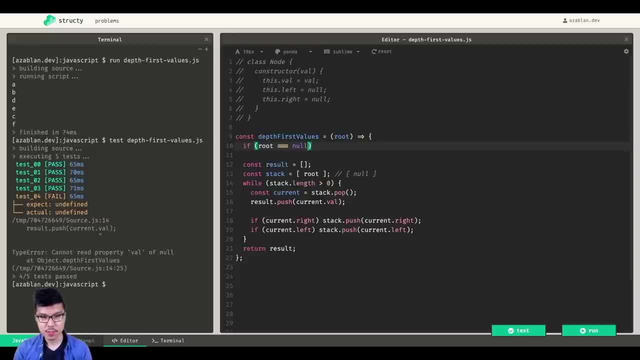 tree is empty. so if root equals null, then what I'll do is just return an empty array. Right, Because that means there are no values inside of it, And that actually is the expected answer. according to this, right should return an empty array. So let's give it a go now. 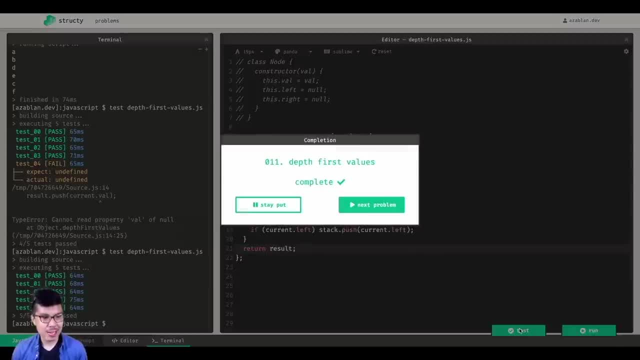 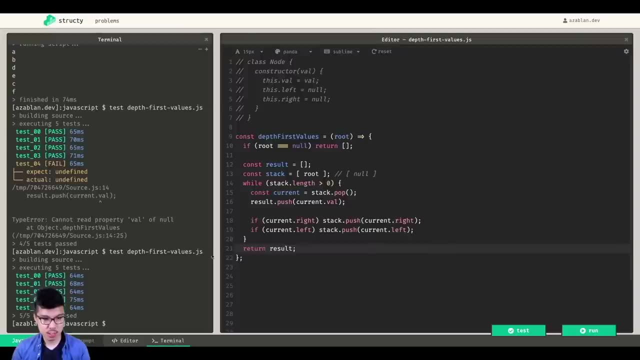 Should be pretty good. Nice, And there we have our nice iterative solution for this depth, first values problem. Alright, so here's what we'll do. That was one solution. Let me show you another way. Let's implement this, and that would be our recursive flavor. So 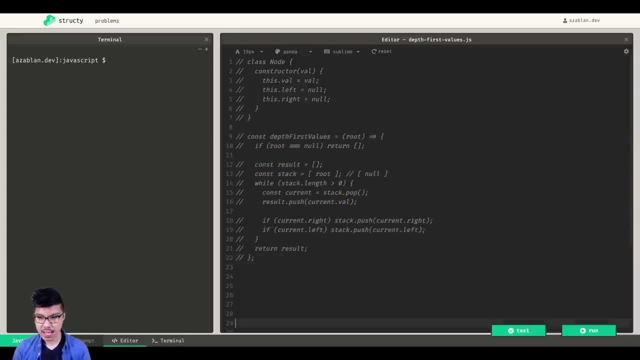 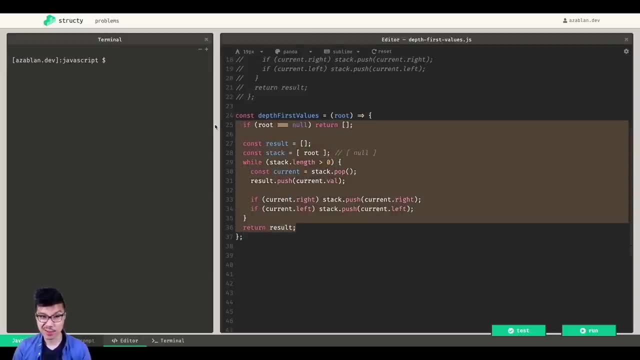 I'll just kind of redefine it down below, And I actually recommend practicing both versions because they're going to serve as, like, the basis for which you solve a lot of different tree problems. And so when I think about the recursive version now, like all of our recursive code, I must think about 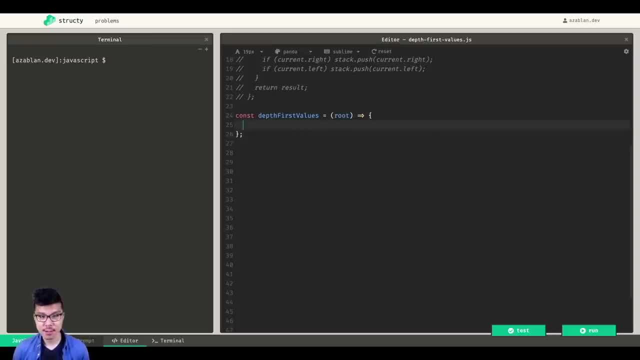 the simplest case of my input and that will act as my base case, right? So in the case of a binary tree, the simplest tree you can be given is going to be the empty tree or just a null root, right? So it's not even going to be about a node, that's single node. 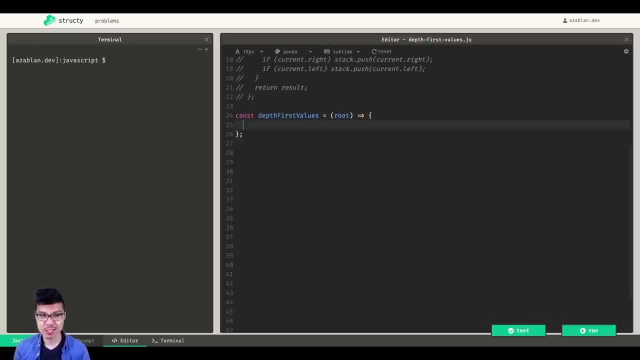 right inside of a binary tree. it's going to be about an empty tree or a tree with zero nodes. So I'm going to check. Hey, if my root is null, then I have an empty tree. And I think about this base case as if it's its own input, because 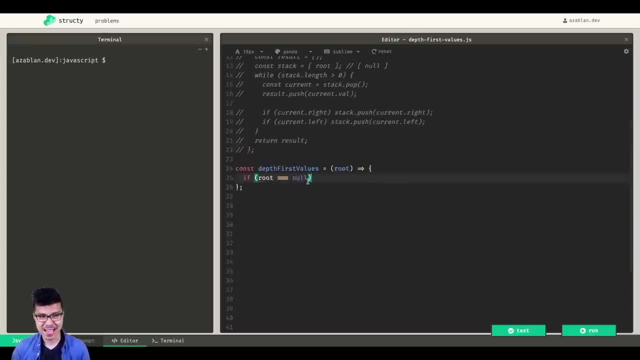 it really is right. And so if someone asked me to give them back an array of all the values in the empty tree, it's still the case that this must be an empty array, because there are no values, there's not even any nodes in the empty tree, And then from there I 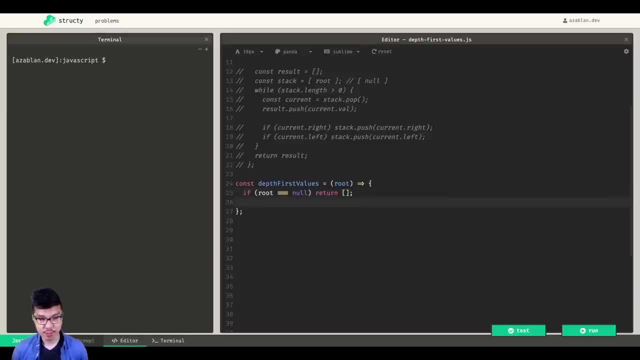 can generate my actual recursive call right, And I know when I call my stuff recursively, that means I have to reference the function name again, go ahead and invoke it, And I'm going to call upon a root dot left as well as root dot right. So this would this color here would give me back. 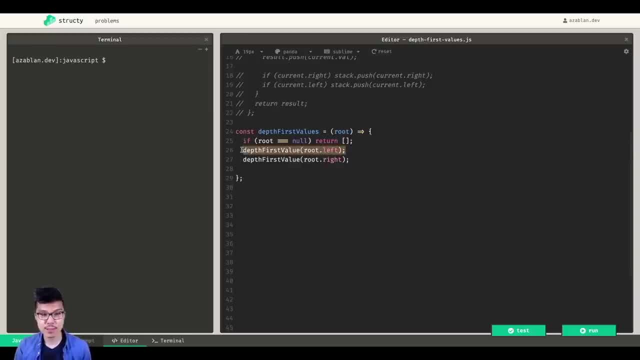 an array containing all of the values in the left subtree, And this would give me an array of all the values in the right subtree. And so let's say, I save these into their own variables respectively. you don't have to do this part, But I'm going to do this, So I'm going to. 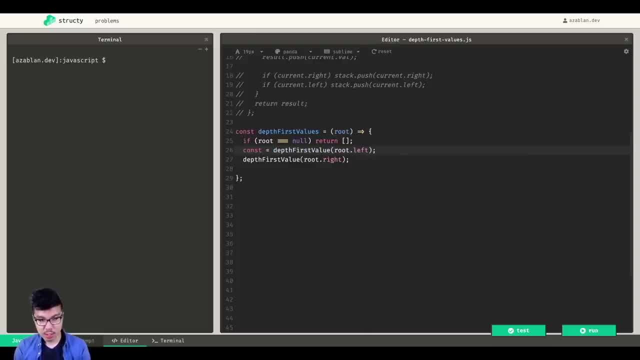 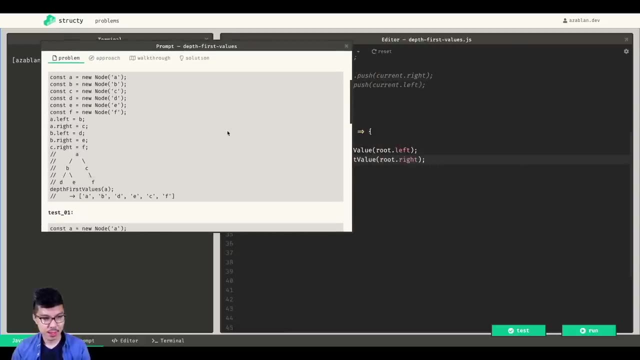 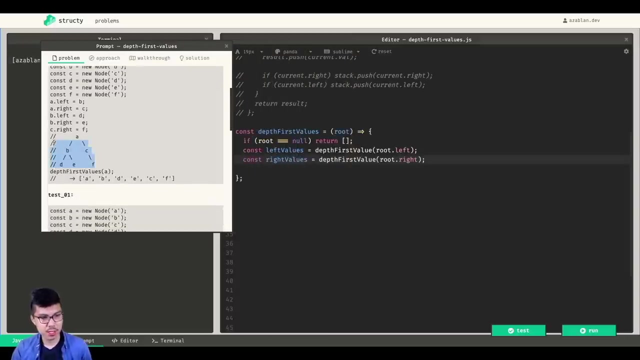 call this my left values And I'll call this one my right values, And here's how I'm able to kind of quickly create recursive code. It's all about taking what I call is a recursive leap of faith here. So let's say we're stepping through test 00.. So this is our tree visual. 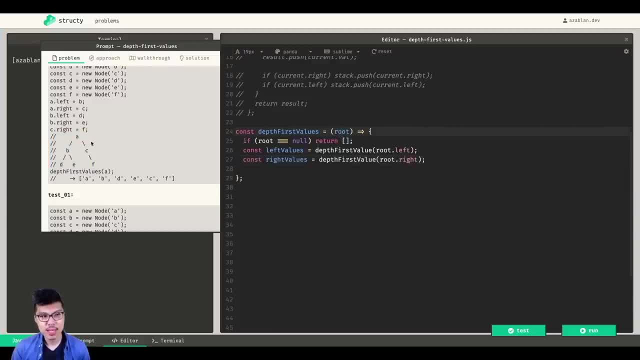 right. So we know that our route is going to be the a node. So when I actually make this top level call, this base case does not fire And so I make my recursive calls right. I know when I do depth first, value or values rather, we fix. 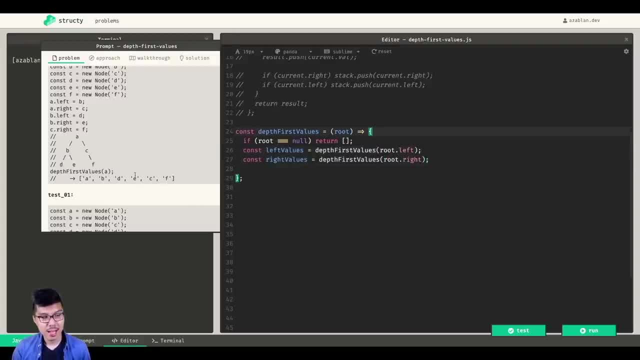 that depth first values of root dot left. that means I'm going to be passing in the B node right, And here's how I have to actually pretend my code behaves. I'm just going to get back the correct result from this call, right? So if I passed in the B node into this, 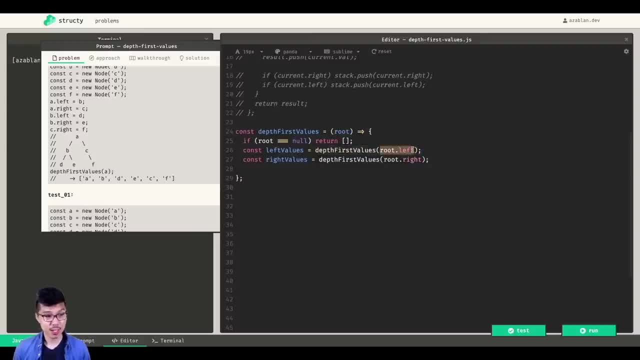 call. what I expect back, you know, is I'm going to get a call into that node, So I'm going to get a call into that node, So I'm going to pass in that node into this call is the full array representing the depth. first reversal of that sub tree, starting at B right. 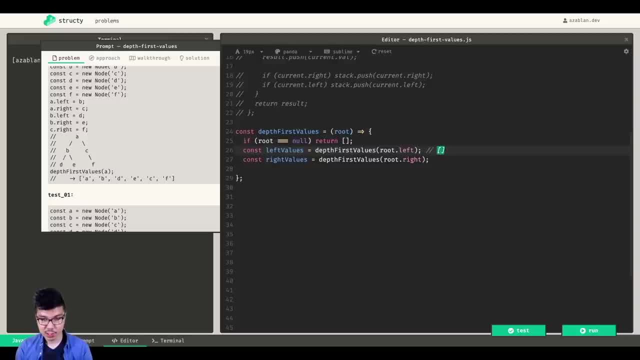 So if I got correct data over here, what it would look like is just B, D and E. That would actually be the full depth first reversal from this sub tree. right, And I'm kind of doing that just mentally- I know the expectation for this algorithm. it's going to be a similar. 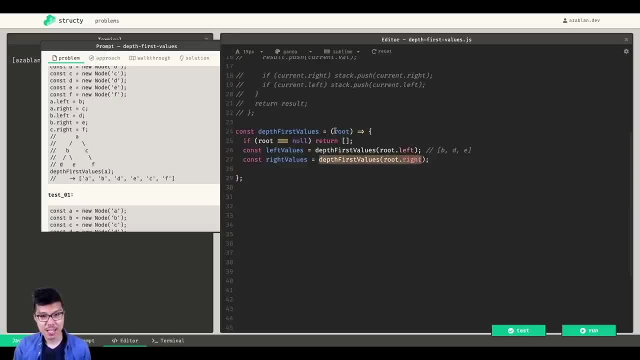 story for my right call- right If I'm at a, so a still my root- and I passed in my right child C to this call. what I expect back is just an array of CF, which would be the depth: first reversal of that left sub tree And now that I have, you know, my left sub. 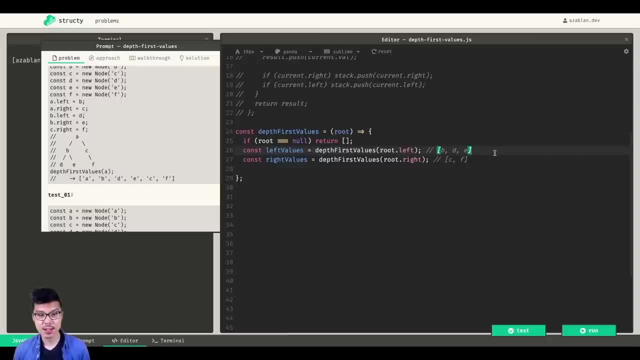 tree values and my right sub tree values. I have to think about how to combine it all together, right? How do I work myself into that output? by combining both of the results from my children, right? what I need to do is really just take myself, put it in the array. 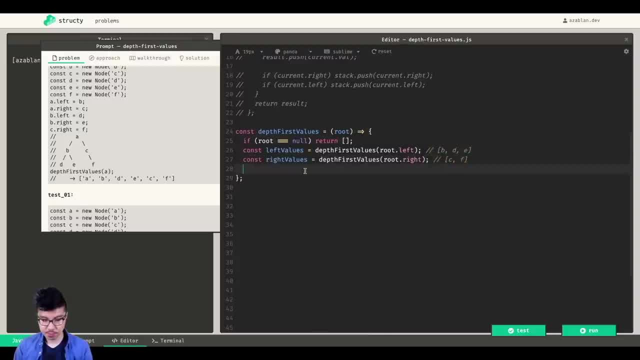 followed by my left children, followed by my right children. So I can use some nice JavaScript syntax for that. when I return a new array, I'm going to throw myself in there. So I'm going to throw in a root dot Val. that's myself. 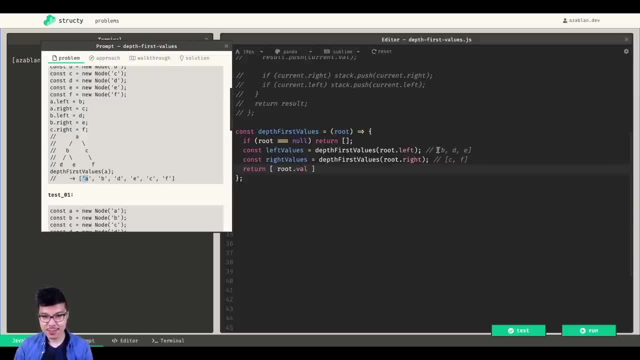 So that'd be like the A node. then I just take all the values in my left result, put them in here. I'm just gonna use the spread operator to unpack that array And I'll do the same thing for the right values of CF, right? so dot dot dot, spread out right values. 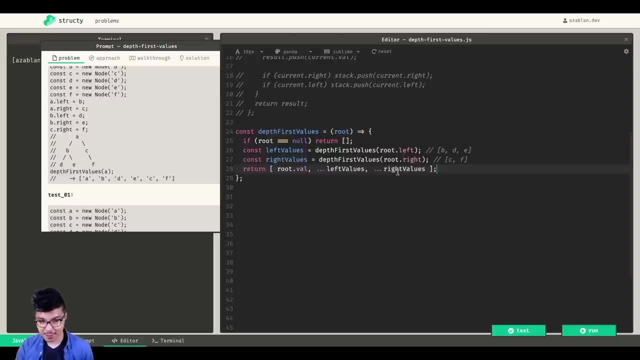 just so, I return a single array And this pattern itself does match This output. right, kind of taking the leap of faith and assuming correctness from these recursive calls over here. right, I have a and I plug in, substitute B, D, E and then 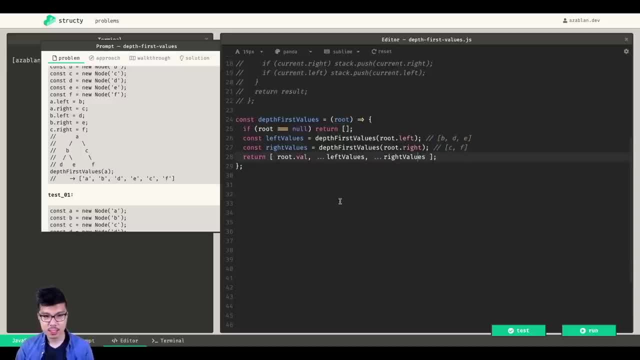 for the right. I have CF. maybe before we run this I'm not going to, you know, assume too much JavaScript knowledge, So maybe you're kind of new to this spread operator. So in general, super quick aside over here. let's say I had an array of some stuff So I'll. 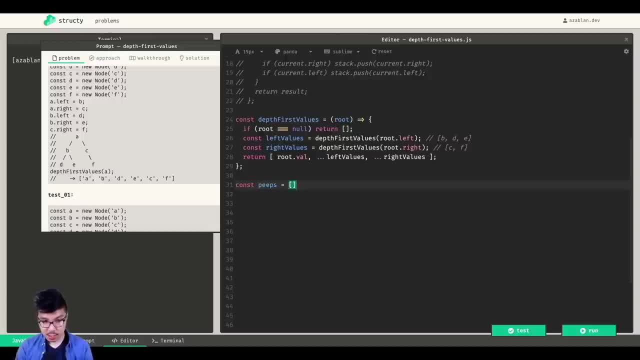 say, peeps, throw in some people over here. So we'll throw in Felipe, we'll throw in Jason, throw in Raj, throw in Abby, And what I can do is, whenever I have an array, I can just use a spread operator to kind of unpack. 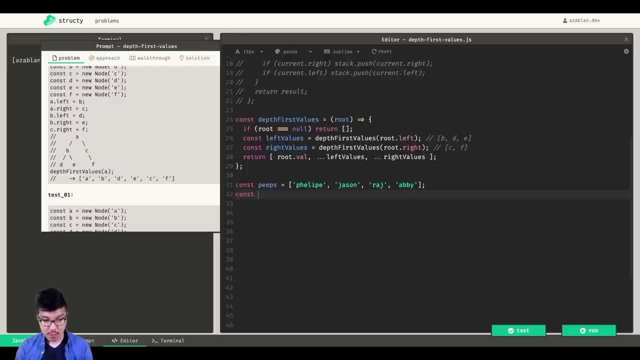 that array. So, for example, I can say const, we'll say new peeps And I'll create a new literal array. So whenever I say square brackets, it gives me a new array literal. And what I'll do is I don't know- put an element at the front, we'll call it Alvin, And then I'll. start writing around And then I'll express the element And then I'll get the new array in my list of favorite elements And then I'll say complet and I'm done, And I'm done. So I'm going to keep it simple. And then I'll dab my keyboard and then I'll do a new element. 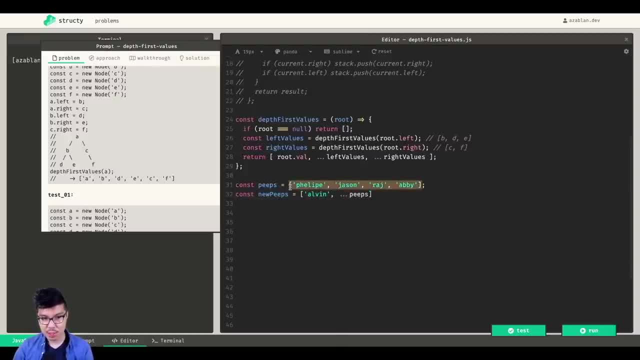 And then I'll spread out the elements of peeps, Right. So just imagine I took all the elements here and just remove the brackets. that way I don't add any initial nesting And then at the end- I don't know- I can add someone else like brian will console dot log what. 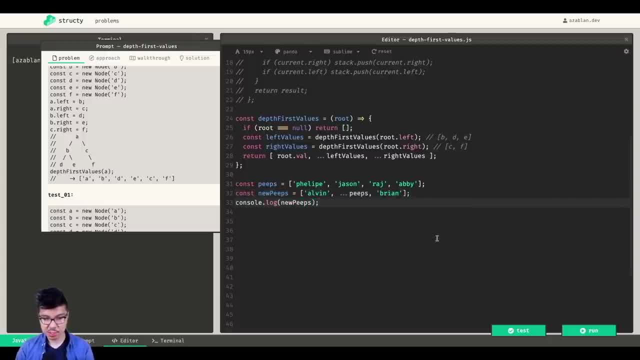 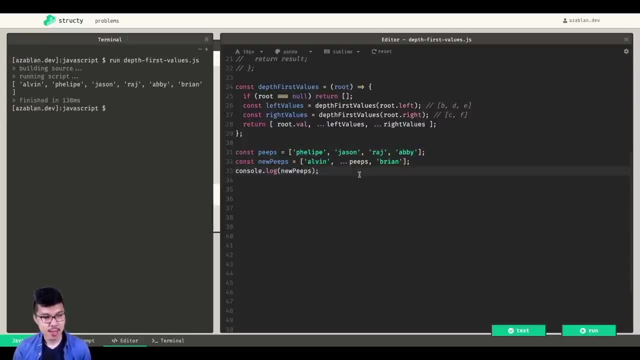 new peeps looks like. so I'm not going to run the test cases, we're just gonna run this file as a script, just so we can review this spread syntax. So if I give that a go, we kind of make this bigger. 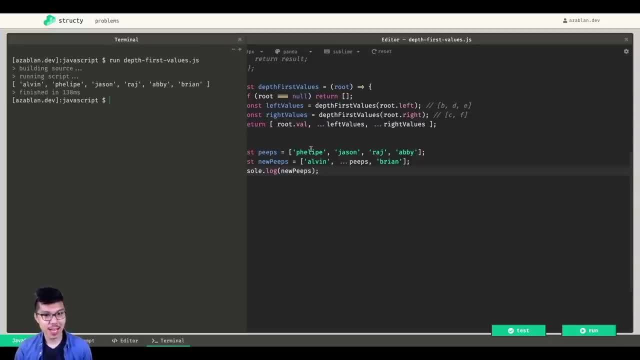 notice that I have correctly spread things out: right, have Alvin at the front And I have all of the things from peeps in the middle right, followed by Brian at the end. So you can do this. you can also use like the concat method on arrays. you're probably going to see me use this spread. 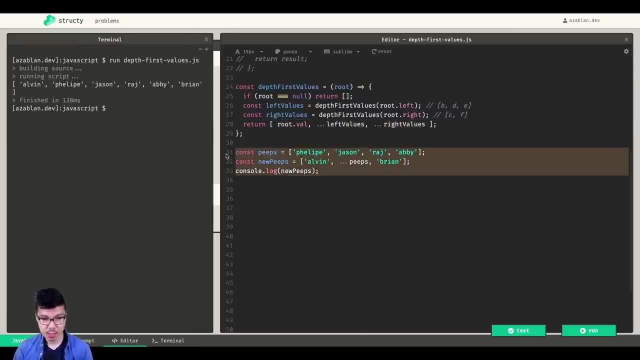 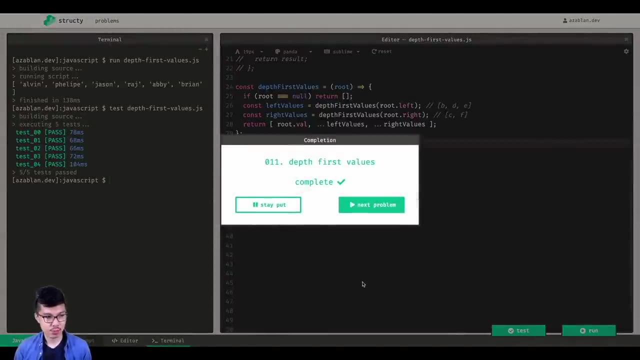 syntax, a lock, some kind of a fan right. With that in mind, let's go ahead and actually test this code. So we'll run all the test cases. Nice, And this is another working solution for our depth first values, And it should be pretty natural that we can solve this problem also recursively. 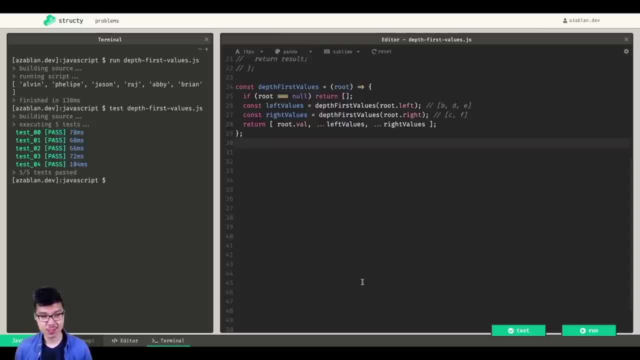 So I know that the iterative solution for this depth first traversal requires a stack data structure And I know whenever I write recursive code under the hood, your programming language is actually going to track all those recursive calls using the call stack. right, that call stack. 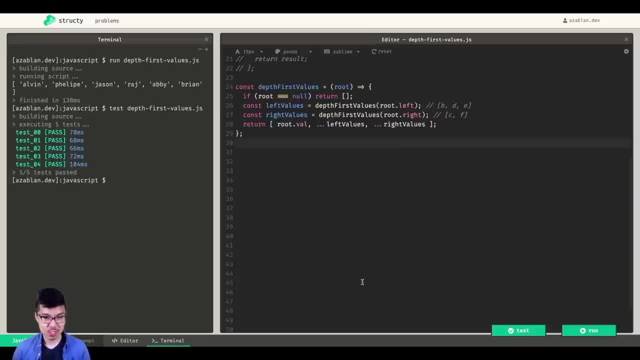 behavior gives you the Same type of ordering, which is really convenient. Cool Alright. so before I send you off on the next problem, I want you to actually practice both solutions for this depth first values code. it's going to be very necessary to actually master some later concepts that are coming. 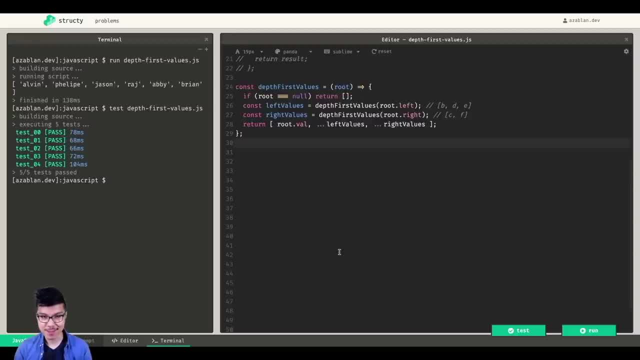 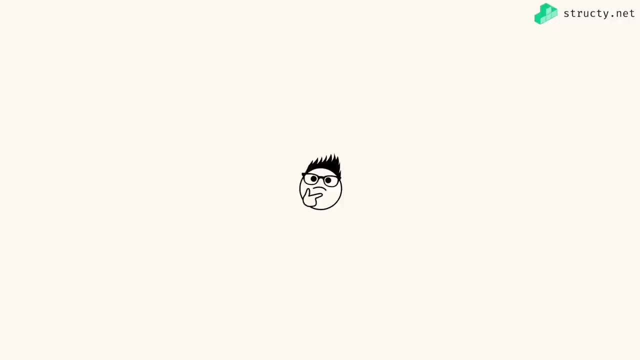 right up, So do spend some time on this. practice makes perfect right, And I'll catch you in the next one. Hey programmers, Alvin here, Right now I want to go over this breadth. first values problem. So it's really just. 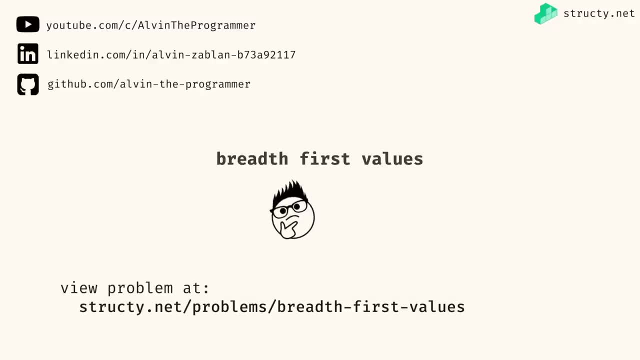 going to be a little variation off of the depth first one we just did, of course, But it's really important that, moving forward for all of our tree algorithms and other data structures, that we have both versions down pat. So in this problem we're going to take in a binary tree once again. very 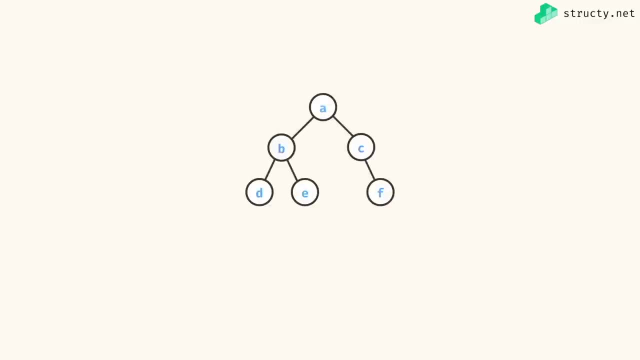 classic binary tree structure. But this time I want to return an array or a list of all the values according to a breadth first traversal order. So a breadth first traversal starts with the root node of A, so that's nothing new- And then from there I could go to B. So right now, 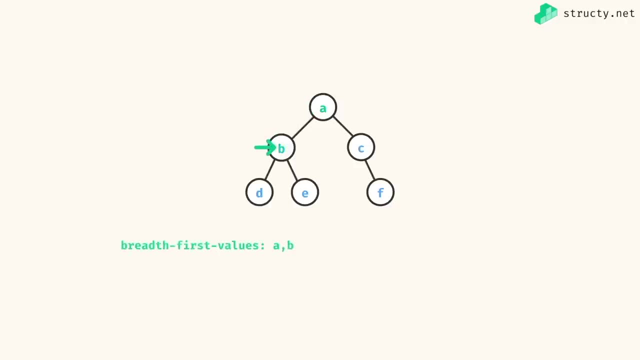 I have my A node And then from there I could go to B. So right now I have my A node and then I have my B node. And here is where we diverge from a previous problem In a breadth. first traversal. 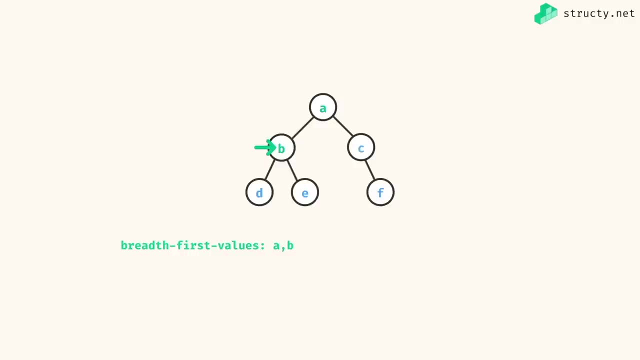 breadth just refers to like the width of something I travel across before I go deeper. So in our breadth, first traversal, I'm going to move to C and not D for now. So I add my C node, C value, to my list And then from here, once I finished this entire level and there's nowhere to go, 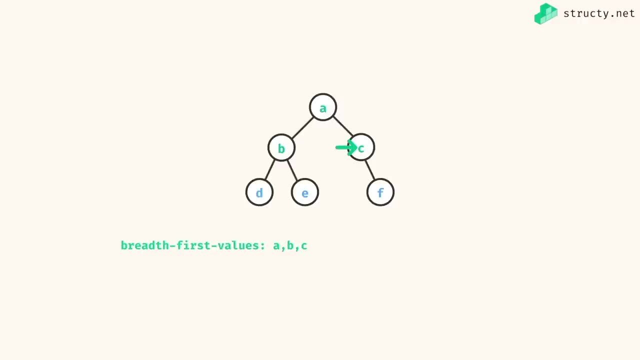 across the tree anymore. Now I can go downward to the next level. So now I have D and then E and then F. So the really important distinction here is the breadth first traversal starts with ABC, whereas the depth first traversal would have started a, B, D, that's a really. 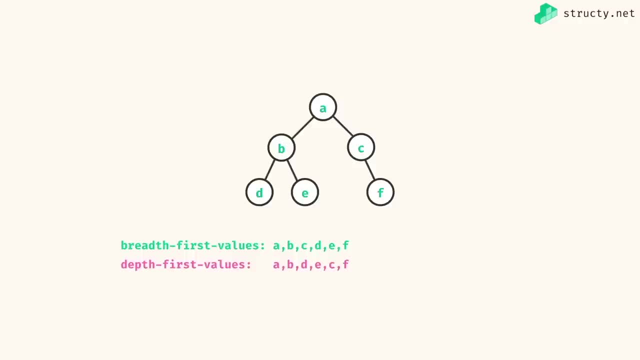 really important distinction. And so how can we go about implementing the breadth first version of this? Well, recall that the depth first used a stack data structure. Well, it is the case that the breadth first is now going to use the queue data structure- really just the. 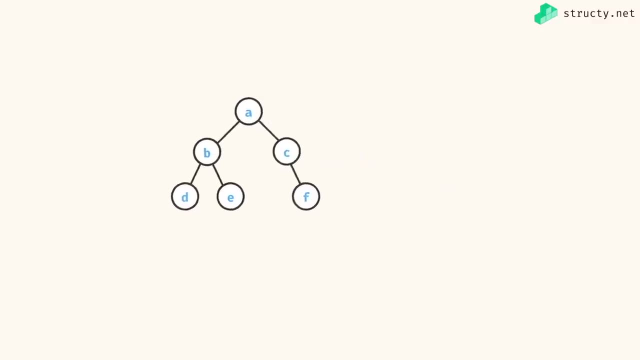 partnering version of that structure, And so let's kind of step through that in a more programmatic way. So I'm going to use and track my queue And just recall that a queue has, you know, a sense of direction to it. have the back of my queue and the front of my queue. 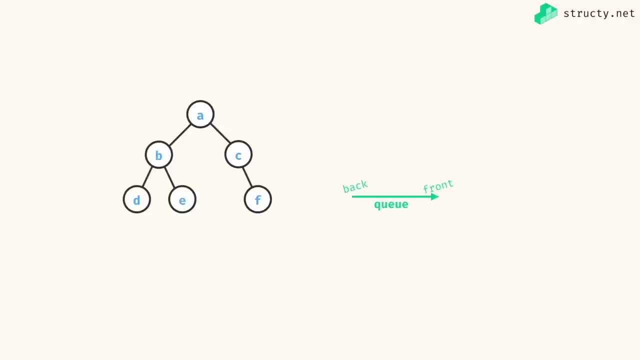 things enter the back of the queue and they leave the front of the queue Right, And so no one gets to skip the line either. So this gives me a nice, fair ordering. think of a queue is just like waiting in line at checkout at a grocery store or something. So how do I begin my algorithm? Well, 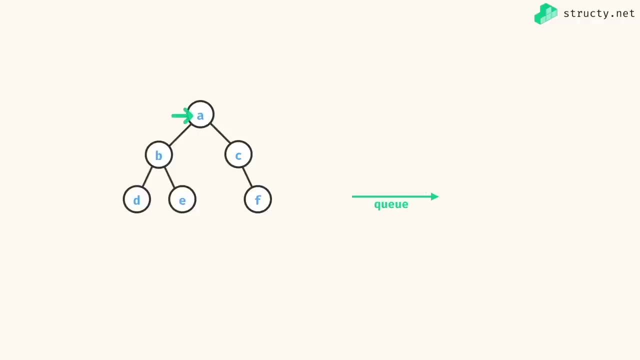 by initializing my queue with the root node. So I'm just going to start with a on my queue, Then from here now I can begin my main algorithm. So my main algorithm should check on every iteration. is my queue empty Right now? it's not, because I have at least one element, And so I. 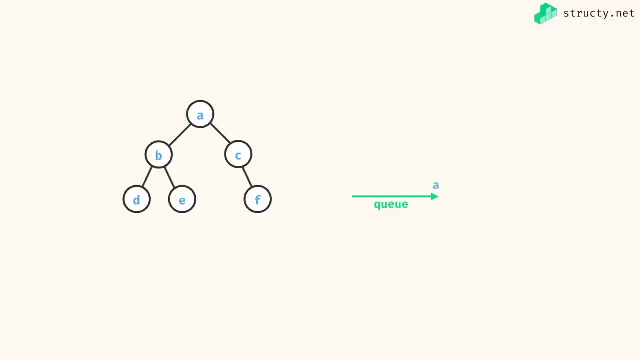 remove the front element of my queue. So we know that a would be removed and we label it as our current node being explored. When something leaves the queue and is marked as our current, we'll say it's visited. So I would add a to the running list of my values And then from here I need to look. 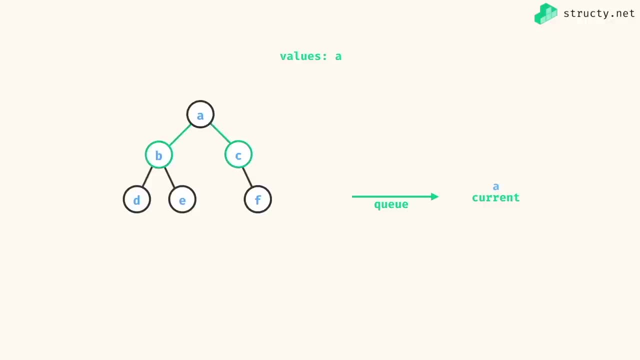 at A's children. a has two children, B and C. I need to go ahead and add them into my queue, And so let's say I added B into the queue first, followed by C. notice that C must enter behind B. 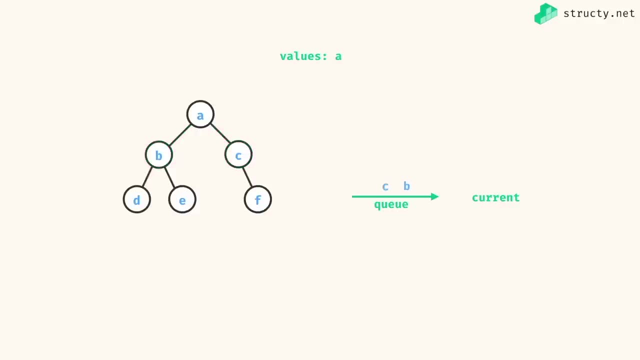 right, And now I finished this iteration. At this point I have the next iteration of my algorithm. I take the front element of my queue and it leaves Alright, so B is now my current. I add B to my running list. then I look at B's children of D and E. I push D, followed by E, behind it At 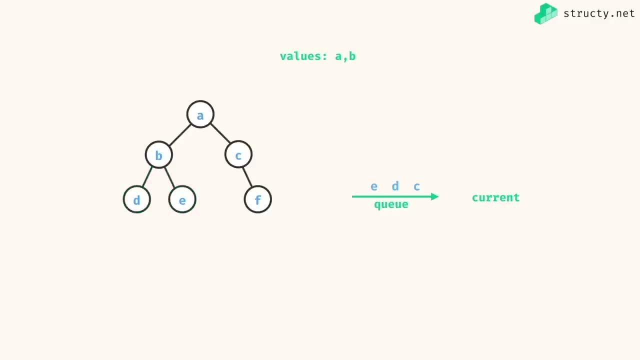 this point, I have another iteration to do, right, And it's so on, so forth From here. C leaves the front of my queue, I add it to my list of values And I look at C's children. C only has one child. 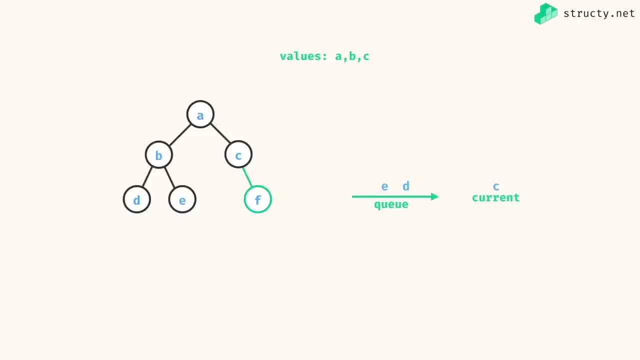 So for that child that exists, I go ahead and add them to the back of my queue, And it's really important that I add it to the back. At this point I have my next iteration. At this point I continue. my queue is still not empty. 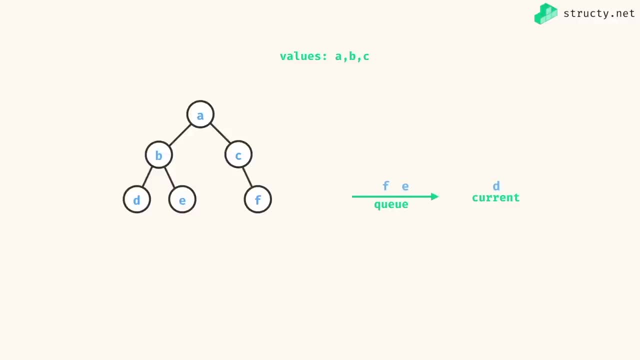 I still have some stuff to remove. So D leaves the front of my queue. I add it to my list of values. Since D has no children, there's nothing to add here. Next iteration: E leaves the front of my queue. I add to my list of values: no children, so I don't need to add anything. 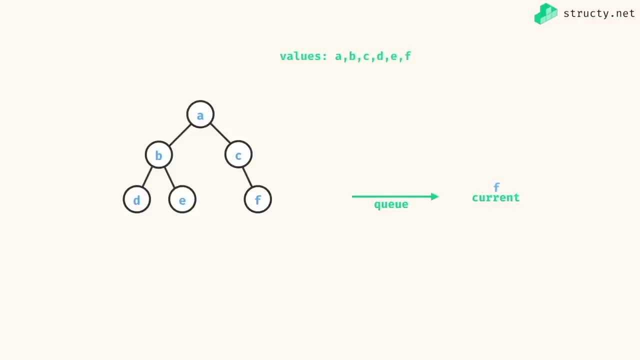 And finally, F leaves the front of my queue. I just add it to my list of values. And again, F has no children. So by now my queue is empty, which must mean that, hey, I must have completed the algorithm, right, There are no more nodes to explored. I explored and added every single node. 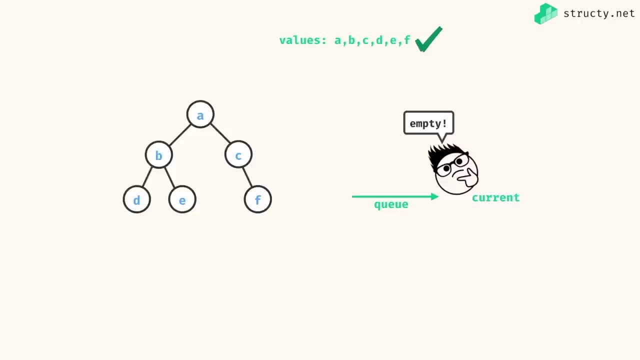 to my list of values. All right, And this output actually looks correct. right, I get ABC, D, F, just like we say. but what about the complexity of this algorithm? So let's take a closer look over here. Well, we know from the get that n is going to be the number of nodes. 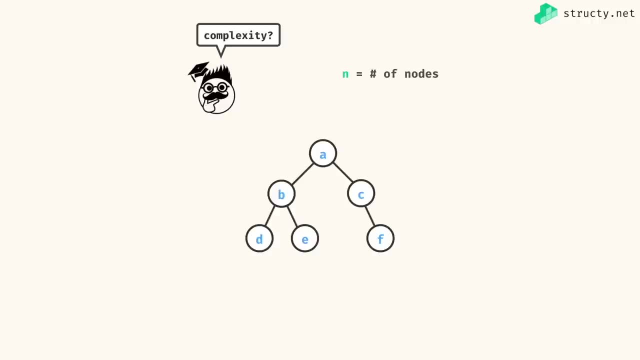 in this binary tree. So that'll be the term for our size of input And we can say that the time complexity is simply just O of n, roughly, because we know, when it comes to visiting these nodes and using our loop, we're going to add every node to the queue once, which also means that that node is going to 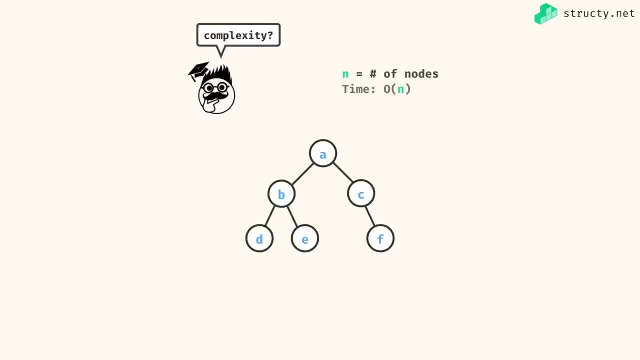 leave the queue also once. So it's not like we're double adding nodes to the queue, right? we're not going to double visit any of these. In a similar way, the space complexity is going to be O of n at most, because you know we're just going to add at most to all of the nodes into our queue. 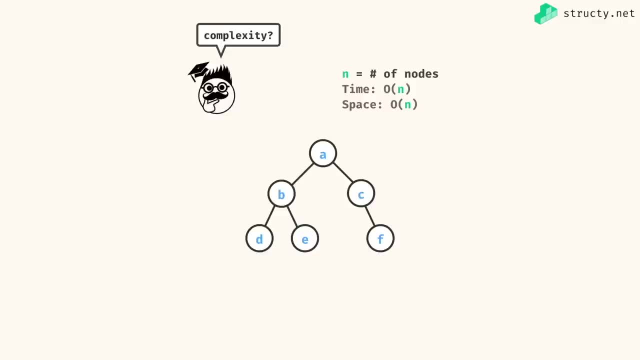 And in general it's probably going to be less than O of n space in terms of how much space we use in our queue. An important thing I'll just mention right now in regards to the time complexity of this one. here we're going to say that the time complexity is O of n, And that's, if we can assume that, adding 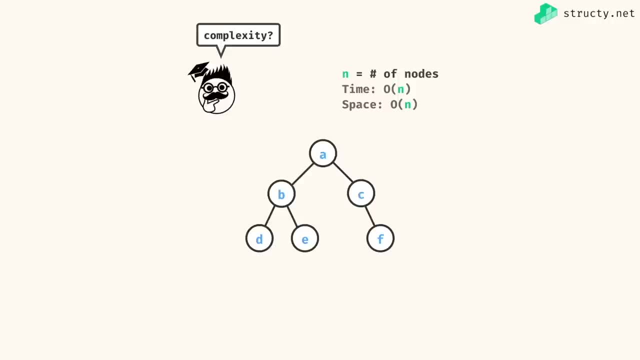 something to the queue runs in constant time and removing something from the queue occurs in constant time. So, depending on how you implement this, if you use actually a built in an efficient queue data structure, you will get this O of n time complexity for our breadth first. But if you 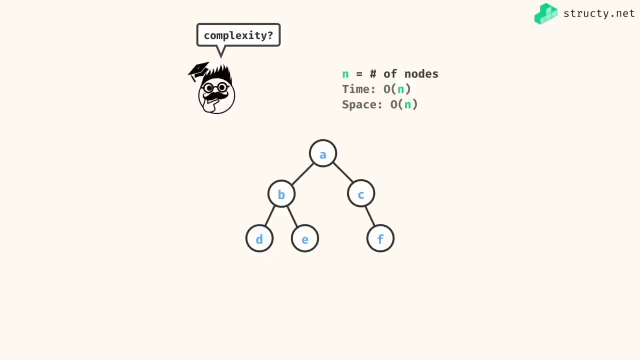 use a less optimal like data structure- maybe not a perfect queue- then you might have an actual worse complexity. So again, this time, complexity of O of n assumes that we have a maximally efficient queue that has O of one add and remove operations. With that being said, I feel pretty good about coding this. 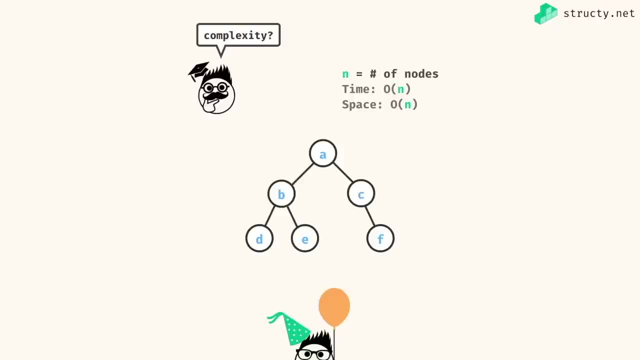 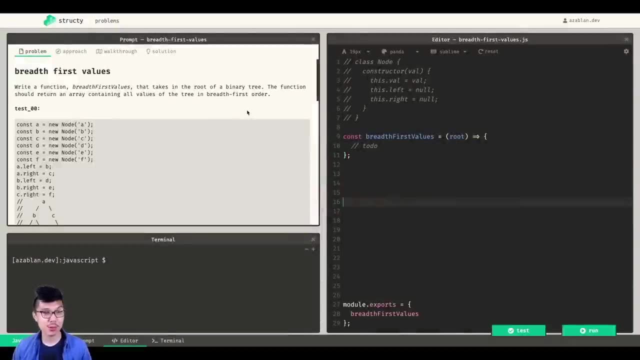 one up. I'll catch you in the walkthrough video And I'll show you a few different ways. Let's implement this one. Hey, programmers, Alvin here Right now I want to walk through the JavaScript solution for this breadth first, values function. So hopefully you just finished the depth first. 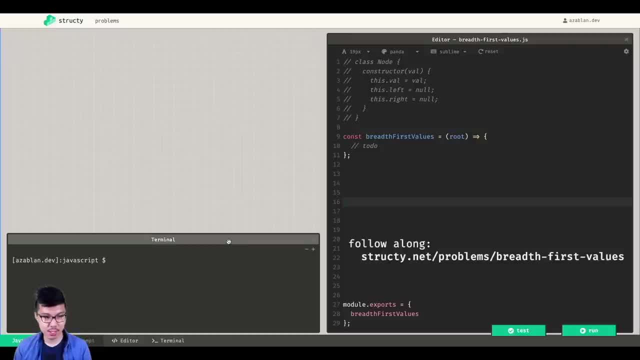 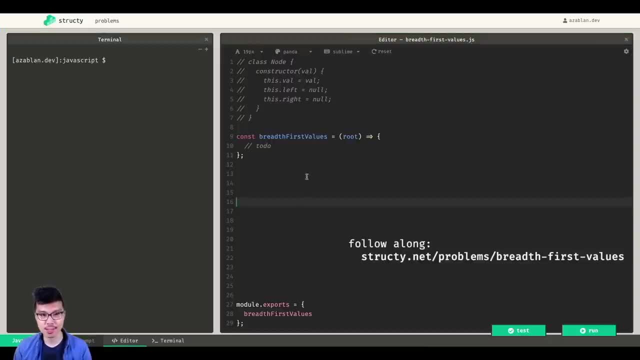 version, And what we're going to do here is we're going to go ahead and create a new function called an array, And in this case this one should be pretty much a cakewalk, But of course we'll still go through the motions of it because it's going to be useful to solve much harder problems later. 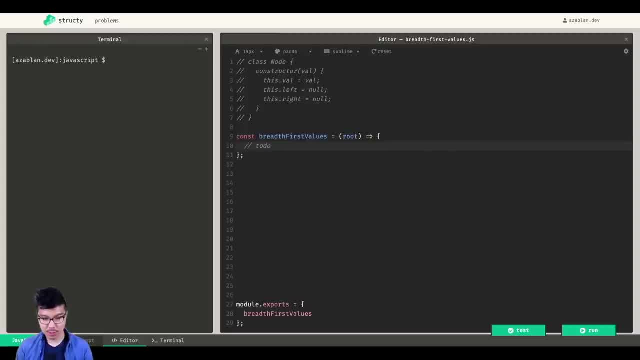 on, as you always hear me say. Alright, so to tackle this one, we'll start with our queue data structure, right? So nothing fancy in JavaScript. what I would do is just use an array and just stick to using very specific methods, right? So I'm going to create an array, I'll call it my queue. 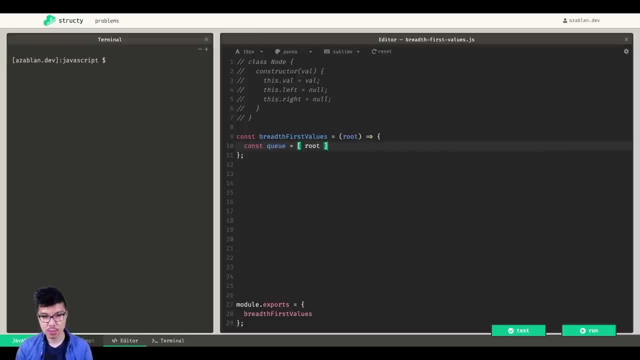 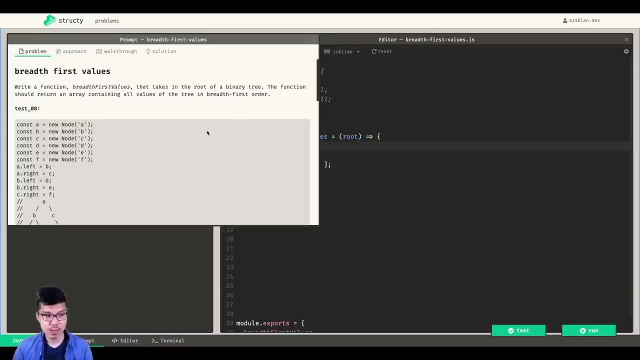 I'm going to initialize that queue with the root on it by default. Now I'll also guard against upfront is: imagine they gave us an empty tree to begin with. So in other words, the initial root is no, which case I would be like this: test 04.. And they just want us to. 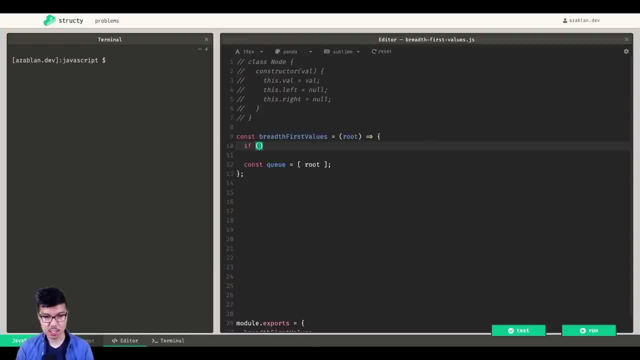 return an empty array. So I'm going to guard for that explicitly. So I'll check: a is my roots? No, And if it is just go ahead and return an empty array Like that, Nice, Then from here I need to start my main loop for my algorithm. So I iterate while my queue is not empty. 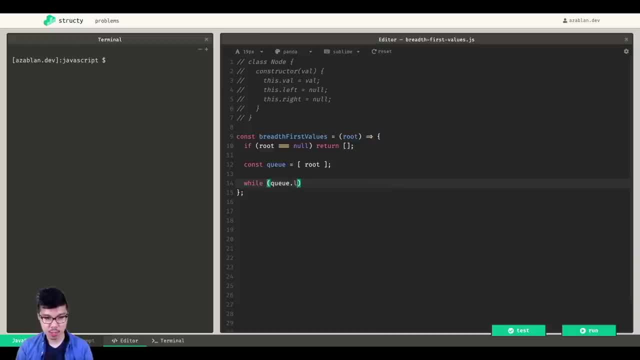 Okay, perfect. This is how a block is going to appear here. right, I can remove a block and away. Right. So it's basically like a loop for my first array, my array, right? So if I want to remove the front, I can say array dot, shift. or for me, right now. 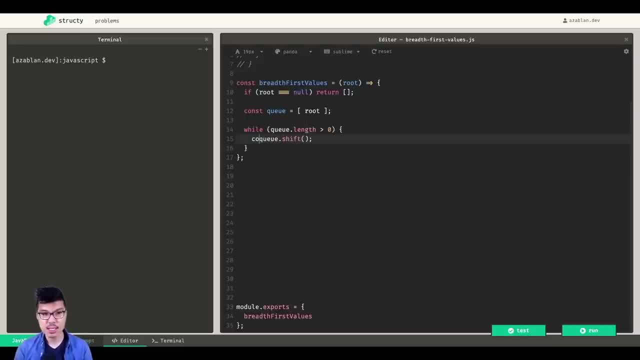 q dot shift that removes the front but also returns to me that element. So I'll call that my current node Nice, And then from here I need to add this node children into my queue and that'll give me my main flow for this breadth. first, reversal right. So I'm going to go ahead. 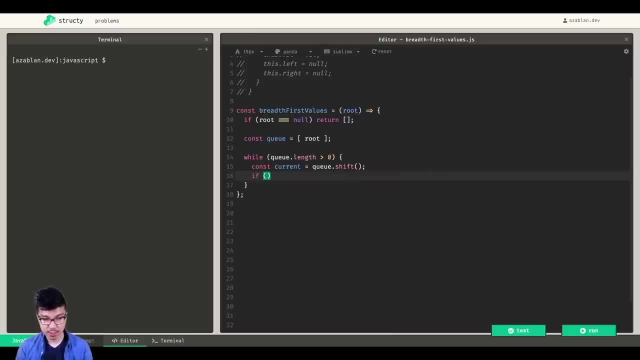 and check a if my left child exists. So if let's say current dot left, that is not null, then what I should do is go ahead and push that into my queue. So I'll say q dot, push my current dot left, And it's just going to be symmetric for the right hand side of course. 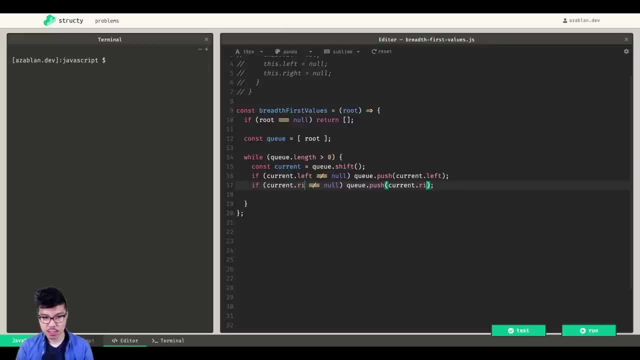 So if the right exists, then push the right into the queue, Just like that Awesome. And so that looks pretty good. And then from there I actually want to store the nodes I visit in an array for the final return, just like the problem asks. 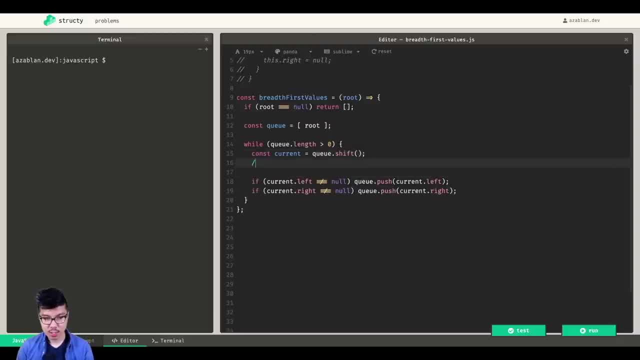 So nothing too fancy. I really want to insert some code over here about And so I'll create a result array. call it: values start out empty whenever something leaves the queue. I'll just take that and push it into my values. So I say values, dot push. 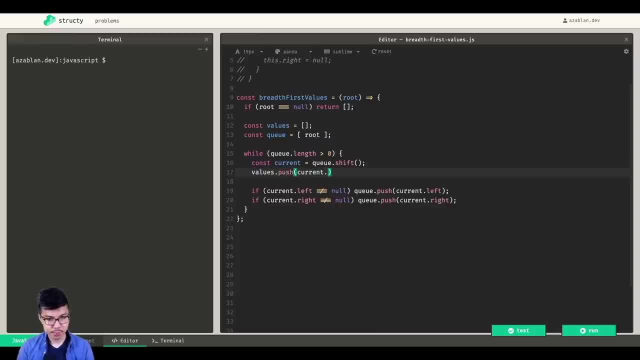 and I'll push that current Val into my queue. And do note that what you can't do is just take like the queue and treat it like your final return value. it must be a totally separate thing, right? I use the queue just for the sake of traveling through in a breadth. first order, 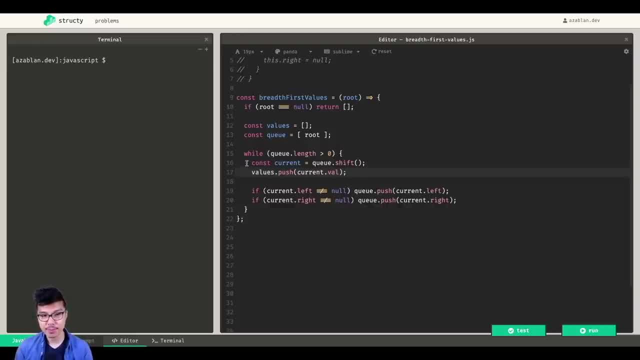 And the order that you visit is actually derived from the order in which things leave the queue, So that's why I'm doing it over here right. As soon as something leaves the queue, that's when I consider it visited, So I add it to my values list. 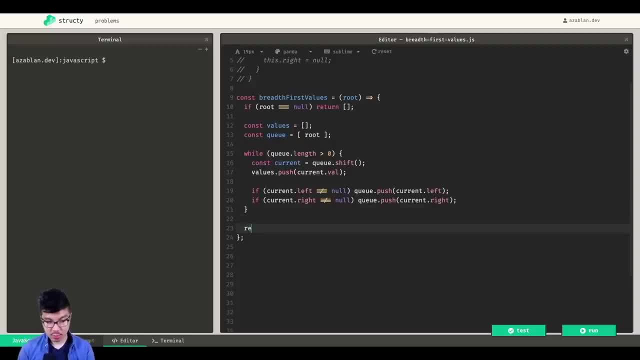 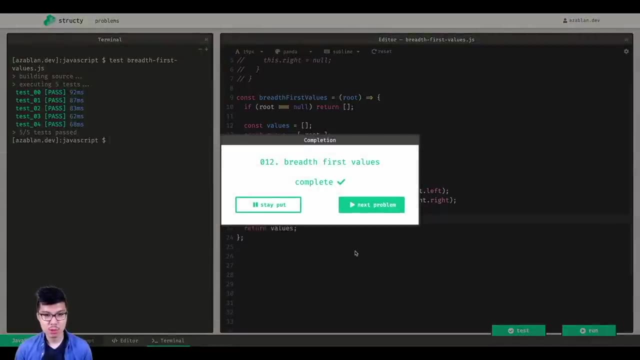 Nice, And after my, while it's done running, I'll go ahead and return my entire values array. So let's give this a test. I'm going to run all the test cases, see what we get, have a few test cases to pass And there we have it. Here's a nice iterative solution for 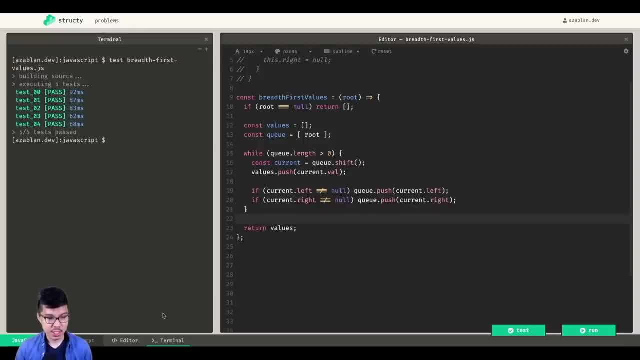 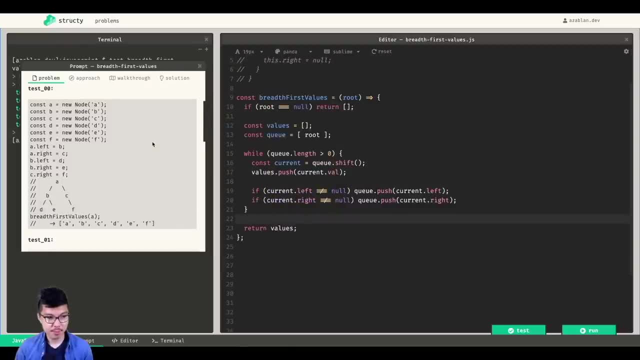 our breadth first traversal. Just something I want to mention. by the way, that's fair, look at the prompt. So looking at I don't know, like the very first example in this kind of condition of breadth first, what they asked us to do is really give us a breadth first traversal. 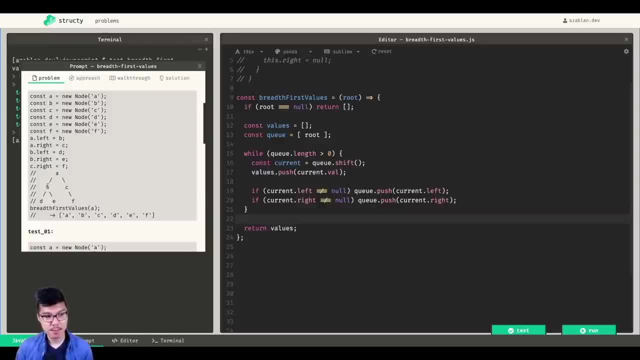 that moves from left to right. So notice it goes a, b, c in terms of the resulting output and not a CB right. those would both be technically a correct start to a breadth first, And then you can kind of choose, depending on what problem you're solving, whether you want to go. 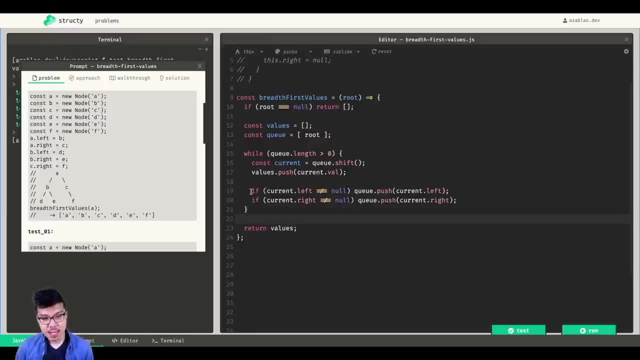 left to right or right to left. For me, because I push the left, followed by the right, that means first right because, remember, the queue is just like a line and checkout. So if someone enters first, that is, the left enters first, they're going to be served before the right go on. 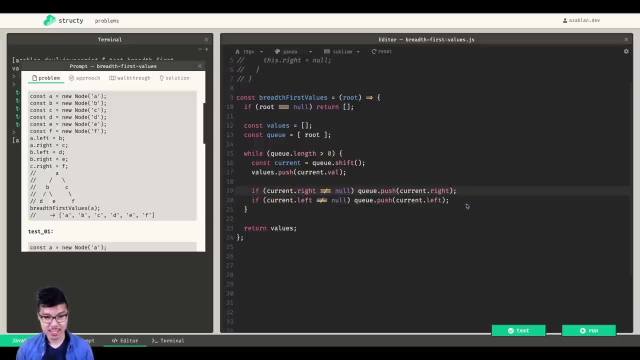 you can just flip these around and I'll give you the right to left traversal, Cool. So, depending on what your problem warrants, you can always manipulate that code a little bit, And this is actually probably like the only solution you can have. you know, maybe aside from just some, 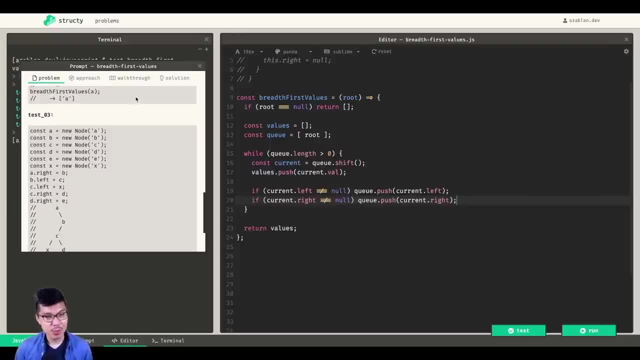 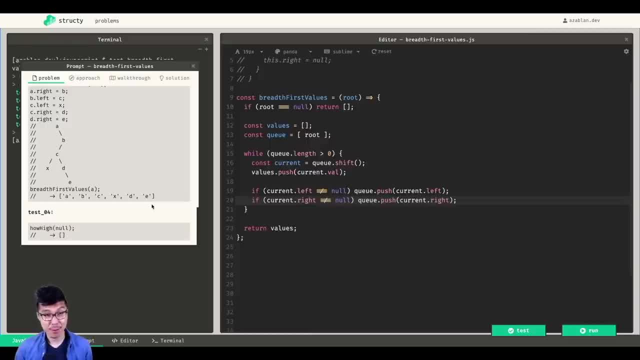 not really a straightforward way to implement a breadth first traversal recursively. And that should make some sense, because a breadth first traversal needs a queue order right needs to use a queue. If you write any recursive code, you know under the hood it's using a stack, And so 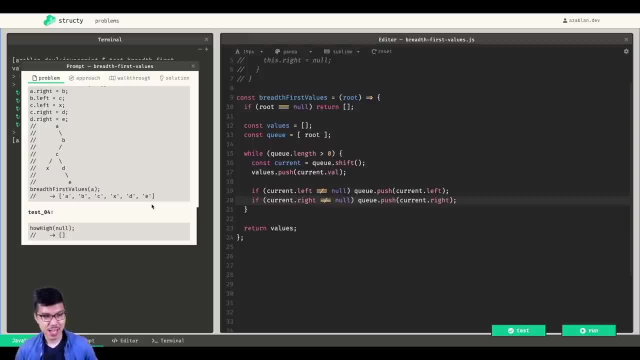 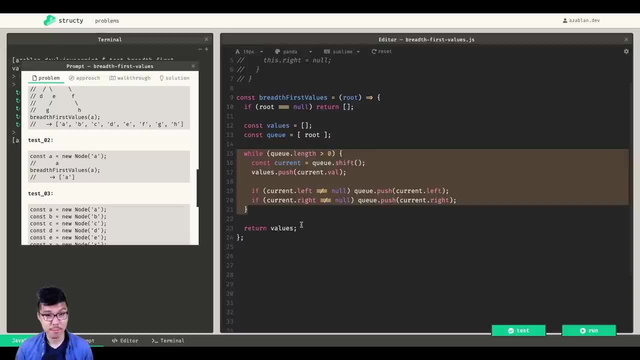 that stack versus queue is really just going to fight against you And you're going to have a really tough time trying to implement the correct ordering. So always just write the iterative version for your breadth first traversal. Alright, so I recommend before you hop into the next video: 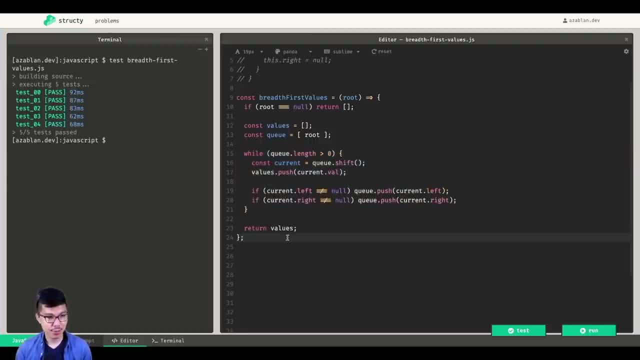 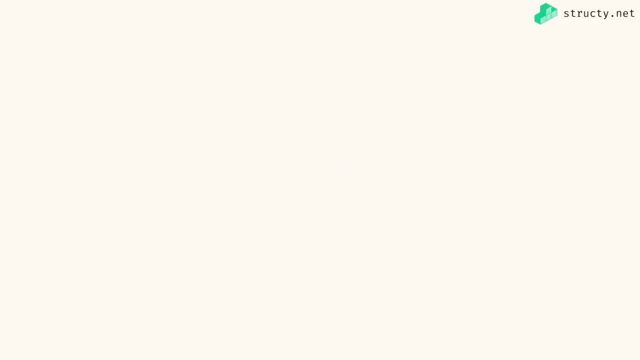 make sure you're able to write this code on your own, because we are going to level up difficulty a little bit, but I'll catch you in the next one. Hey programmers, Alvin here right now on a walk through. the approach for this tree includes problem. So premise of this problem. 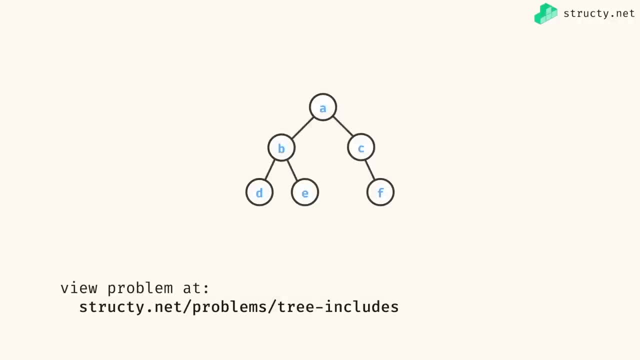 is. I'm going to give you a binary tree and also a target value to look for. I just want you to tell me, true or false? is that target value found within the binary tree? So for this particular example, input, the answer is obviously true or yes, right, you could definitely find E within. 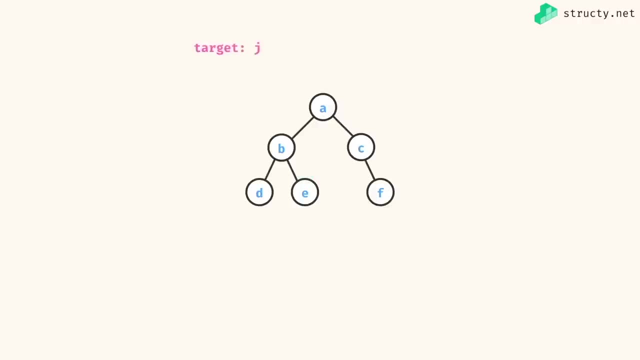 this binary tree. If I give you another target value like J, you would respond with false right Because that value, J, is nowhere to be found within the binary tree. And really what I'm asking you to do here is we're stepping through the canonical like breadth, first search. 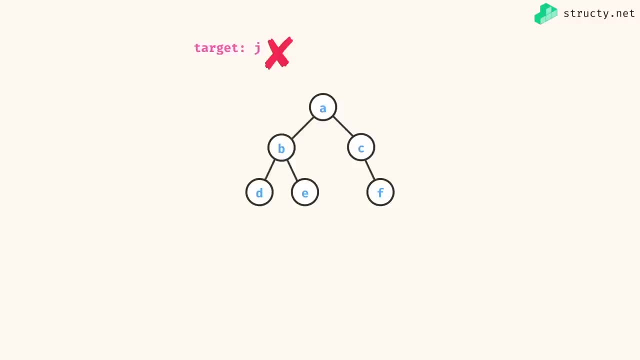 and depth first search problems, And I think I'll walk through approaches for you right now. So let's say I was testing, or I wanted to trace through, rather, the input where target was E. how can I go about attacking this one? right, We know that in most, 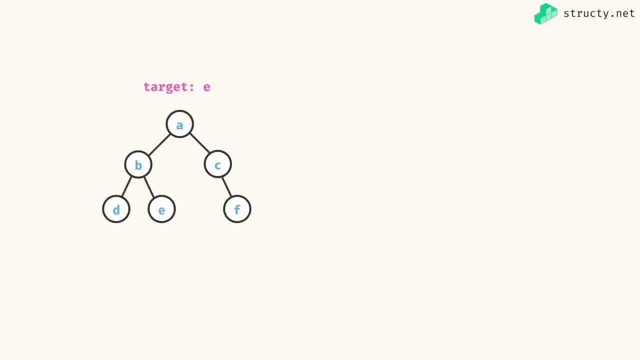 of these problems. when they give you a binary tree as input, they're only going to give you, really, the root node, But, that being said, if you have access to the root node, then you know you have access to all nodes that comprise of the tree, right? So what I can do is just perform any 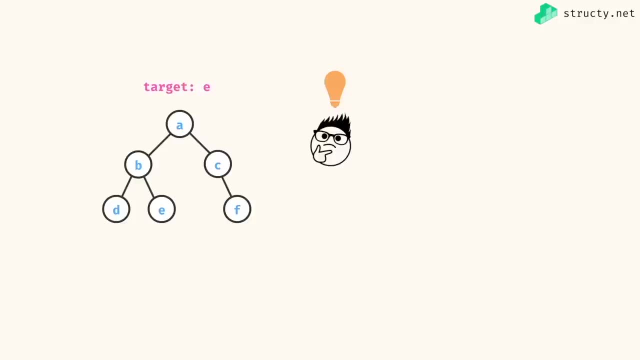 of my traversal algorithms. so maybe to get going now, let's just do either the breadth first search or the depth first search iterative style. So I think for this trace I'll stick to the breadth first version, which means we're going to use a queue right. So as we trace through this, I'm thinking about this one. 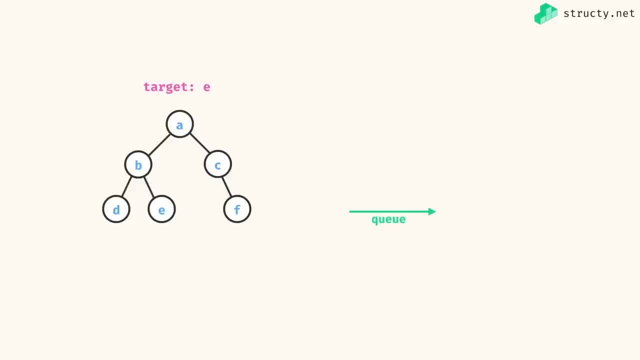 iteratively. right now, Hopefully you recall from our previous problems. when it comes to your breadth, first traversal, you start with your root node on your queue And when something leaves the queue you mark it as your current right And when you leave the queue you mark it as your current. 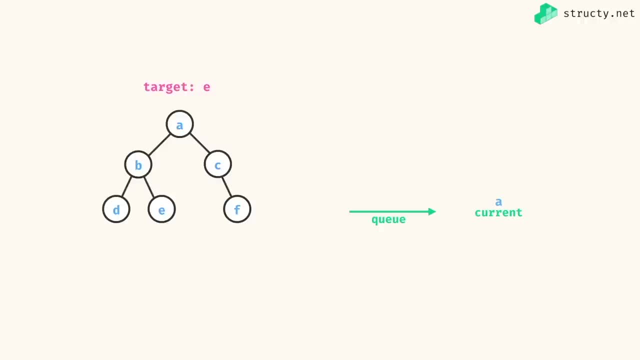 and here's where I work in the new logic For this, this particular problem. when something leaves the front of my queue, I'm going to check: hey, is that current value the same as my target value? So, is A the same as E? it's not. so I have not found the thing. I'm looking. 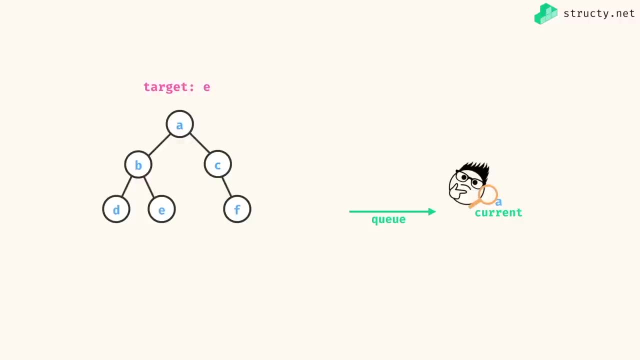 for right, And what I can do is now consider A's children, right. so I look at his children. they both exist. I add them to the queue. so I add B to my queue, then I add C to my queue And now I'm on to my next iteration, right? 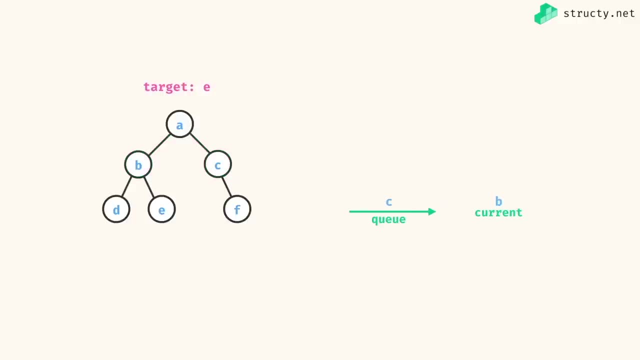 element B leaves the queue. then I have to check: hey, is B my target? It's not right my targets. So I keep running. I look at B's children, So I take that D and add it in, And I take the E and also add it, And this process just continues. C leaves front of my queue. is C. 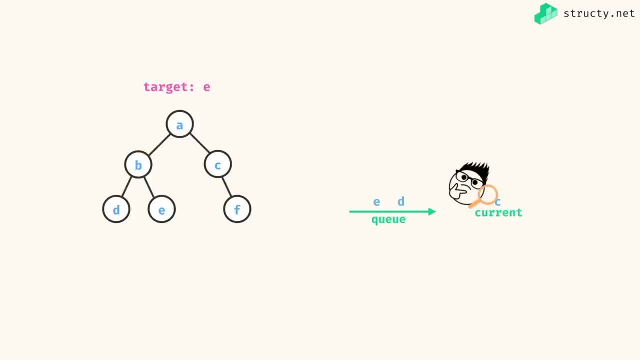 my target. It's not, So keep going. I would add C's children to my queue. So I just add F to my queue And this process continues, And so D leaves the front of my queue. I check: is D my target? 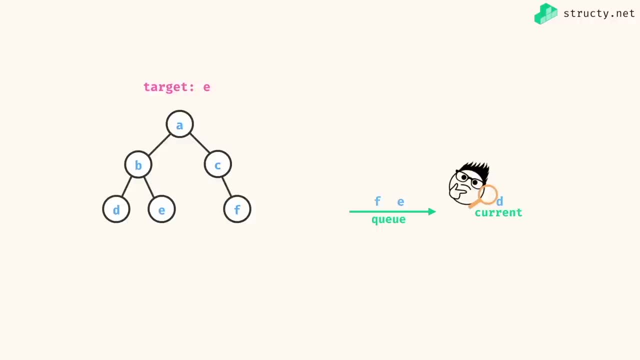 It's not And D has no children to add. right, Recall that in our breadth, first traversal, I only add the children if they exist, because I don't want to add any like null pointers into my queue And so I just continue my algorithm, right? I still have stuff in my queue to check And 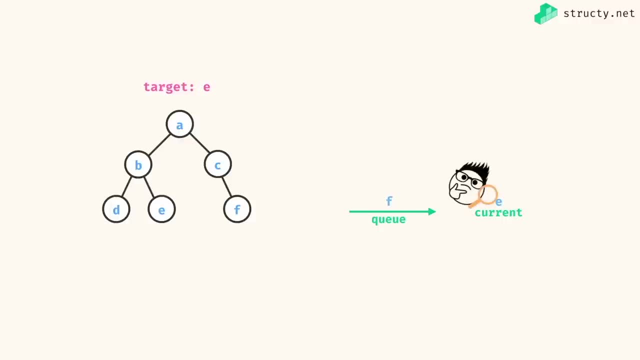 finally, when he leaves the front of my queue, I check: is he my target? And indeed it is right. At this point, I've just confirmed that he is found inside of my binary tree, So what I can do is just end my algorithm by like: 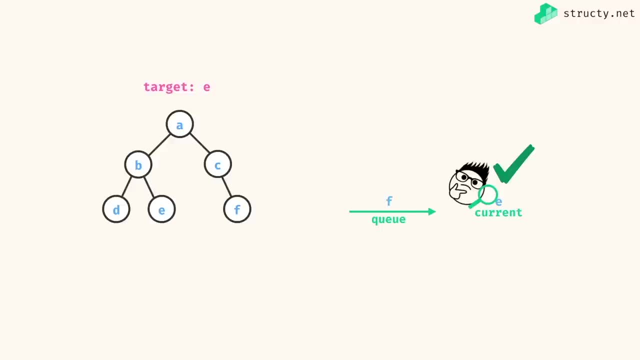 returning the true value, right. There's no point of actually looking through the rest of the tree, because I already figured out that, hey, my target value is indeed within the tree, right? One thing you might notice is it looks like I only checked for E once it left the front of my queue and not 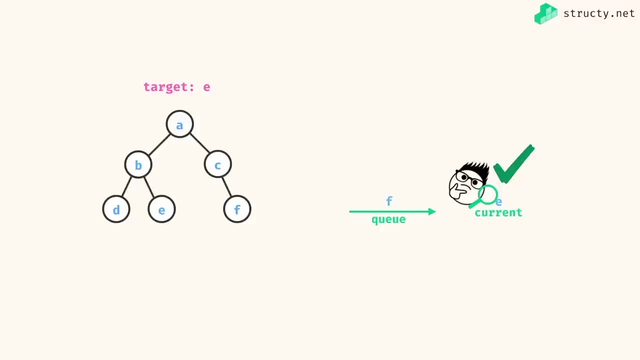 when it was initially added to my queue. Technically, you could have returned early when you added it to the queue, But we'll kind of see when it returns. I walked through the full code for this one. it would end up with cleaner code if you just checked. 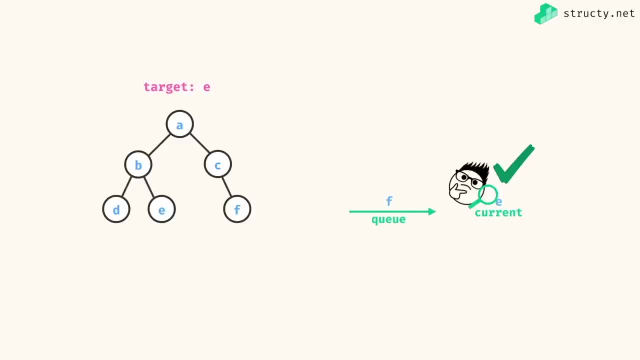 for your target value when something leaves your queue. So we'll see that when we go through the code. It's just a small implementation detail. That being said, for this iterative breadth, first strategy, what can we say about the complexity? Well, if we define n as the number of nodes, 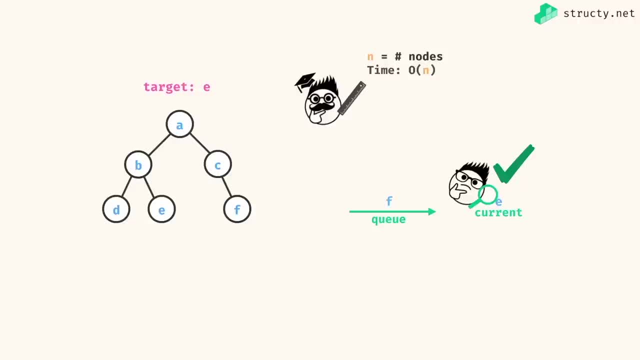 then we know that the type complexity is just O of n. it's really just a classic breadth, first traversal, So nodes are going to enter the queue once and leave the queue once. So that's O of n Right. And again that's considering if we use a efficient queue right where our queue add and 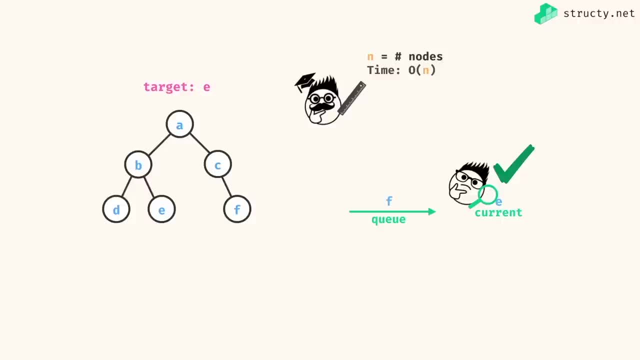 remove. operations run an O of one constant time, So we have linear time, And for the space complexity it's also going to be O of n- linear, right, because we're just going to store our nodes within the queue, And so we just looked at the approach for a nice iterative breadth first, 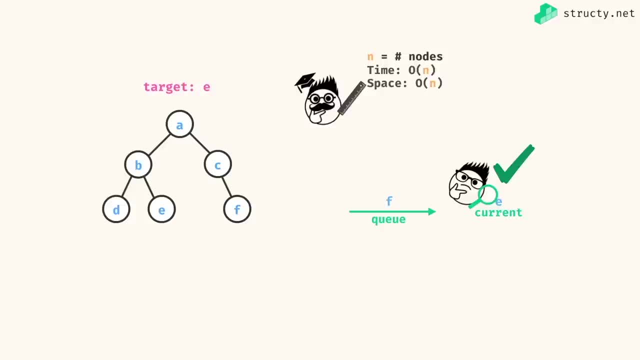 solution to this problem. But I want to show you the depth first version. and the depth first version that would be recursive, right. So obviously you could right the iterative depth first solution, which case you just use basically the same code. we just 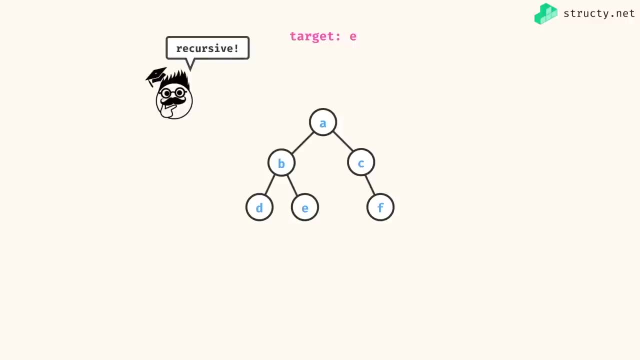 spoke about, but just use a stack instead of the queue. But let's try to solve this one recursively, right. And the reason I think it's really important to expose yourself to recursion like this is as we move to more complex topics, you're going to find this style of recursion. 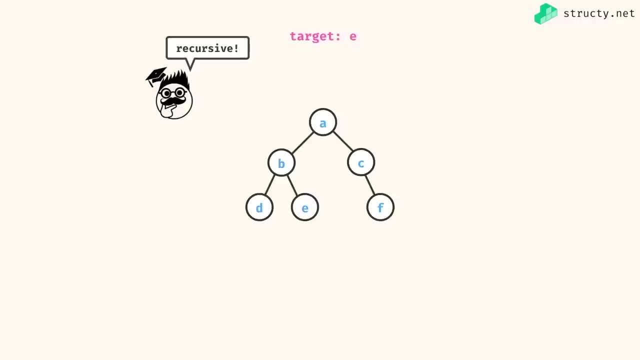 very, very useful, right? So we have the same input, right? let's say, my target is E and I have the same binary tree And I want to check recursively: is E within this tree? And so how do we start attacking this? Well, we're going to need to. 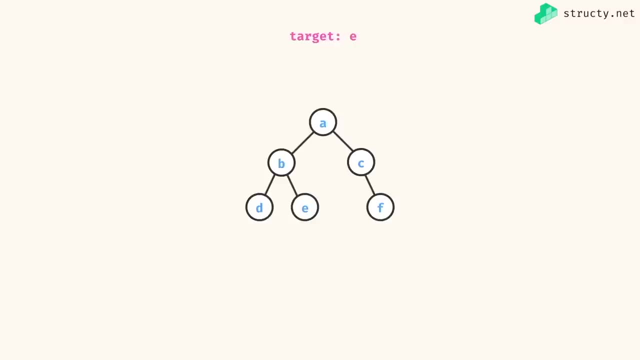 think about our base cases, right? So we're going to have really two types of base cases. we'll have like the affirmative base case, meaning hey, we found a match, And so whenever I counter a node whose value is E or whose value matches my target, then I'm going to have that node, or 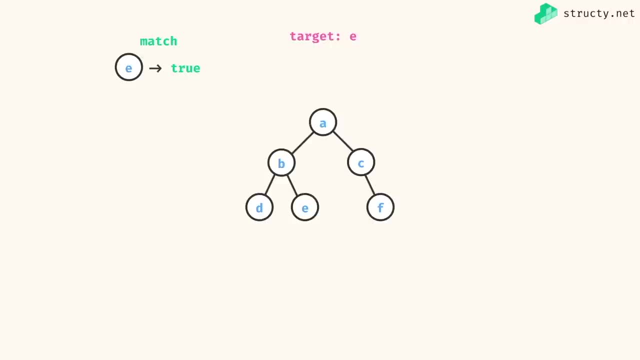 that recursive call return true right. So that's my like affirmative base case. So I'm just going to plug that return value individually in my tree. you know that this E nodes going to return true. And now I'll think about my negatory base case right For times. 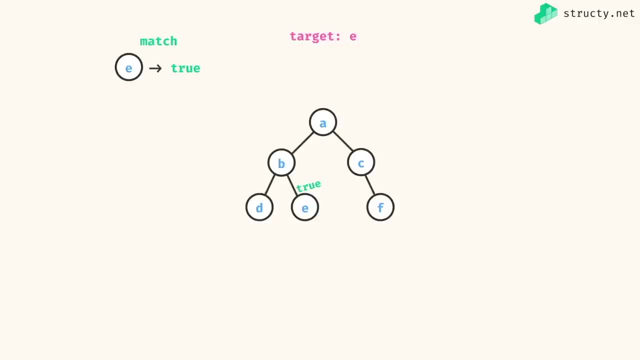 where I call upon an empty node or the null node, I should return false And recall from our previous lectures we said that we're going to, you know, sometimes represent explicitly our null nodes, So I'm going to fill those in. for example, the C node in my picture would have a left child. 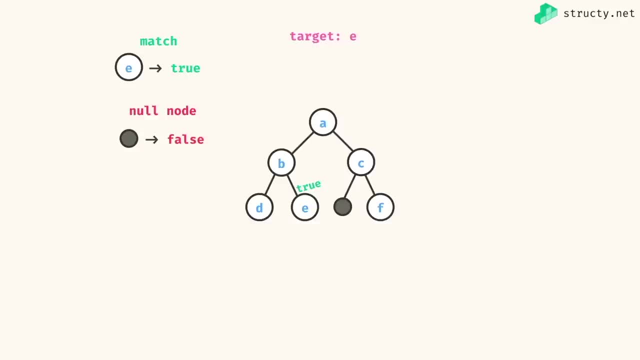 that is null. So I'll kind of draw that one explicitly- And I know that a node like that is going to return false, Because logically I shouldn't be able to think about all of my recursive calls as if they're their own sub problems, right? So if someone asked me, hey, 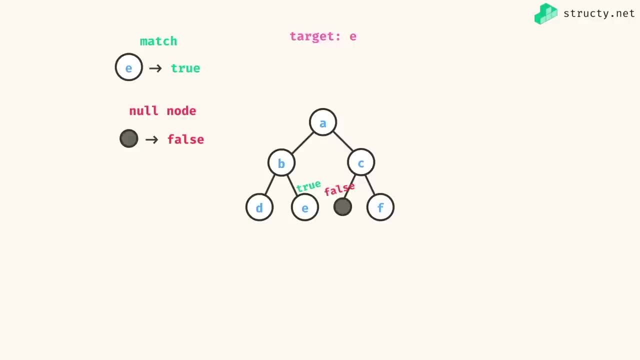 can you find this E value within an empty tree? right, a null node represents an empty tree. the answer would be no. I can't find the E value in an empty tree because there's nothing there, And so from there I'm also going to draw explicitly all of those similar. 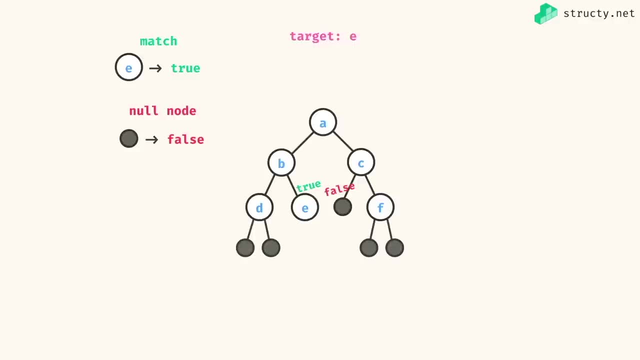 null nodes, null pointers, right. So it looks something like this: Notice that from the E node. I don't need to give it a null left and right, because I already said that that node is going to return true, right. So that's why I draw my tree like this And I have 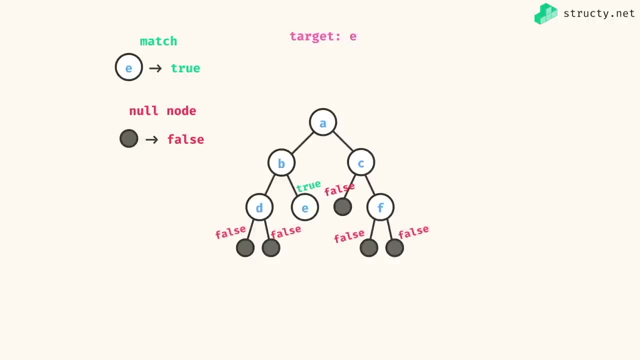 all of those false return values, Cool. So we just labeled all of the base cases right as the leaves of our tree, And recall that a leaf is just a node with with no children, right, And from here, how do I actually combine all of these Boolean values to get the true at the very top? So I know. 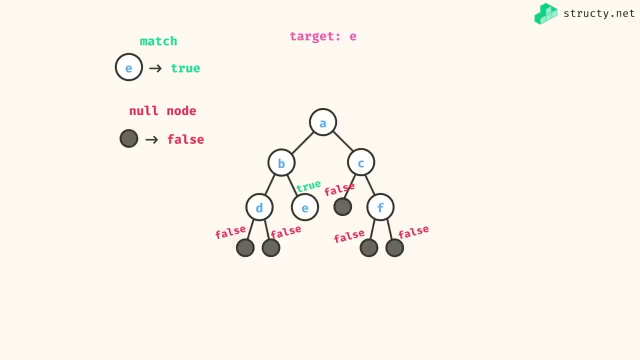 that the DA node is a. no, I need to make sure that I'm not using a null object here. So what I need to be able to do is I need to think about what I want to get on here, what I want to create a. 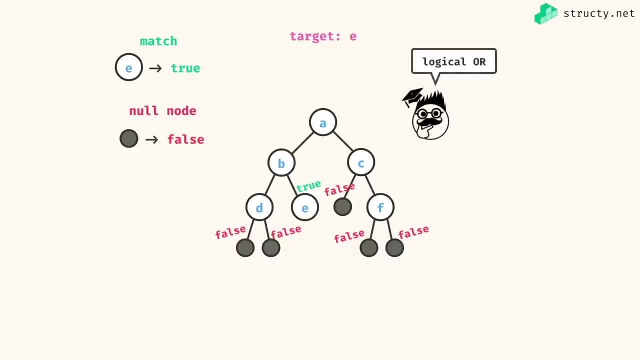 node of that value and how do I want to get all of these values to that value right? I'm going to make a tree with no children, So I'm going to write a tree, The value of the tree, and it should. 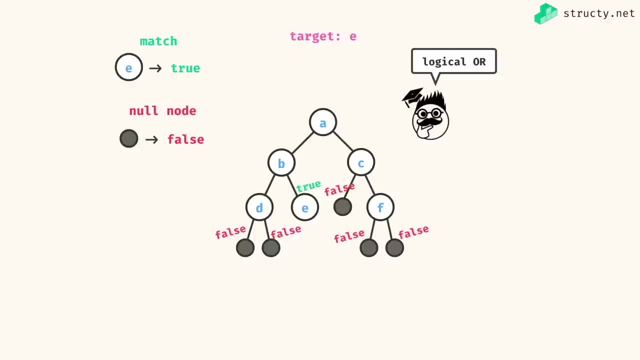 be the $$, $$, $$, $$, $$ and the tree. if we have a $$, $, $, $$, $, $, $, $$, $$, $$, $$, $$, $, $$, $, $$, $, $$, $$, $$, $$, $, $$, $$, $$%, let's start evaluating our return values and combining them at the parent. So this should be. 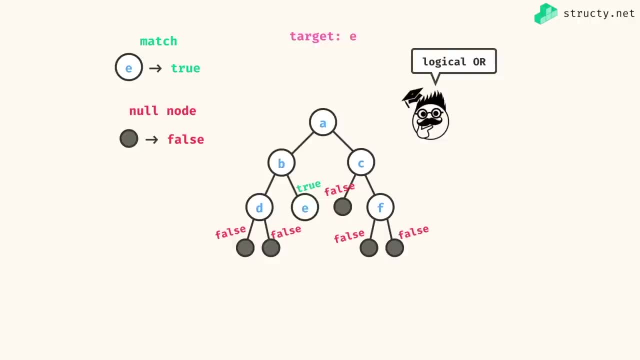 somewhat of a similar pattern to like the tree, some problem I showed you, And so what we could do is focus on this D node over here. this node has values ready on its left and right, has two falses, And when it actually gets those falses returned to it it just should do the logical, or 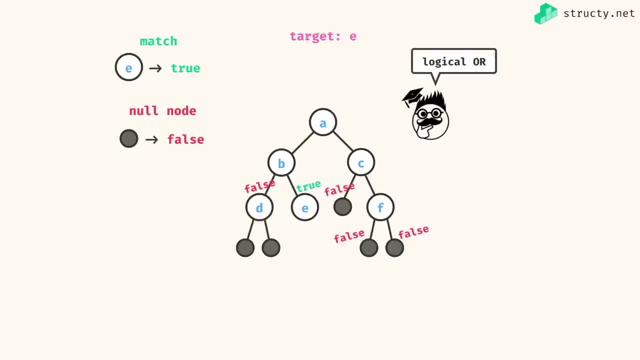 so it's doing false or false, which evaluates to false right, Which means that, hey, in this subtree rooted in D, I cannot find the E value which makes sense. That's why it's false. I'll continue this process. If I look at this B node now, this B node has values ready on its left and right. 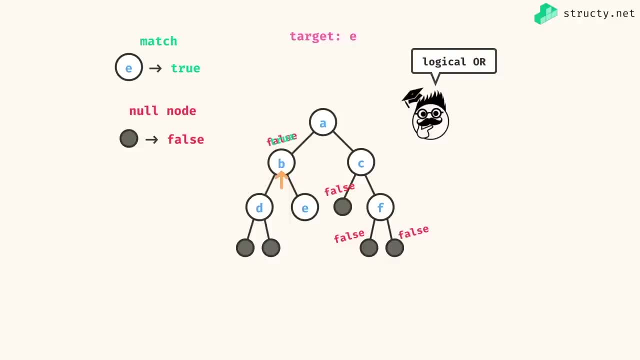 and they're going to bubble up a little bit And I take the or of them, So I do false or true, which evaluates to true, And this process continues everywhere in the tree right. So at this F node, false or false. 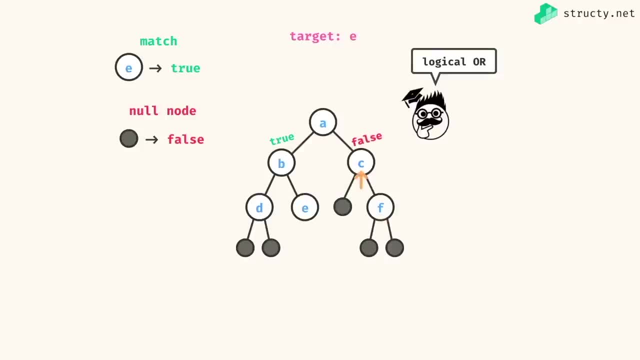 gives me false. at the C node, false or false gives me false. Finally, at the top level, root of a, I do true or false, giving me back a final true, which is indeed the correct answer. So hopefully you realize how similar the solution is to our previous. 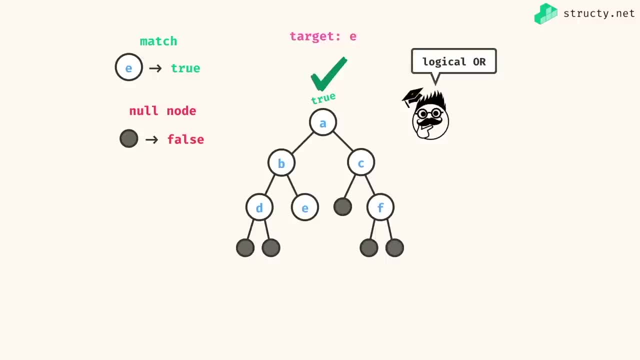 tree some problem. right And the tree some problem. I combined my left and right child return values by doing the arithmetic addition, But this time around I just need to use the Boolean operation of or right. So by just adjusting the type of the Boolean we have a very 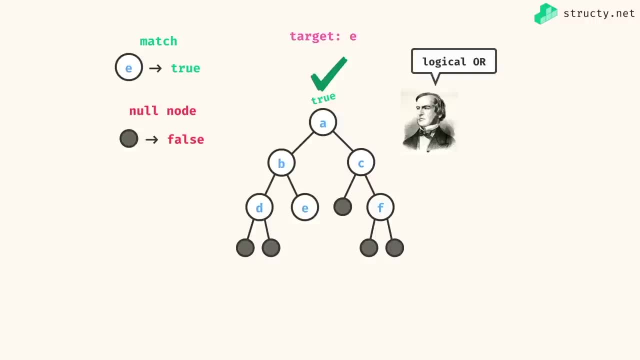 very elegant solution that shout out George Boole, And so, with that, I think let's go ahead and implement this one in some code, And I'll show you it using the iterative flavor, using maybe a breath first, and also the recursive version, which is my personal favorite, using 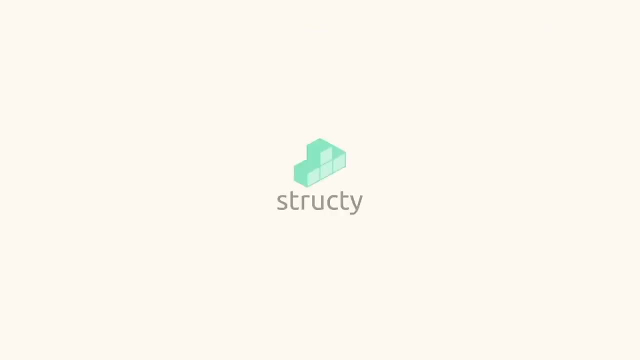 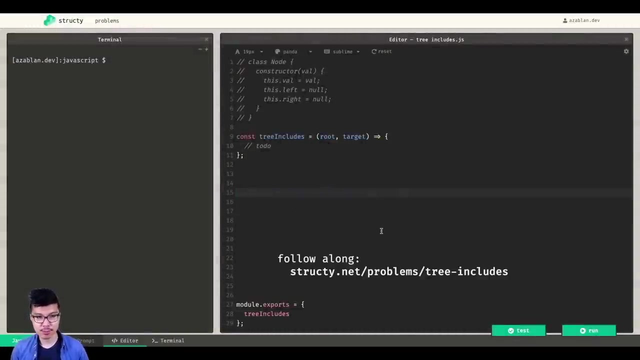 this recursive tree structure. Hey programmers, welcome back. Right now I want to go over a JavaScript solution, for this tree includes problem right, And we'll solve this both depth first and also breath first, And I think we'll start with the iterative breath first version, And so this is really just going to be an 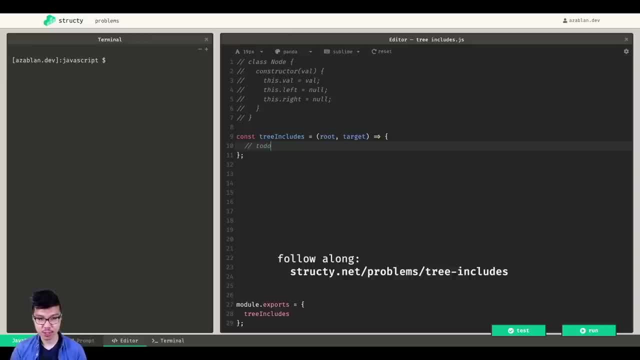 implementation of the classic breath first search algorithm. So I'm just going to lay down my classic breath first traversal code and then just add some conditional logic afterwards. right, So you should be familiar with it by now. But for my breath first traversal I'm going to use a cube. 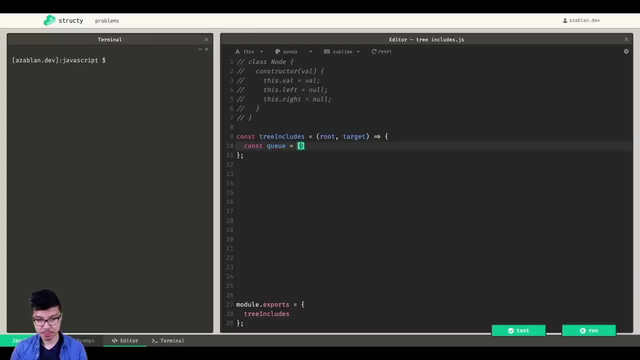 So I'll say const q equals and empty array, or really an array with the root thrown on the inside And from there I have my main algorithm right. So I loop while my queue is not empty, So I'll. queue length is bigger than zero. 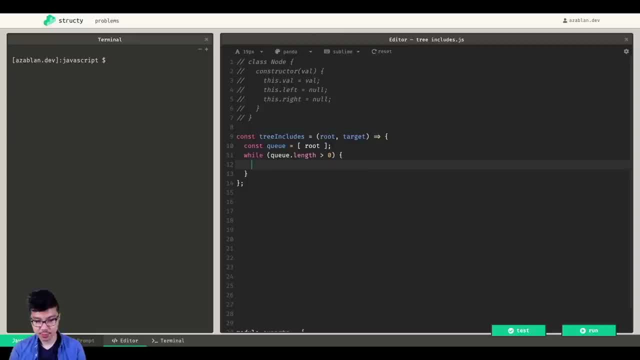 and keep on going And on a single iteration of this traversal, what I do is q dot shift. so remove from the front of my queue, the front of my array, remove the first element And I'll save that into a variable called current. So that will be just an instance of node And for now, 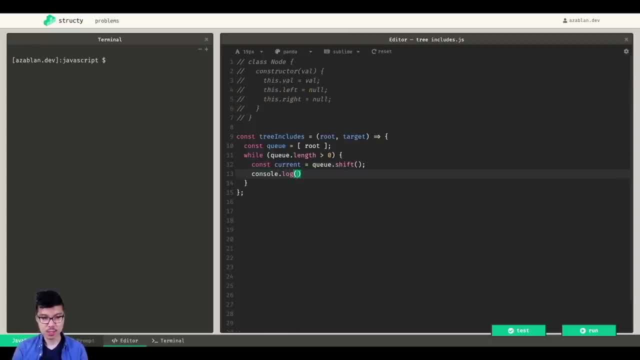 just build up my solution slowly. I'll just- I don't know- console dot log, what current dot val is. But once I consider this node, what I want to do is really add its children into my queue. only if they exist, though, right. So in general, I'm going to write like: q dot push, I'm going to 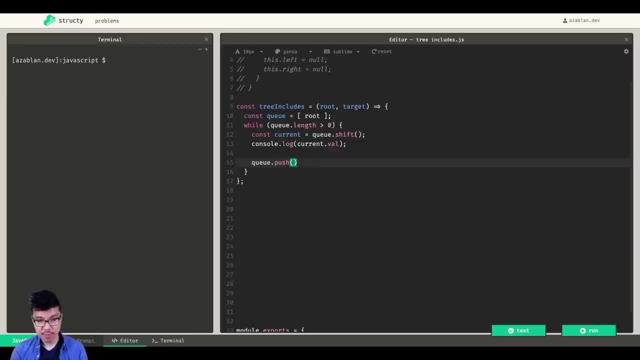 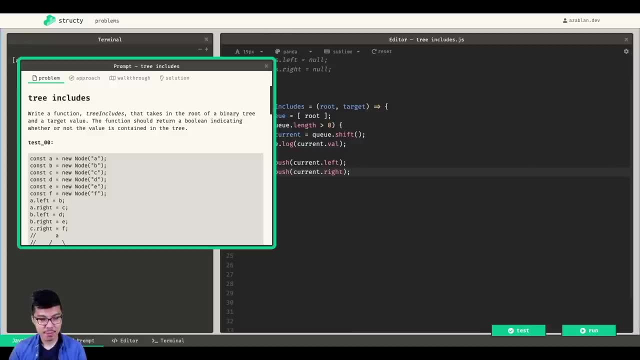 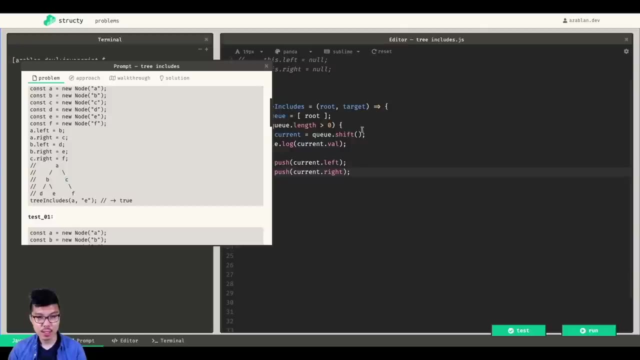 add to the back of my queue, So I get a nice queue order. push the left child, So current left, likewise the right child. But imagine that I have an asymmetric node or just a leaf node right, So something like C would only have a right child, so it's left would be null. So if current is C, 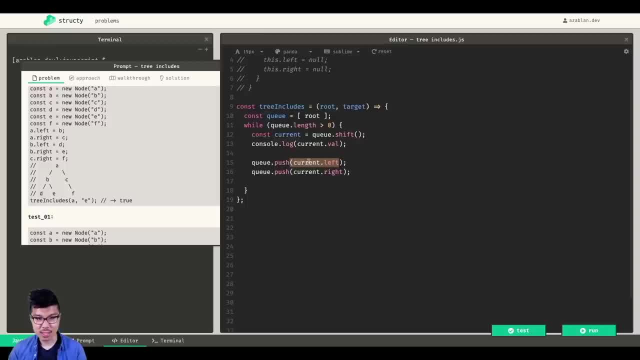 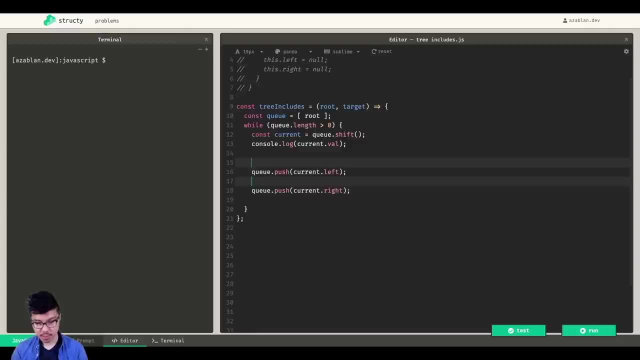 then I'd be pushing null into my queue as the left, which is no good right, And so I need to guard here and only push the children if they exist. So something like this: hey, if the current has that corresponding left and right, then I can go ahead and push it. So this is looking pretty good. 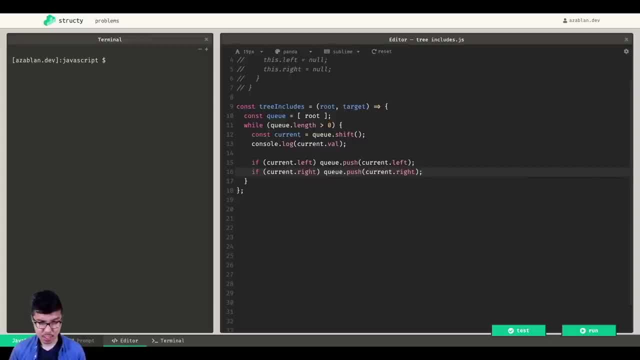 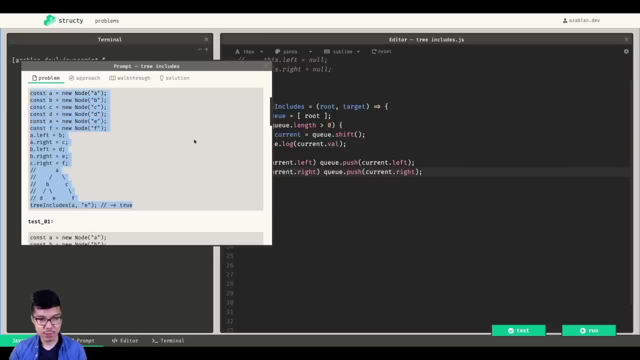 And that should actually be the main traversal part of the code. So I'll just test this manually, So very manually, So maybe just this call. So I'm not going to return Booleans yet. We'll build up to that, But I should. 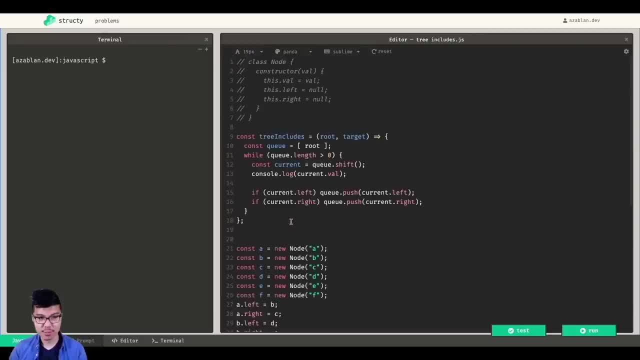 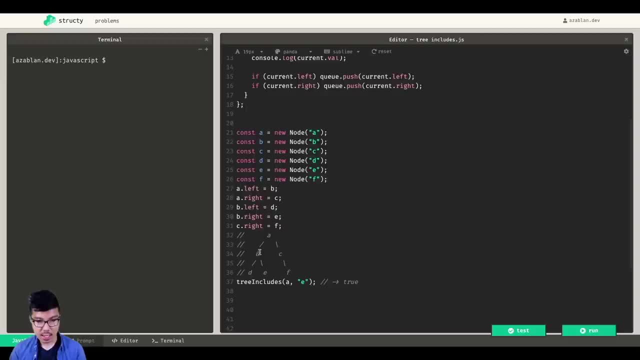 at least see my values printed. If I kind of run this manual test case, I'll bring in my node class. I should see the values printed in a correct breadth first order. So that means A, B, C, D, E, F. recall that breadth first reversal travels across our tree before going lower. So 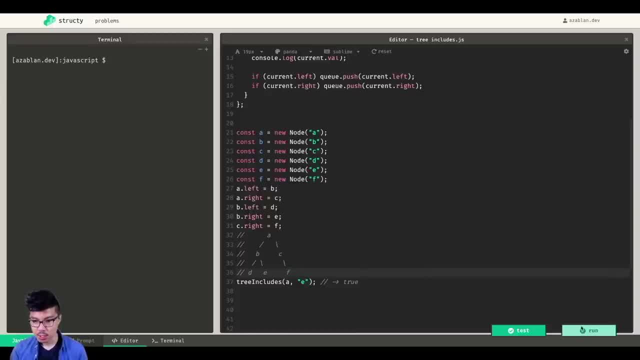 this is a very, very simple method to get to the next level, So we just need to run this manually as a script, So we'll go ahead and check. no, we must finish a level before traveling to the next level, So let's just run this manually as a script. See what we get here: A, B, C, D, F, nice, So I'm. 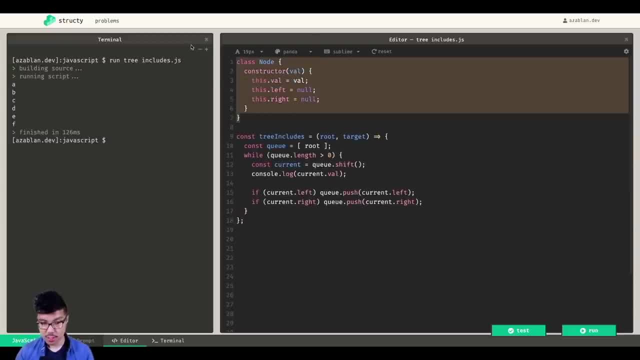 getting the right order of traversal And now I can work in, I think, the conditional logic because they want us to return Booleans over here. So pretty straightforward stuff, We'll go ahead and check is equal to my target. then I found the thing I'm looking for. So just return, true, right? 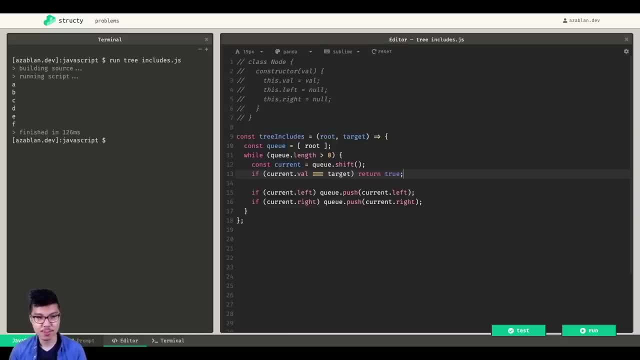 you're done. you don't need to travel through the rest of the tree because you can return, true, But on the flip side, if my value that I'm currently at is not the target value, then I must continue looking through the rest of the tree, right? So if I finished the entire, 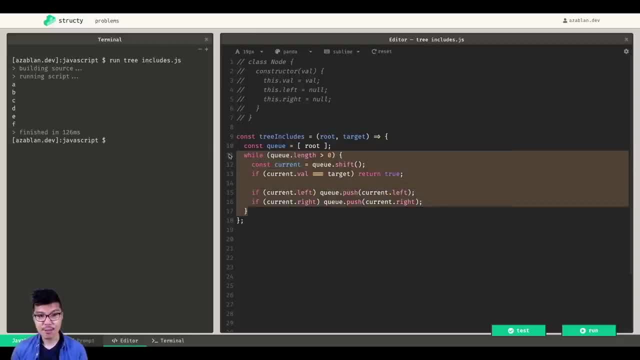 while loop. that means I've traveled through the entire tree and I never found the thing I'm looking for. I should return false, So I need a late return false over here. A really common mistake people tend to make is: what you don't want to do is just do like else. 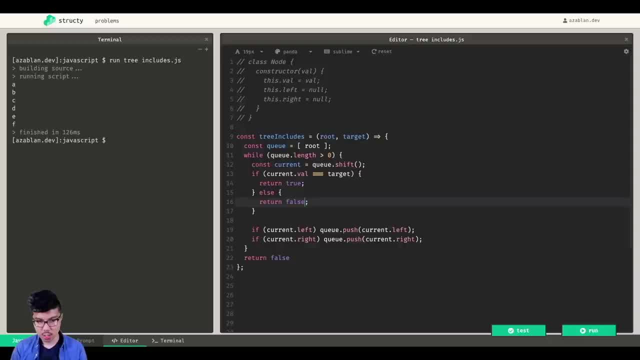 return false here. So this is going to be wrong. Right, Because this would only check, like the very first notice, only check the root, And then you check if the root is not equal to the value. If it's not, you just return false, which is not really useful. 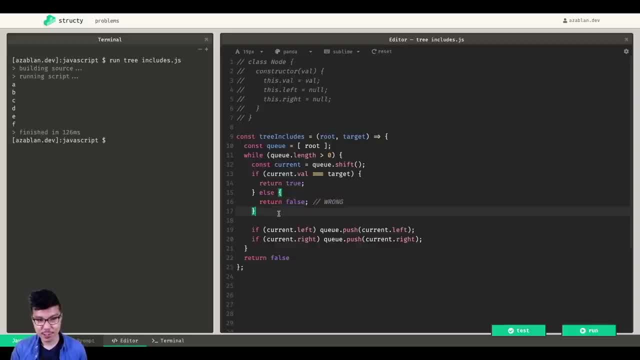 because it could be somewhere else in the tree. So you're going to need that late return false pattern over here. But with that I think we're going to pass some of the test cases. So I'll run the test cases by hitting that test button And there's probably one scenario we did not foresee. 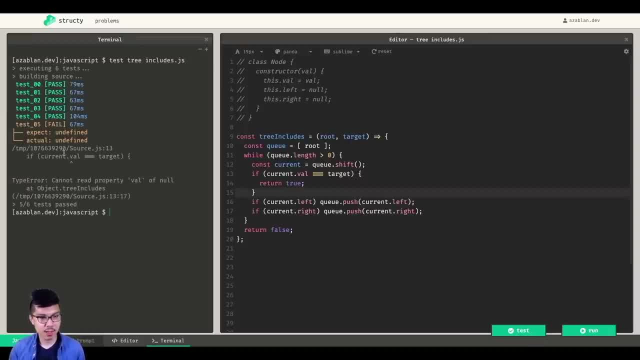 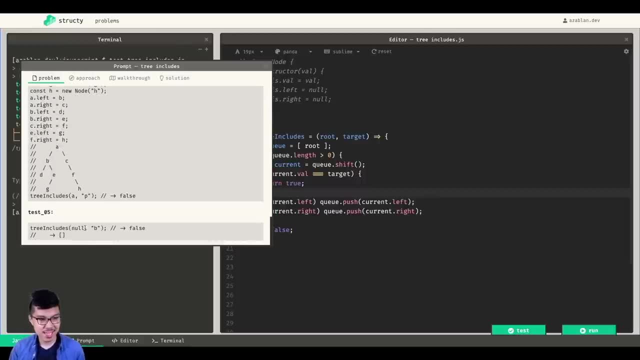 Cool, And there it is right. Can I read property valid? No, we're failing test 05.. If I look at that spec test five gives us a null node as a route right. So just the empty tree. you cannot find the. 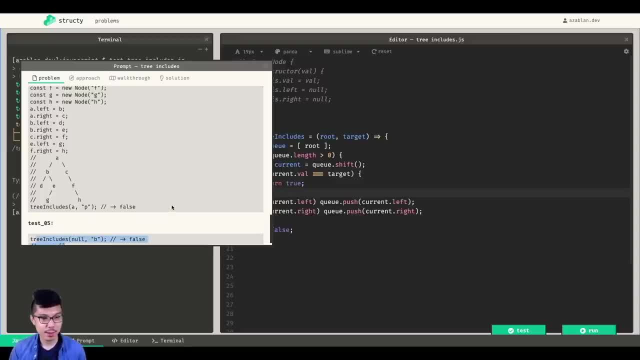 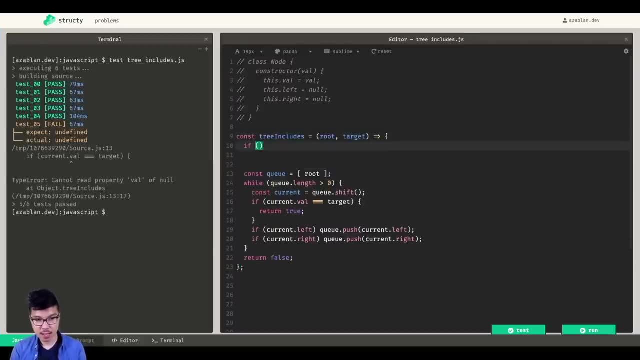 b, b character inside of the empty tree. So return looks like false over here, And so I can just handle that one explicitly. I'll go ahead and check at the top. If my route is no right that's the case, then just return false. So I can't possibly find any target in an empty. 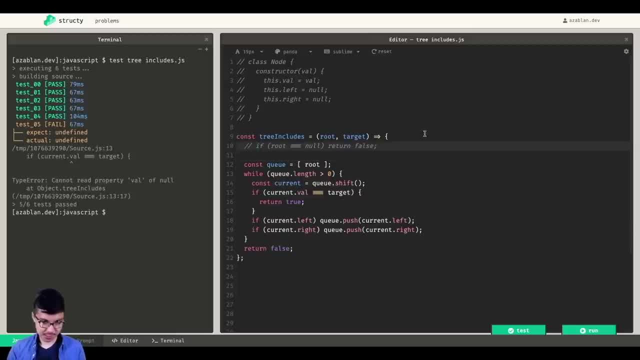 tree Right. The reason our code was failing before is: if root is null, then I initialize my queue with null And when that thing is popping, that null is popped, or rather shifted from the queue in the first iteration, then I check null dot Val, which is an illegal JavaScript. 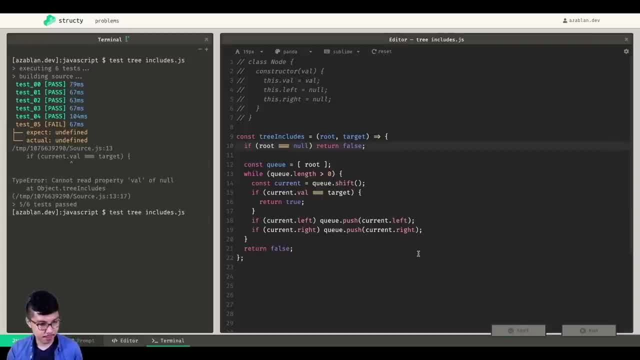 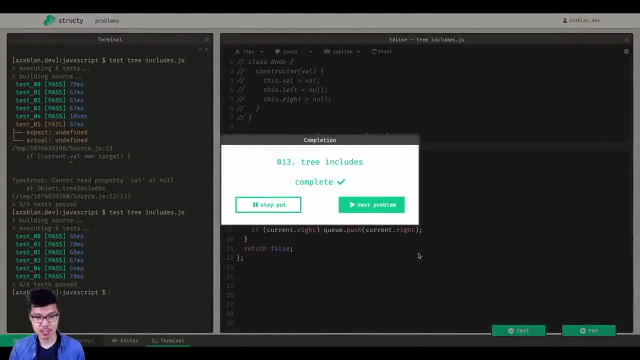 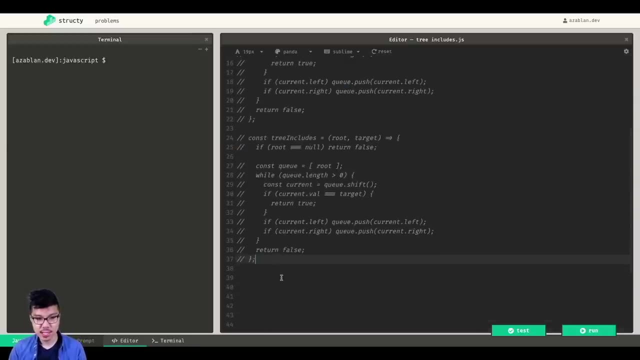 operation. So I'll run all these test cases now. Nice, and there we have our breath. first solution for this tree includes problem. All right, now let's work on the recursive depth. first version of this, And it's actually my personal favorite, because it utilizes a pattern that I think is quite elegant and one I use a lot. 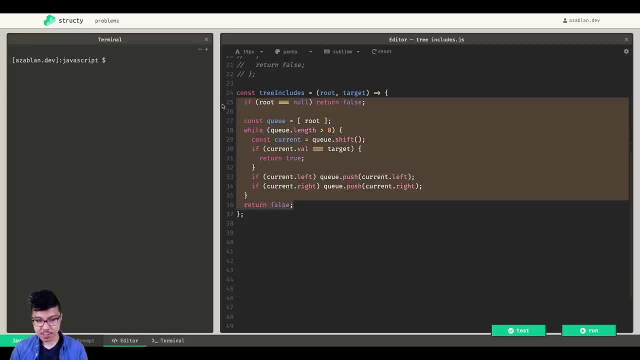 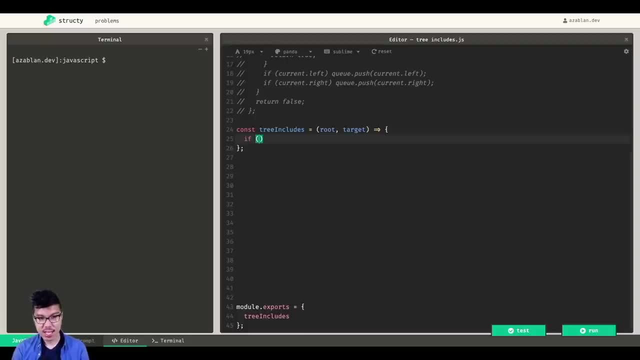 for much more More difficult problems. So, like we said in the approach video, if you haven't watched the approach video, you definitely want to check it out for this recursive version right, What I should do is check, hey, if my route is null, if I have the empty tree, basically. 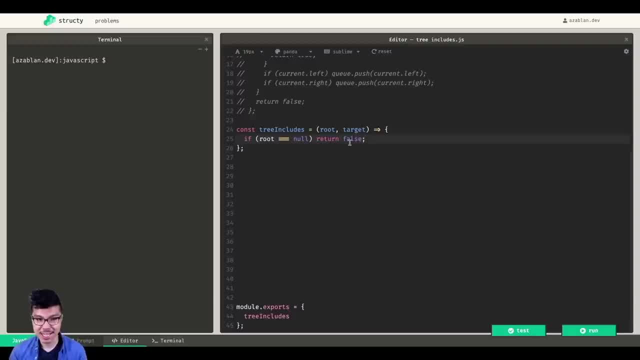 then just return false: right, Because I can't possibly find my target in an empty tree, right, That's just a given. And from there I know I'm going to have the general shape of some just depth. first traversal code, which means you call the same function because it's. 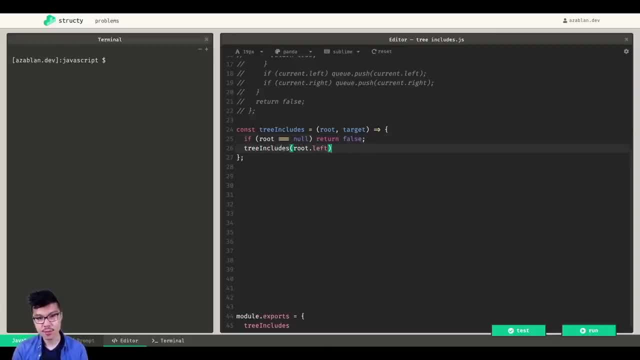 recursive. That's what recursive means. And you pass along your route dot left and a separate call, And then you pass along your route dot left and a separate call, And then you pass along your route dot right, And what I should be sure to do is don't forget to pass in your 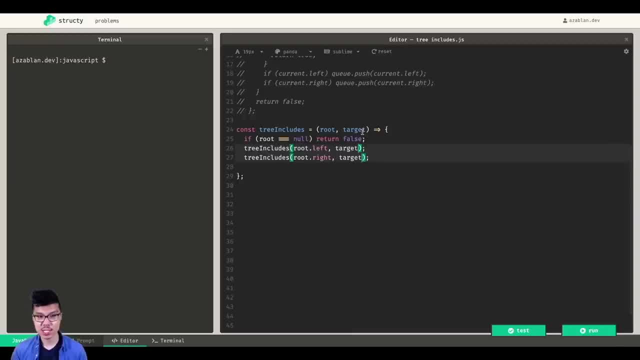 target right. The target that you're looking for never changes And I know that these two, these two calls, are going to give me back Boolean data And I know that the Boolean I get back from like this call would represent whether or not I found the target in that subtree right. So this: 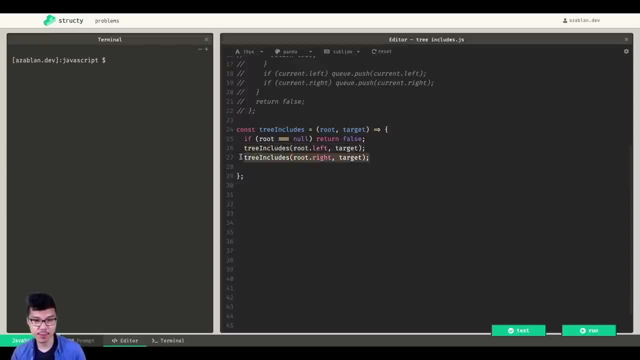 gives me the result of if I found it in the left subtree or the result if I found it in the right subtree, And I can just do the logical, or on both of these right. So if I find it in either subtree, then return true. So I could just write an inline return true over. 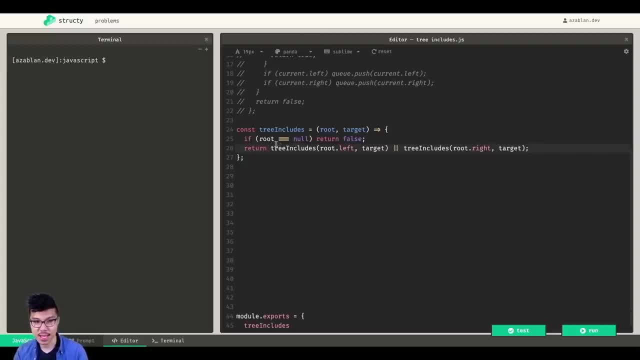 here, right? So let's say it's in my right subtree, then this left hand side evaluates to false And this is true, in which case this entire thing evaluates to true. And let's say, in a bad scenario, let's say it's not found in either subtree, So this evaluates to false, this right. 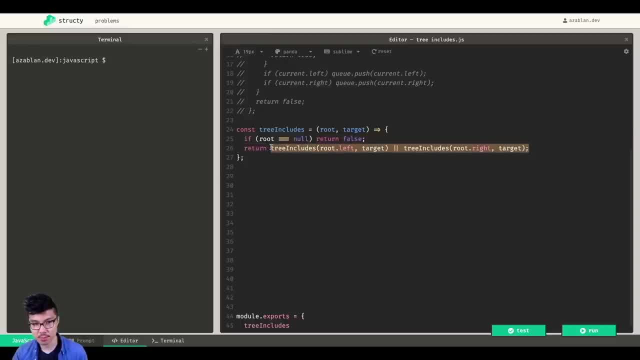 hand side also evaluates to false, false or false gives me false. However, one thing I need to be sure to add is also an additional value. So if I find it in either subtree, then I can return true additional base case After I check if my root is null. what I want to do is then also check. 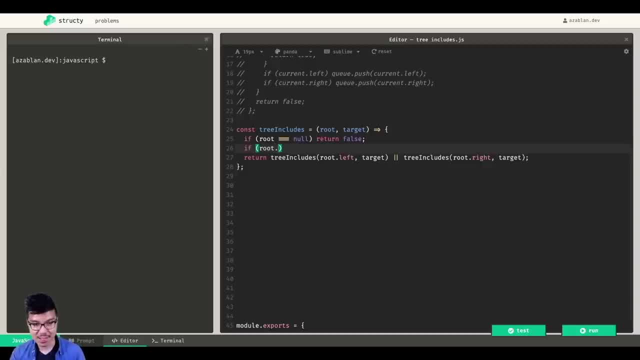 hey, maybe this route I'm currently at, maybe it actually has the target right. So if root vowels equal to the target, then you're also done, except you can return true. Cool, And that was very reminiscent of our approach video. So let's give this a shot. We should be able to pass nice. 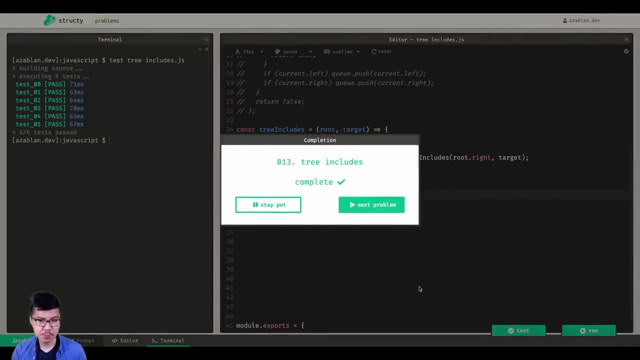 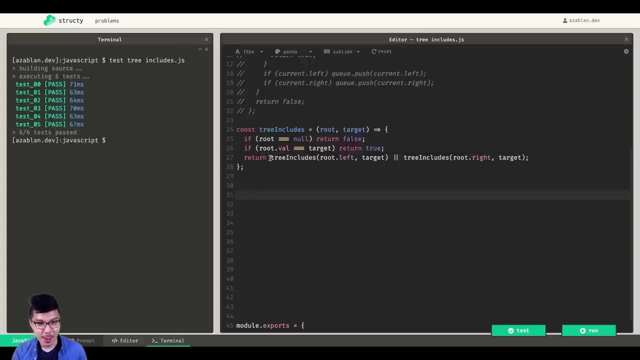 And I love how clean this code is. I will admit, you know it's pretty tricky if you're not a fan of writing recursion, in which case I'll totally convince you into being a fan of recursion. But notice how kind of clean this code is really leverages recursion. One very important thing I want to bring up is 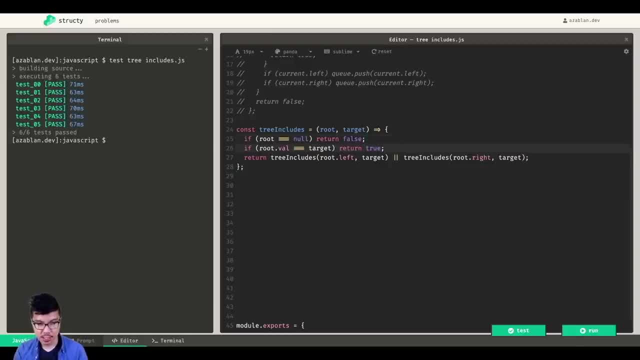 it's really keen that I put this base case on line 26.. After the null check: right? So let's say I flip the order of these. let's say you did this. I believe that would not work out always because it. 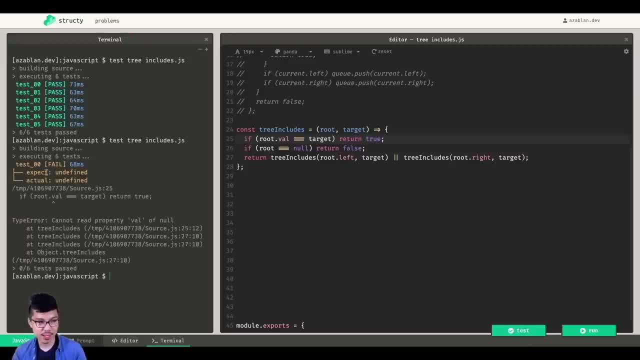 assumes that you even have a route right. So I'm feeling a test 00.. But in general, if you look at this code, let's say that route was null right. You're going to start by checking null dot Val. 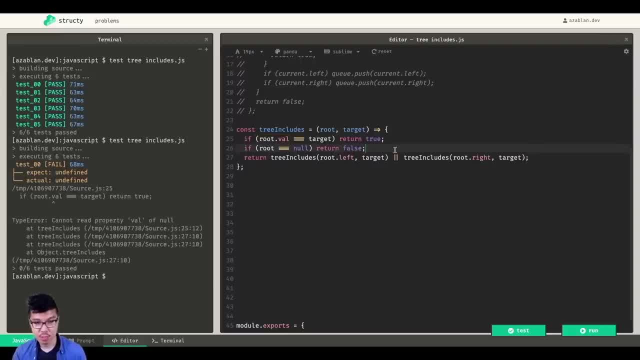 and I'll throw an error right. Can I read property valid: No, So you want to actually always lead with your base case that checks if your route is null. right, Because that should guard really the entirety of our code. So this is actually the code you want over here, All right. 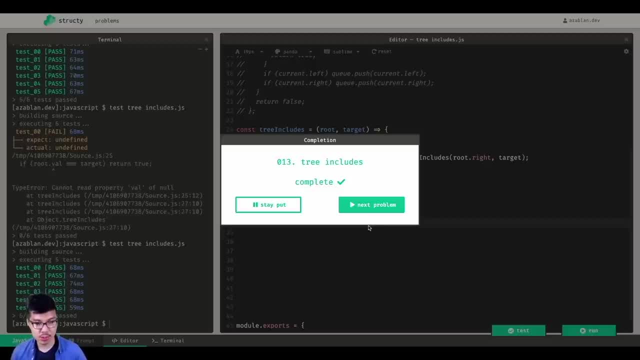 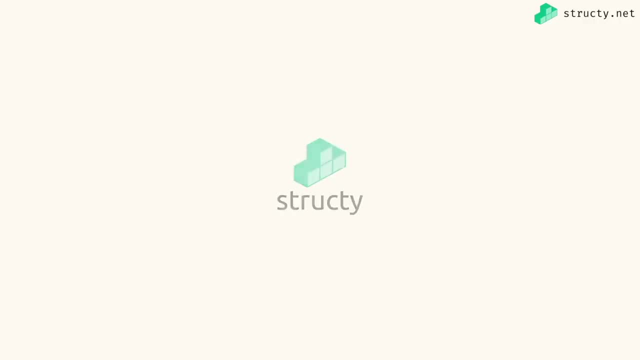 programmers, So that's all I got, for this tree includes a solution. I want you to practice both versions and I'll catch you in the next one. Hey, programmers, Alvin, here Right now I want to go over the approach for this tree sum problem. 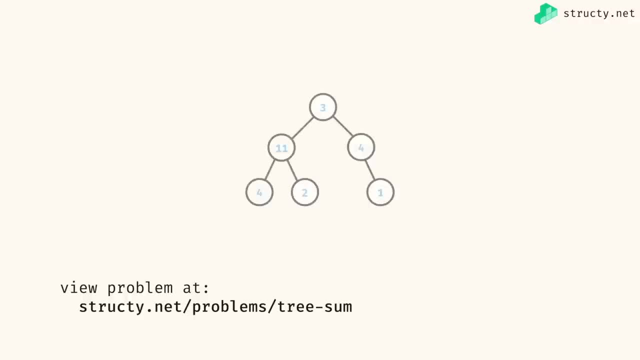 And so, in this problem, I want to take in a binary tree, just like we've been doing as of late, This time the values within the nodes of this binary tree. they're going to be numbers, right. What I want you to do is compute the total sum of all the values in this tree. So, for this example, 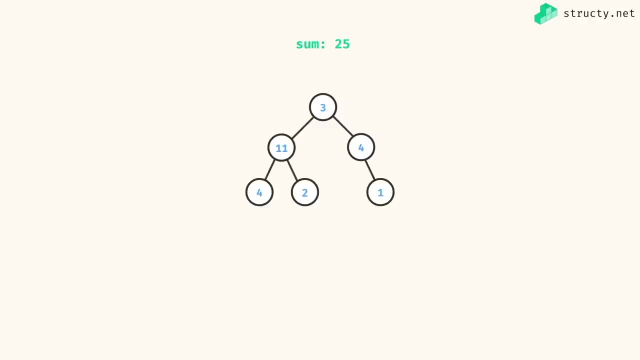 we should end up with 25.. And so hopefully you're kind of gathering how to attack this problem, especially given you know the algorithms I've been showing you as of late. So if you've been studying our problems in order, hopefully you know a straightforward solution to solve this one. 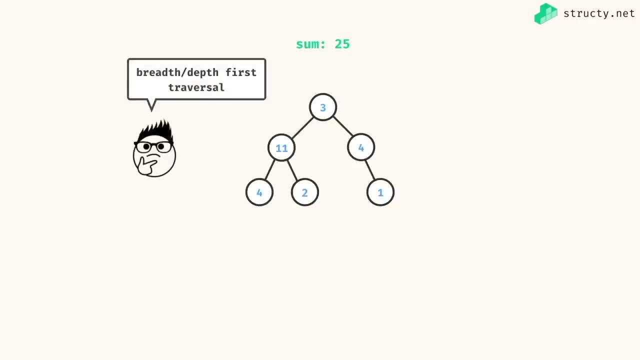 we could of course just use any type of traversal algorithm. So we can use either a breadth first or a depth first traversal, And we can just add all these values into a running sum. then, of course, we'd probably initialize that sum to zero, right? So the iterative? 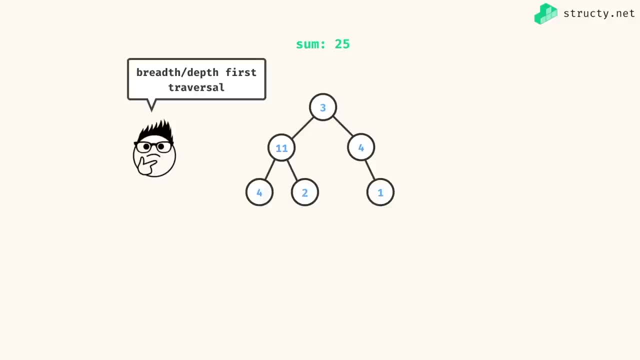 breadth first or depth first solution I think is very straightforward, right, And I'm not going to really a step through that approach with you over here. I think you have that one down pat, especially if you've done the previous two problems. But what I will show you here is: 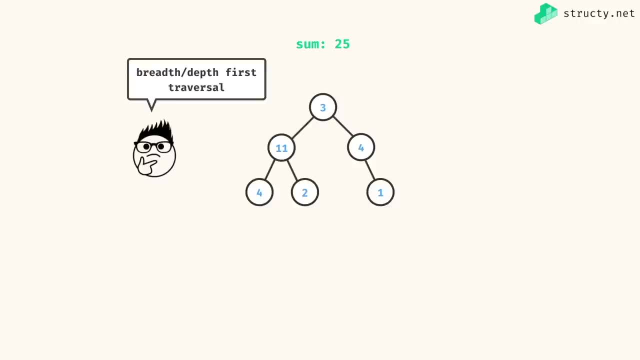 actually how to solve this one recursively, which would be a type of depth first traversal, because we know that, hey, depth first traversal relies on a stack And if you do something recursive, it is utilizing the underlying call stack. So I will get a similar type of ordering. 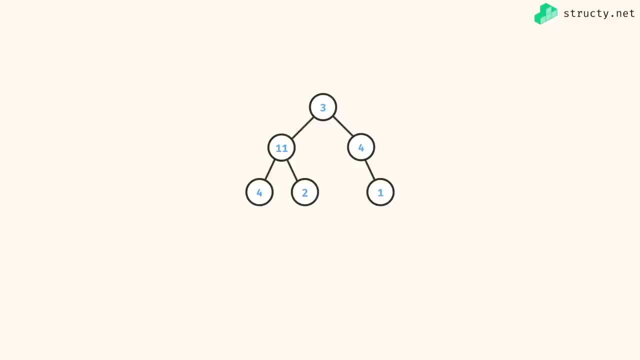 And so when we trace through a, this type of solution is recursive solution for this tree sum problem. what we're going to do is try to be very explicit. I think this is really helpful, especially if you struggle with recursion right. So, given this binary tree, I know that for. 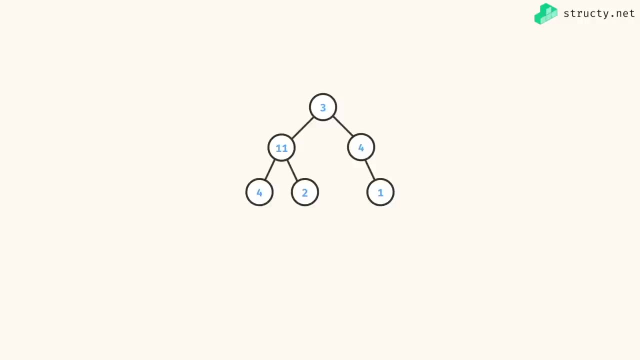 particular nodes of my tree, like the four node, it does not have a left child Right, And I know, like, programmatically, what that means is, like that nodes dot left pointer points to like null right. it's a null pointer And so I'm just going to draw that explicitly, sort of like. 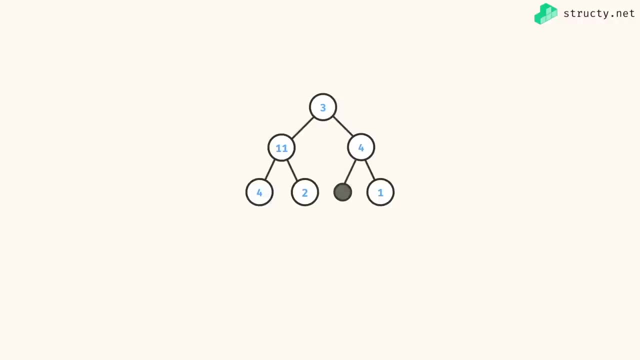 this Again. that'll just help us really understand how our recursive code performs on this type of input. And so if I know that I can put like a null node to the left of four, then it could be the case that other nodes like the leaves of two and one- they also have both left and right children. 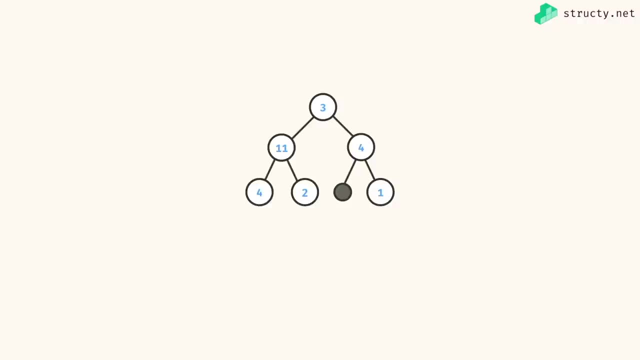 that are also null. So if I drew all of my null pointers explicitly, it would look something like this: Cool, And this is a really something that helped me really get comfortable with recursive problems, especially those on binary trees, And what we're doing now is we know that. 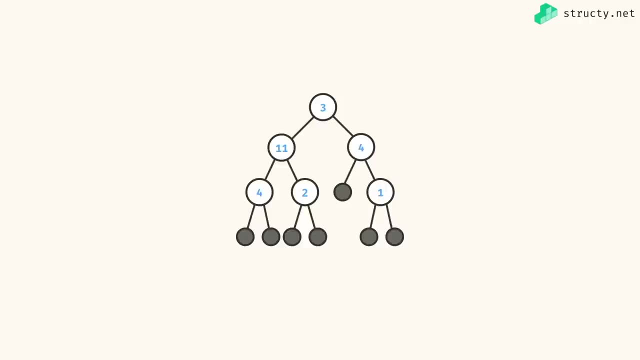 when it comes to solving any problem recursively. it's about writing a base case that is like the simplest version of our input. And here I'm going to argue that our base case needs to be about the null node. right, The null node basically represents no node at all. 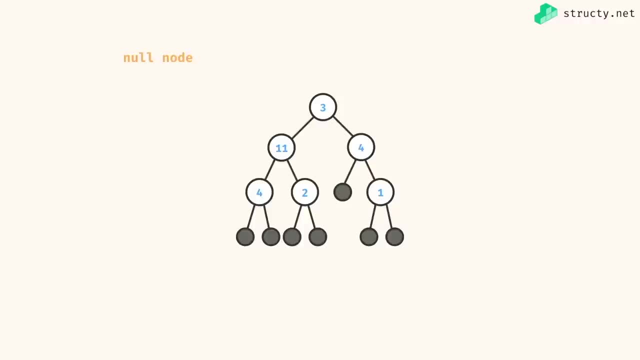 represents the empty tree in a sense. In other words, if someone asked me to calculate the sum of a null node or the sum of an empty tree, then to me that some would just be zero to write elegant recursive code to try to think about your base case as a problem in itself, right? So if 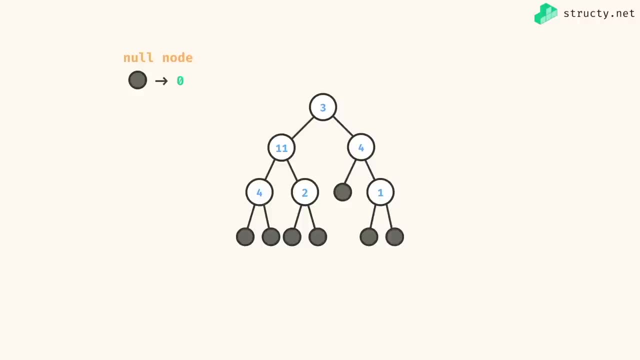 someone gave me an empty tree. that is a null node. I would return the total sum of zero, And what that means is I know that all of these null nodes, they would return zero as their computed sums. Nice, And then from there, how can I use this information to actually build up? 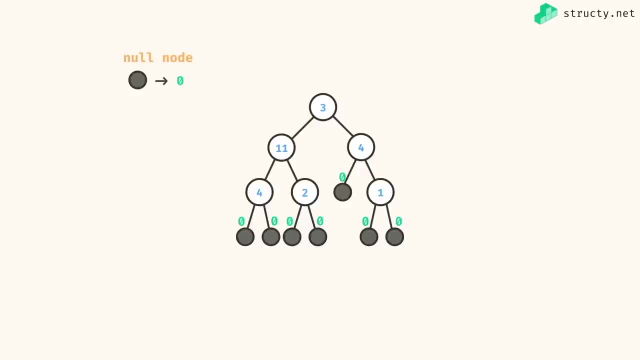 my main solution, Right? So let's go ahead and target this four node to the left, And what I have to do is figure out: hey, what is this sub trees, total sum? and I can compute that given the values to the left and right. In other words, if I return those two null values returns. 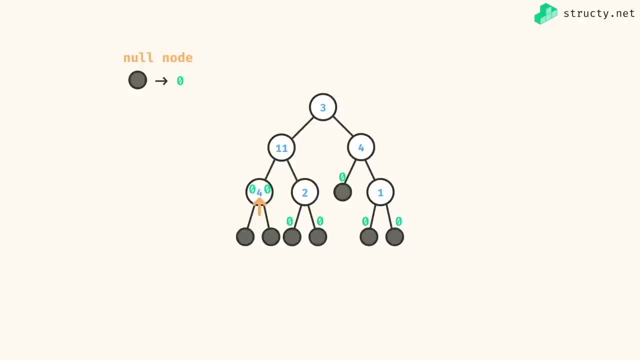 so they're both zero. now I just have to do zero plus four plus zero, which just equates to four, right, And that is actually correct in itself, right? So a green number above a node represents the total sum of that sub tree, And so it is a case that, hey, the total sum of that. 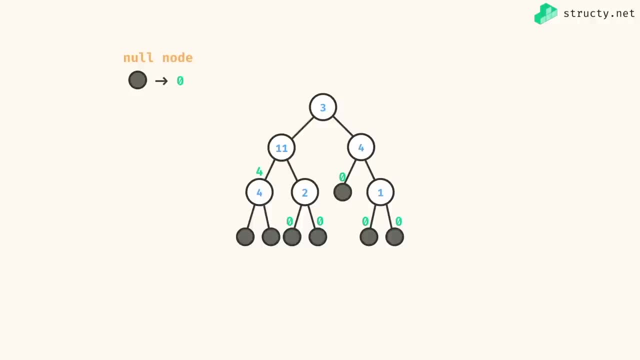 four node is just four, And I will do something similar for this node over here right, When these base cases return to their caller or return to their parent. I just have to add my left and right child together along with myself. So zero plus two. 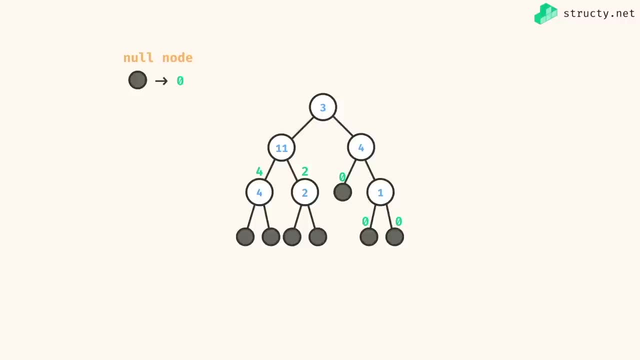 plus zero gives me two, And I'll do that same thing for this note 11 over here. And now things get interesting right. To calculate the total sum rooted at this 11 subtree, I would just return these values to the top, And now I do four plus 11 plus two, which gives me an answer of 17.. 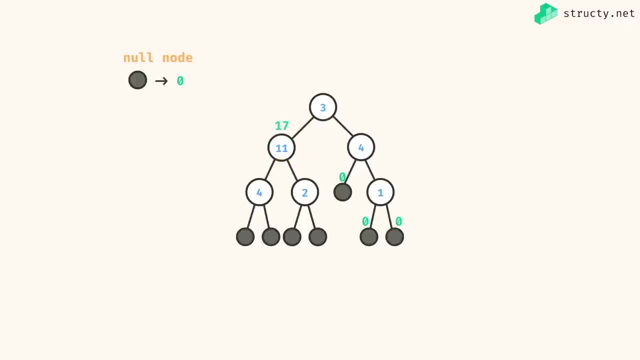 And if you do a quick spot check right, this 17 does represent the total sum, just in this subtree right, And we'll carry on over at this one node. we know that this is going to return just a value of one, And now at this four node, I can compute its total sum. 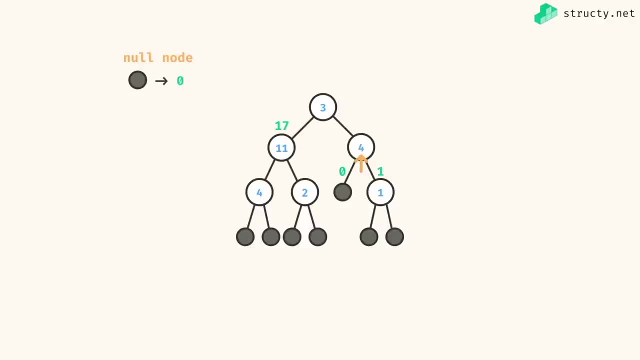 and recall that this four node had a left child of zero right because it had a null node. And so when I compute this sum, I get five, which is perfect. And finally, at the main root now, I bring up these two values and I compute 17 plus three plus five, and 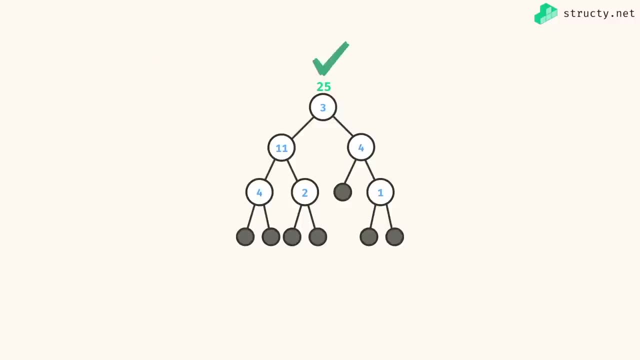 that gives me a final answer of 25, which is indeed the correct answer, right? So that's how we should really think about our recursive algorithms for our binary trees, right? I kind of draw it out. I think about the base case, which is typically not always, but typically. 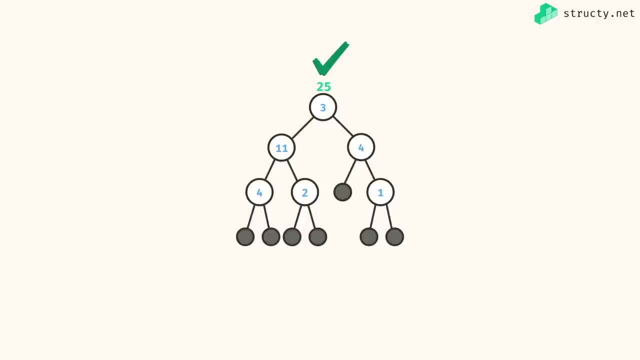 about the null node, And then from there I figure out how a parent can compute its results, given its children's answers. Alright, so if we take a look at the complexity of this, it's pretty straightforward. We'll go ahead and define n as the number of nodes in our input tree, in which case 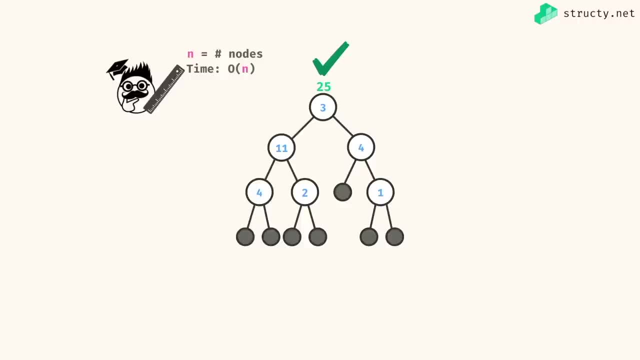 I can see that my type complexity is just O of n. right, We know that we're going to make a recursive call just for every node of the tree And we're not going to call duplicate nodes. right, we're going to have just one call for every single node And within any 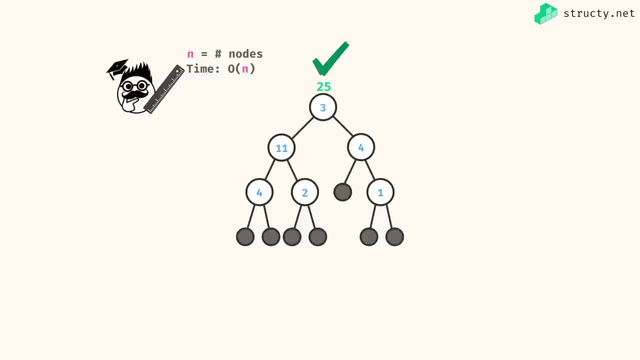 single node. we're just going to do some simple arithmetic right. we just add roughly three numbers together. So it's not like we're going to have like a loop inside of our calls at all. And in a similar way we'll say: the space complexity is O of n, just because we have 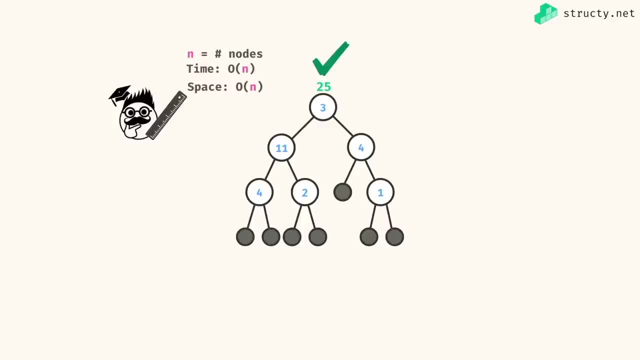 that implicit a call stack space, because we are going to solve this one recursively, And so we're solving this one in O of n time and space, which would be actually a maximum efficient solution for this problem. And so with that, I think, let's head over to the walkthrough. 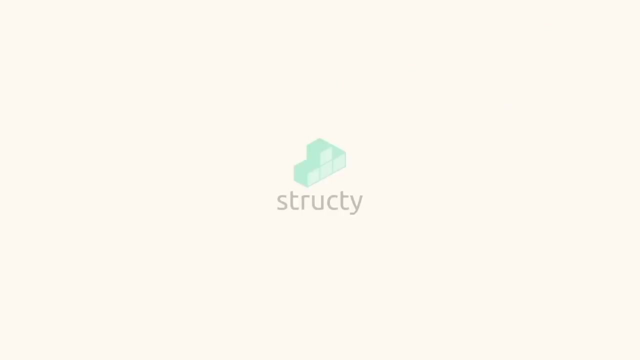 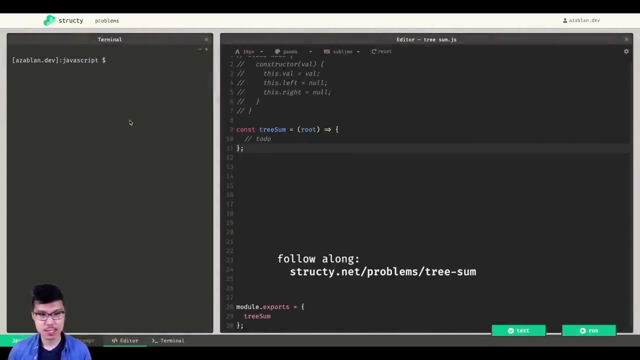 video and I'll show you how to code this one up. Hey programmers, Alvin here, Right now I want to walk through the JavaScript solution for this tree. some problem, And I think this time around I'll jump right into the recursive. 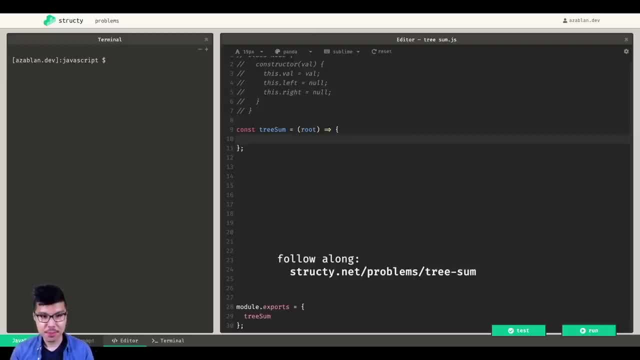 version, right? So we'll start recursively And we'll begin with our base case, right? My base case is always about the simplest version of the input, where I just know the answer without needing any additional calculations. right, I know that the simplest tree here. 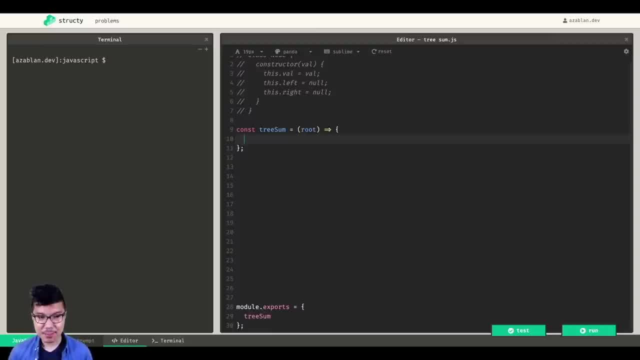 that I could be given is going to be the empty tree. right, But have the empty tree. That means my root is null. And if your root is null when you have the empty tree, what is the sum of the empty tree? well, kind of inherently, it's just zero. So that'll be my base case, Nice. 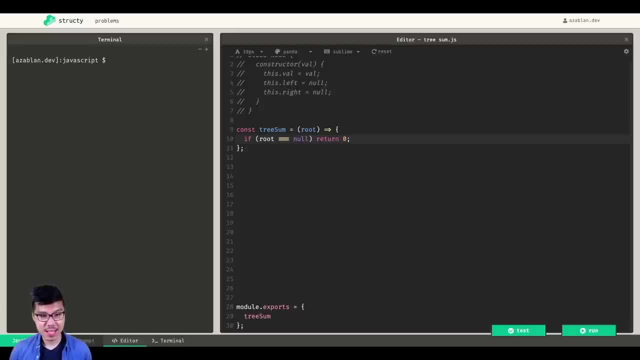 Then from there I'll think about how I can compute my answer, given my children results. So I need to find the results of the sum of my left subtree and also the sum of my right subtree. So just call recursively, So tree sum of root left as well as tree sum of root right, Cool. 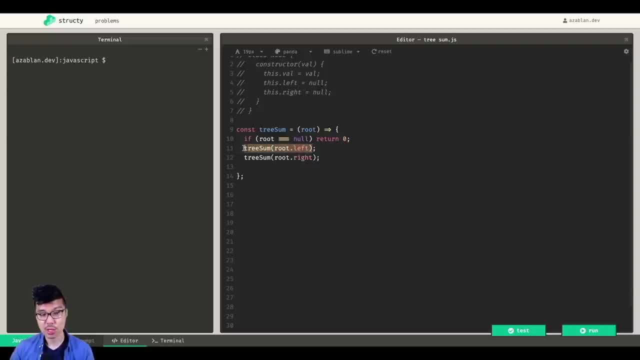 And I know that these two calls they return numbers right, representing the sum of my left subtree and the sum of my right subtree. as the parent, that is, as the root, how can I find my total sum? Well, it just is myself, So root dot value plus everything in my left subtree, plus. 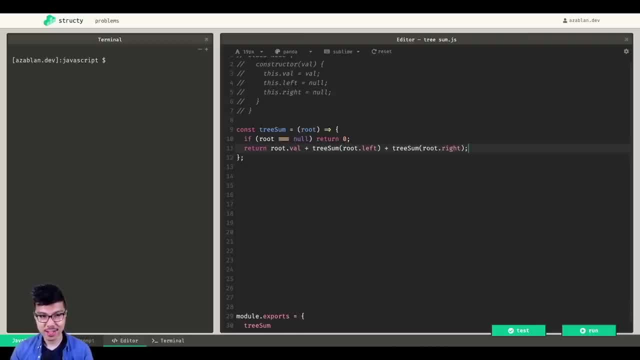 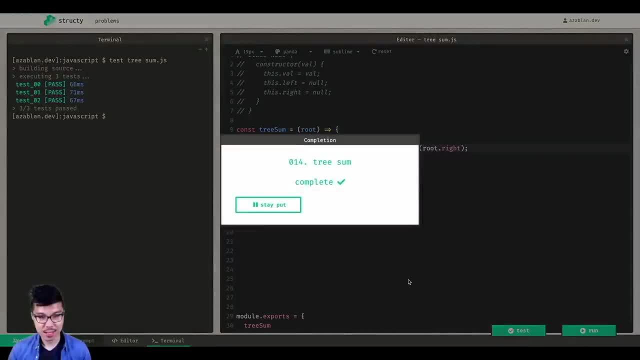 everything in my right subtree, Right, And we'll go ahead and just test this out the gate. But this is nothing fancy, a really elegant code. So look at the test cases here. we do have some diverse output, So this code does work. 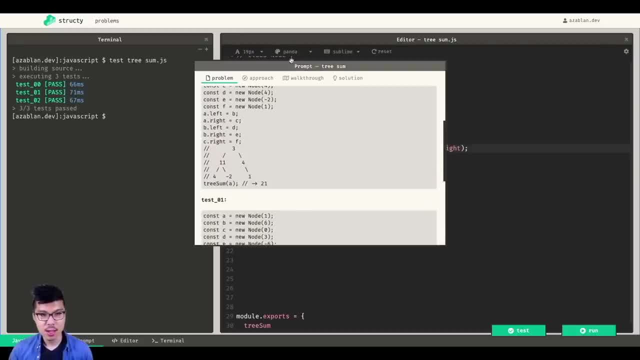 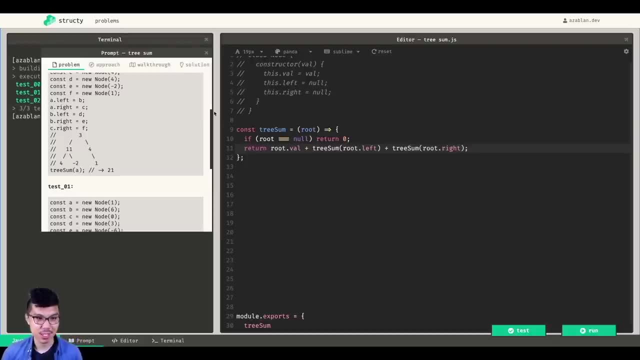 on trees of all different shapes and sizes. Something that helps me, you know, really believe the magic of recursion- is to just analyze the assumptions here. right? So let's say that I'm stepping through tree sum and my root is this three over here. right, So I check the base case. 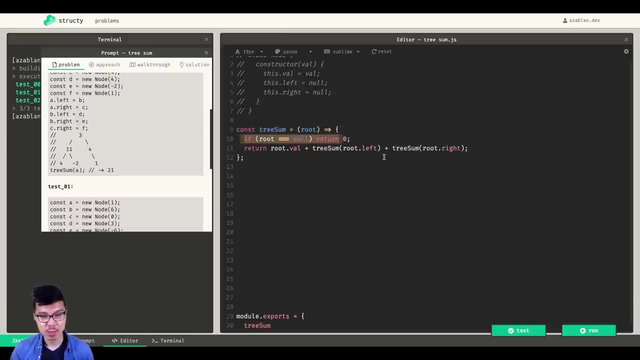 is this three node? No, it's not. So I must make the recursive call right And I know that when I break down this code recursively I know what route that Val is going to be like three. So I'm kind of corresponding. 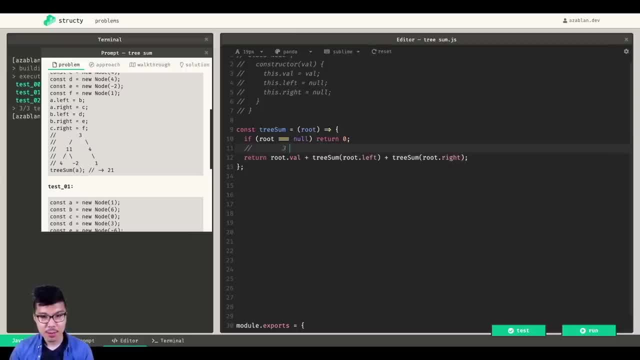 this comment with the thing below right. And then when I make the recursive call on tree sum root dot left, that means I'm asking for the total sum of this subtree starting at 11.. So I'm looking at the 11 for negative two subtree right If I take the total sum of just that left subtree. 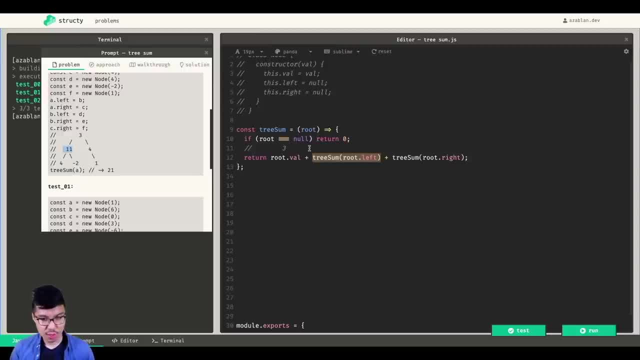 it looks like it's going to be just 13.. So now I'm saying plus 13.. Over here, right. If I do the same thing on the right subtree- I know that this call is for this four node right and all of its children that should just magically return. 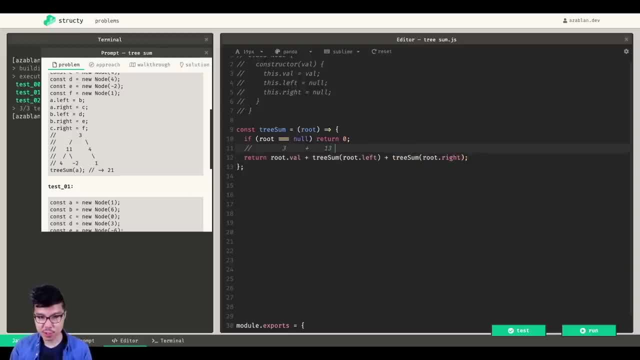 by the power of recursion, that should return five, right? I'm going to assume that that recursive call just works, So you have the five right. If I take the total sum of these, three plus 1316, 16 plus five is 21.. That would give me the correct answer, right, So to have. 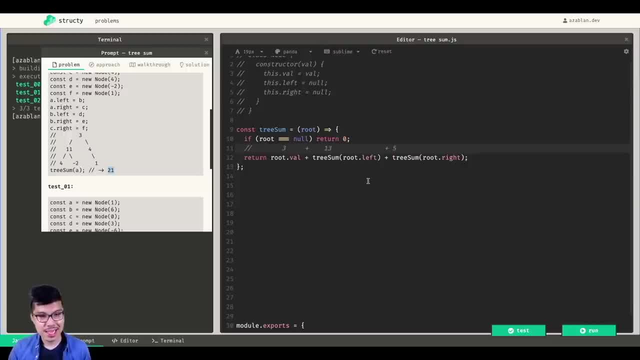 some confidence in my recursive code. I just write the code and then I assume you know I'm going to correct this from my recursive calls and I figure out how to can take those no sub values from my children, combine it with my own value And that should be my final answer. So here is the 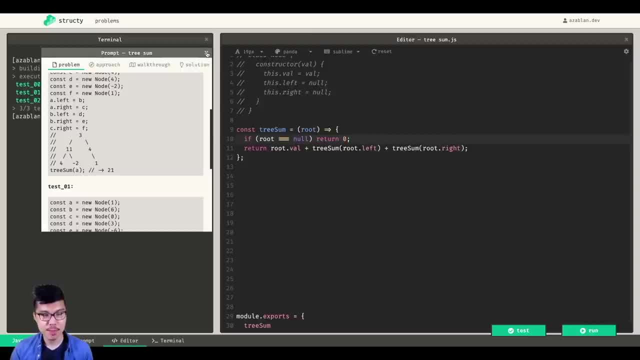 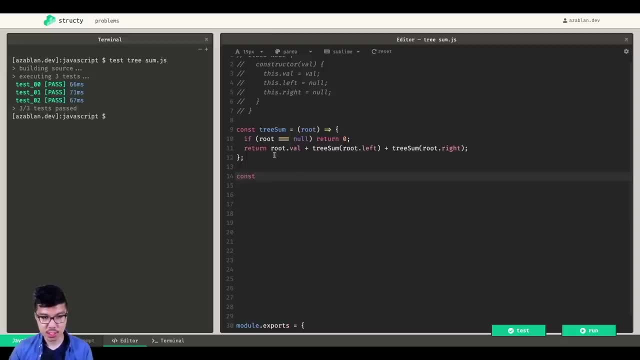 recursive version of this solution, which would be some sort of a depth first traversal, technically, because it's recursive And if you'd like, I can also show you the iterative version. So let's just do that And I always practice usually my problems doing both the recursive as well as the version. 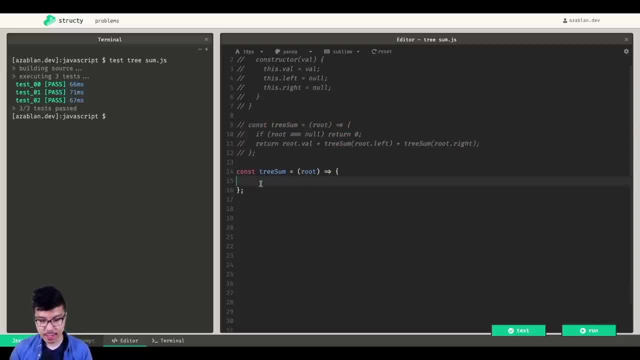 it's reasonable and it is really reasonable here. Hopefully you're familiar with our breadth first code by now, right? So I'm just gonna start by checking: hey, if you're given some root that is already null, then that's kind of just an edge case. I'll just go ahead and 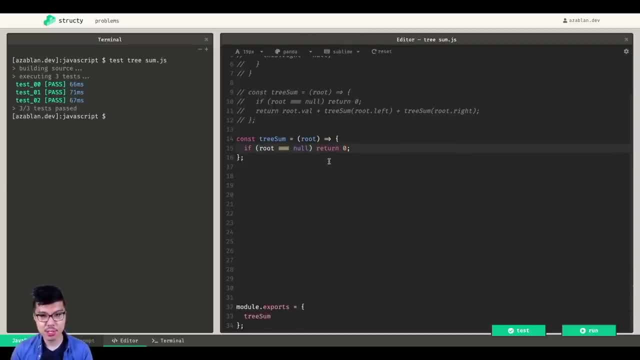 return zero, right, Because the sum of that empty subtree, or that empty tree rather, is just zero. then I can begin my main code. So while my queue is not empty, so I'll start with a queue who begins with the root root And I want to loop while my queue is not empty. So while q dot length. 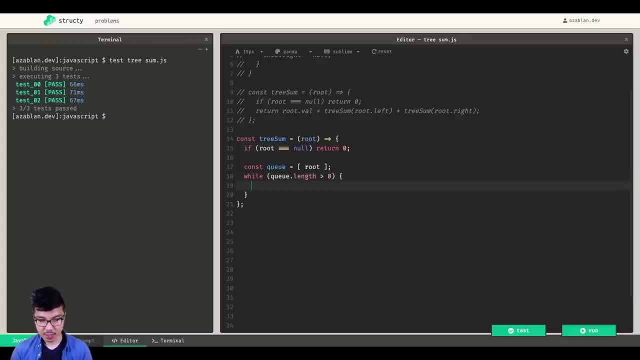 is bigger than zero. I'll begin a single iteration of my while loop by just shifting out the front of my queue. So in JavaScript for me that's q dot shift that removes the front element and also returns it to me. So I'll save it in current And then from there, now that I have this current. 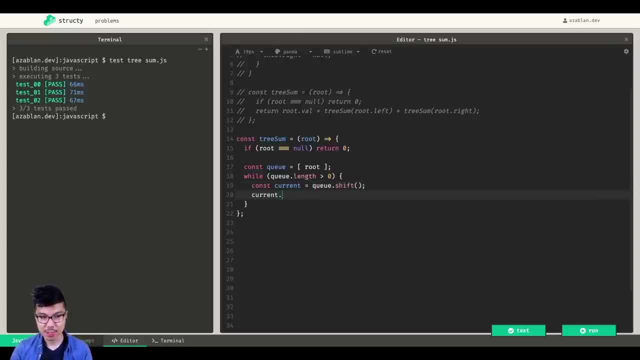 I know that that contains the value that I actually care about. So what I would do is go ahead and try to get rid of the front element And then from there, now that I have this current, I know that that contains the value that I actually care about. So what I would do is go ahead and try. 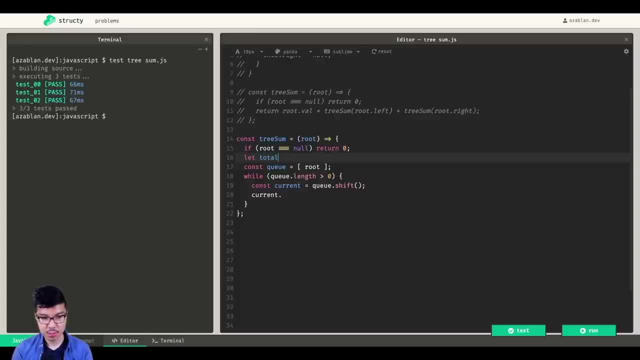 some running some. so I'll say: let some remember. say let total sum equals zero, And as I remove something from the front of the queue I'll take its value and add it to my total sum, So that will accumulate all of the values right into a sum. Then from there I just need. 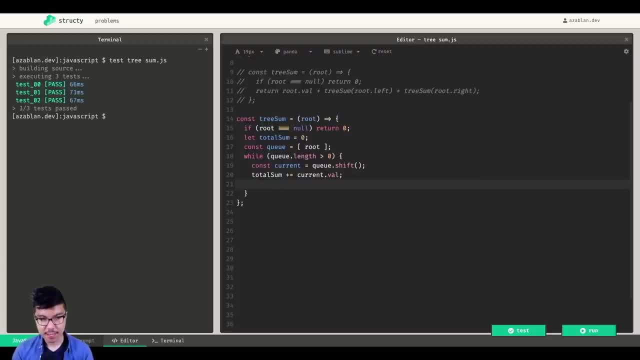 to add my classic logic of checking for my children, right, if they exist. So if I have a left, so if current dot left is not equal to null, then what I'll do is add that left child into my queue. So q dot push my current dot left. Again, make sure you're following your Q rules, right? So 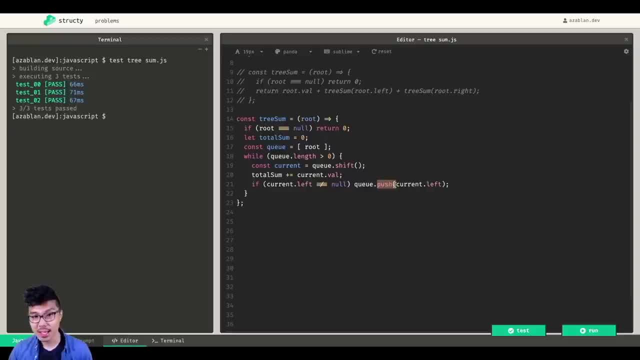 shift removes from the front, push adds to the back. it's really important that my shift and my push or my add and remove methods work on opposite sides of my queue. Otherwise it's not a key right. So that looks good to go And I'll write something symmetric for the right hand side over here. 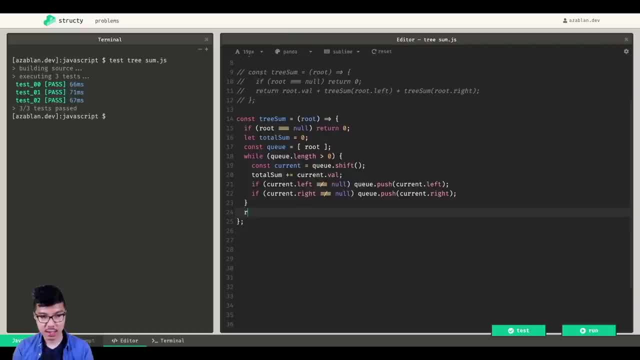 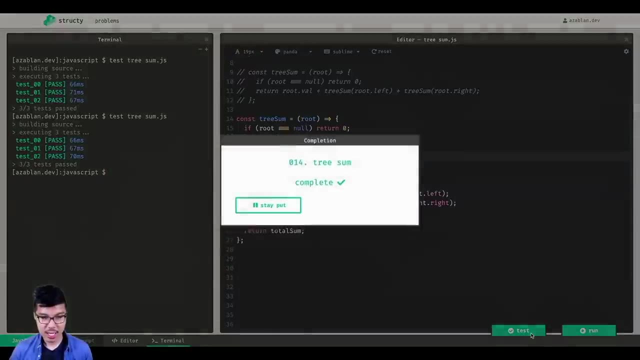 By the end of my function. I'll just go ahead and return my total sum: Nice. So this would be my go to iterative version. Of course it's technically a breadth first, and we'll give that a test. Nice, And here we have that solution. So one. 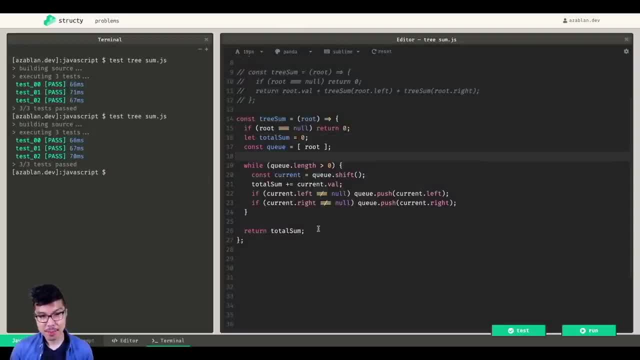 thing to note. I think it's pretty important to be consistent in how you implement these algorithms, at least where possible. So you'll notice that I always am a fan of writing my like processing logic for a node care I consider like the processing logic where I add the 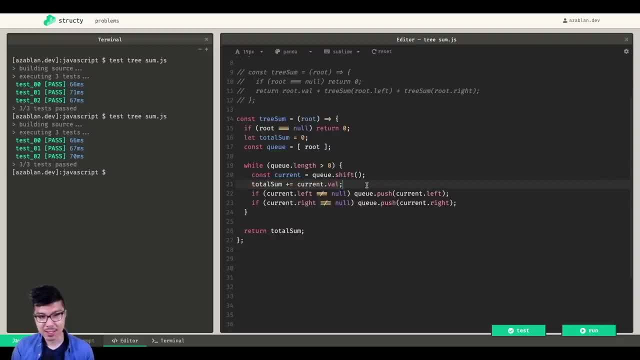 value of my current node into my total sum. I do that processing logic typically when a node leaves the queue and not when the node is added to the queue and just ends up being less repetitive. that way, For example, I've seen some people write code like this: 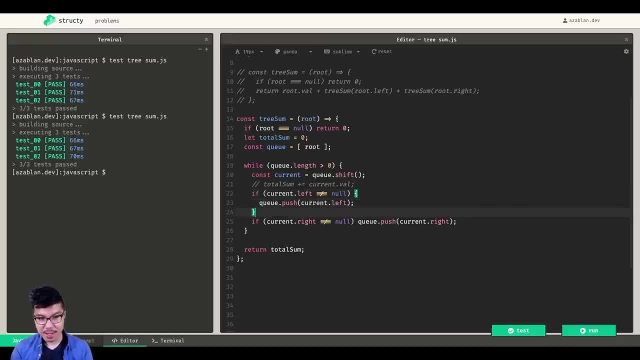 or it's like: Alright. well, you know, I guess, since I'm adding my left child into my queue, that means it exists. So not only will I push it, but I'll add it. So I'll do, I don't know. total sum plus equals current dot. left dot. 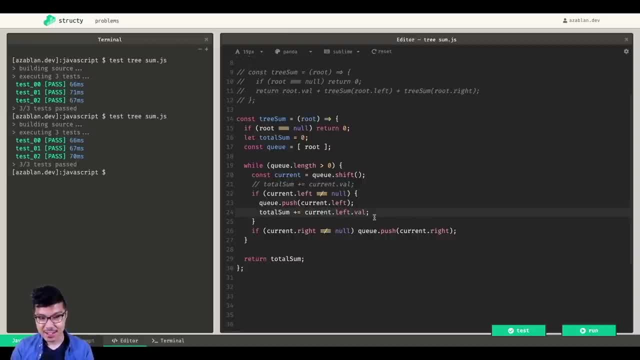 bell right, some kind of adding the child's value as soon as it's added to the queue, And you can write something symmetric for the right hand side. You can see that because of this I kind of have to double up all of my code, which does not make it super clean. 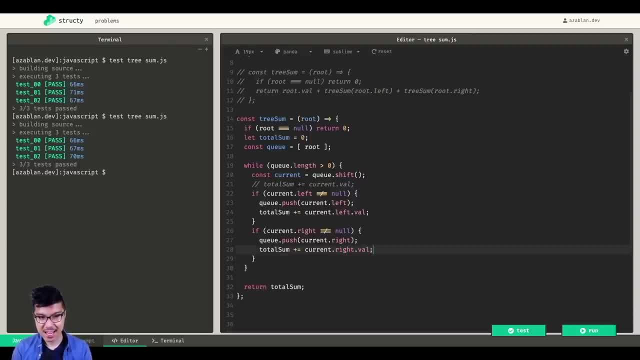 And I think something that is even worse than that is. well now, you actually never added your root value into your, your total sum, So you would have to begin your total sum as root dot Val, And at this point I'm like I kind of just hate this code. right, So you can run this. this would probably work. 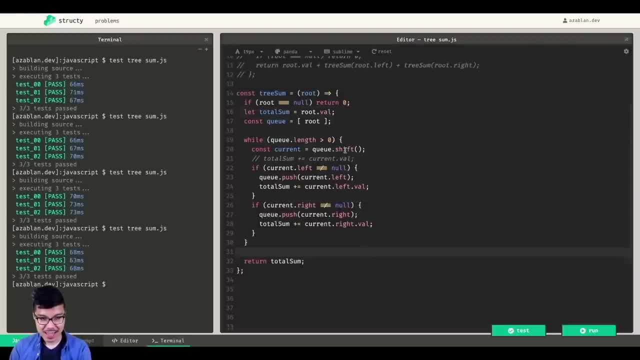 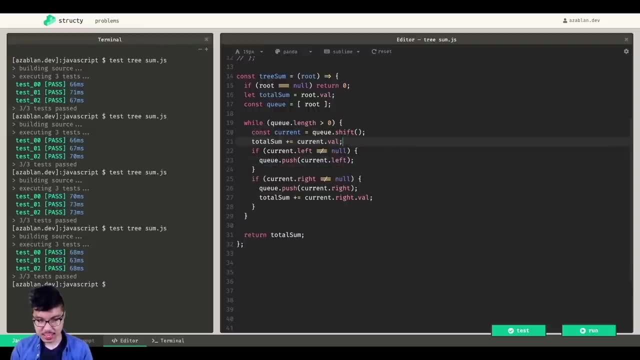 So this code totally works, but it's not what I think is the best design for this pattern, So I'd rather write it like this: right, Consume your values when they leave your queue, because you know eventually everything's gonna leave, right. So I'll prefer it at least like this: Cool, So before. 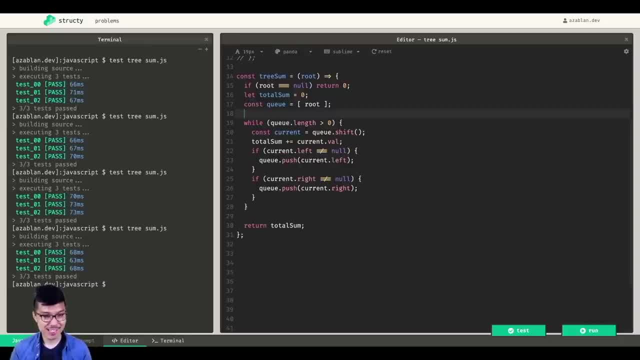 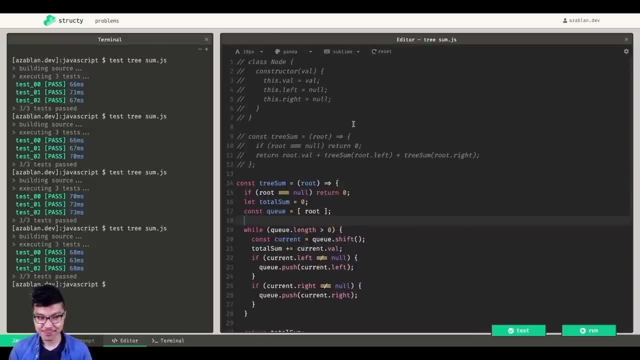 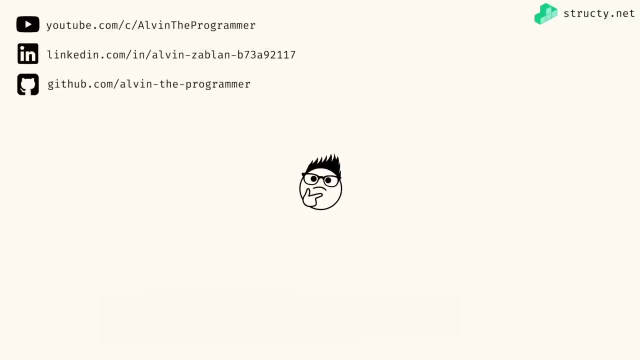 you go on to the next problem. recommend you practice both versions of this problem. So do it recursively, do it iteratively, have them both down pat, because we're going to increase the difficulty right now. Hey, programmers, Alvin here right now I want to go over the approach for this tree. 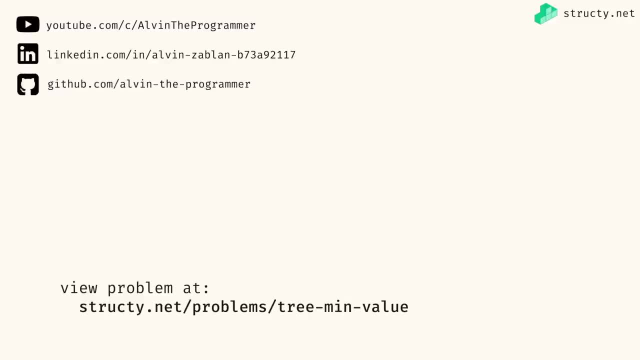 min value problem. So, just like we've been doing as of late, we're going to have to take in a binary tree as input into our function And we want to do is figure out what the smallest value within the tree is, that is, we want to find the minimum. 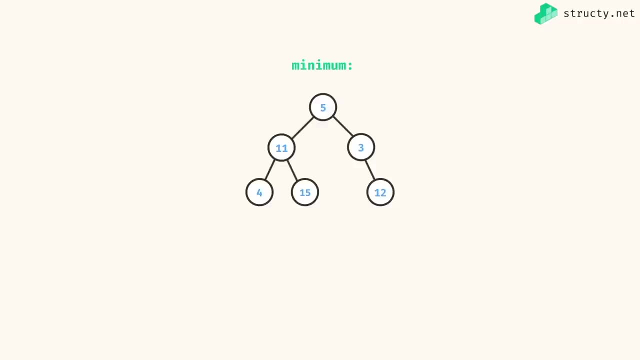 value. So we can totally assume that the tree is going to be non empty right. And so, given that information, looking at this particular tree example, it's pretty plain for us to see that the smallest number in the tree is just this three right. so our function just. 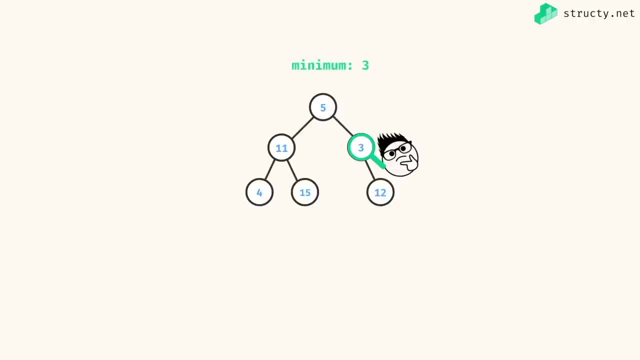 needs to return the number three, And so it's plain to see that the answer is three. And then we're looking at that value in here. I would approximate this as three, but we have to list this as three. But how can we come up with an algorithm to do this for us? 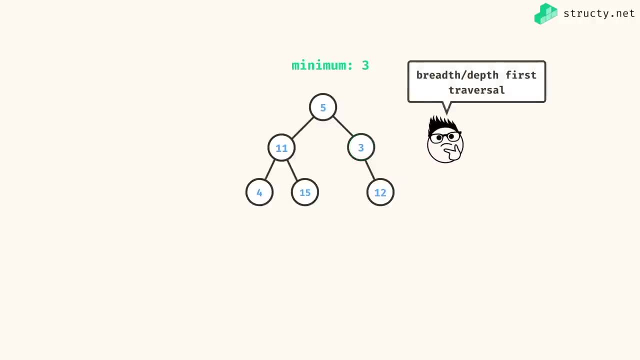 Well, we should look to our tools in our binary tree toolbox, And that would mainly just be either a breadth first or a depth first traversal. One obvious way to solve this one is to use either a depth first or breadth first iterative piece of code that does a traversal right. 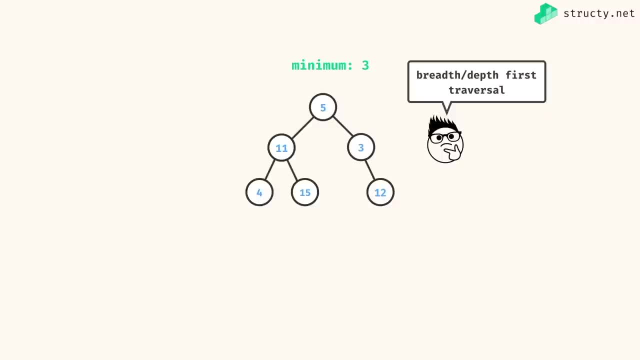 and travels through the tree. then you just need to maintain some outer variable to track the current minimum And whenever you hit a node that is smaller than your current minimum, then you replace should have the true minimum. So the iterative version, I think, is pretty straightforward. 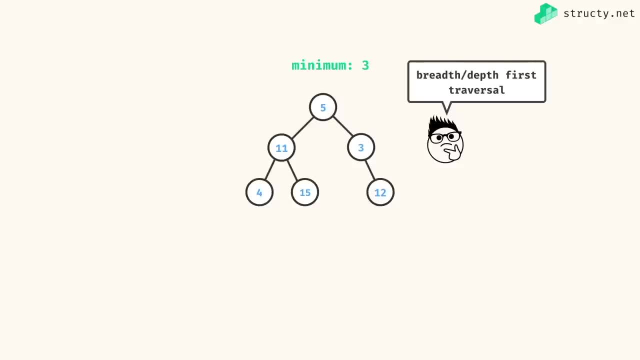 And I'll be sure to walk through that when we get to the code walkthrough. But for now, in terms of our approach, visual, I think we'll step through this one recursively, right, because it ends up being pretty succinct code, And so let's take a look at this tree And 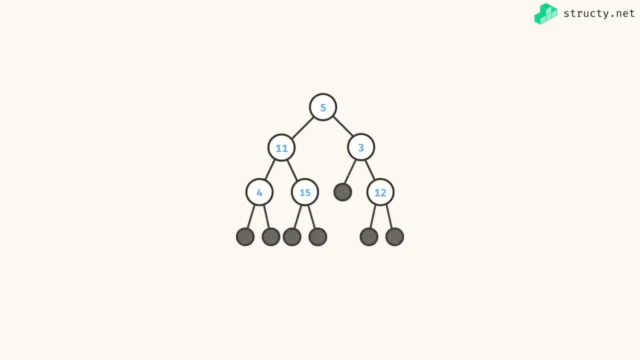 let's pretend that we filled in all of the null pointers like usual, right. So these dark nodes over here represent nodes that don't exist, meaning that they're null right. So, for example, if I look at the three node, its left child is no, but it's right child. 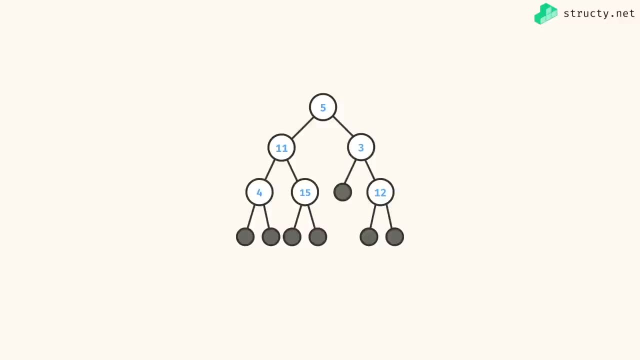 is 12. And that's going to be very useful for us to at least visualize, because I should make a base case about those null nodes, right. So I know, in the long run, what I want to do is figure out what the smallest value within the tree is, And so a great default value. 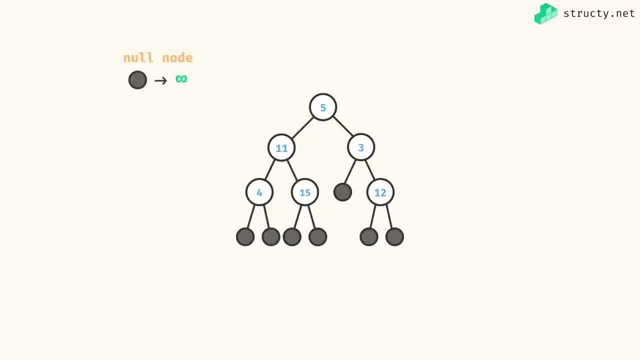 for our null nodes would be to return infinity, And here's the reasoning why I know that I should not really consider any of the actual null nodes, And so if I have them return positive infinity, I know that positive infinity is definitely not going to be the minimum compared. 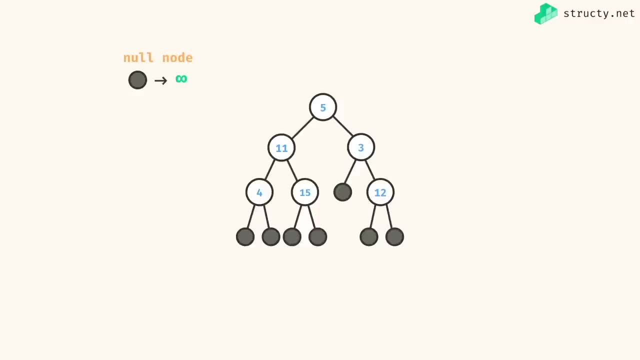 to any numbers that are actually within the tree. So what we'll start to do is just fill in all of these infinite values. In other words, every time we call upon a null node or a null pointer, we're going to return infinity. So I'd fill all of these in Now using those. 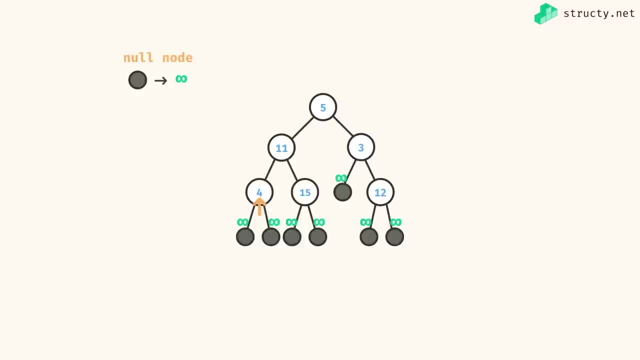 infinities as our basis, we can actually construct our return values. So, looking at this four node to the left, what I have to do is consider both of its children that it received right, and also the value within the current node, And so what I do is I check, all right, compared. 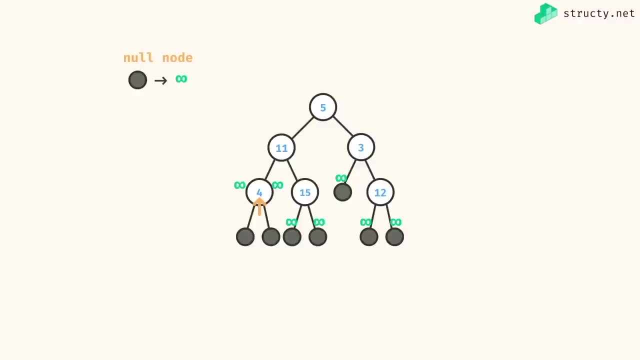 between infinity for an infinity, what's the smallest value among them? Well, I know positive infinity is a very large number, So really the smallest number here should be four, And so this call should return for this node, should return for similar story for this 15 node. 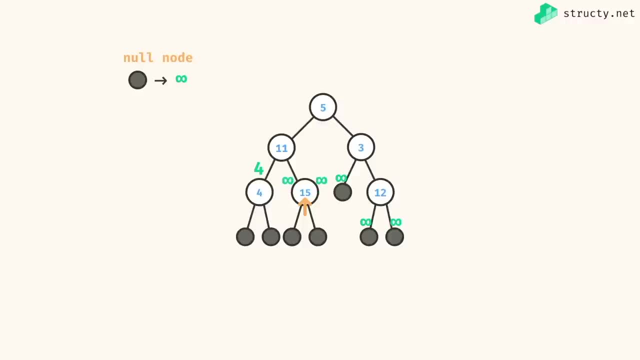 Once I have my left and right return values ready, I do a comparison with those values against myself, right? So I check what's the minimum among infinity, 15, and infinity, the minimum is 15.. And things get interesting now that. 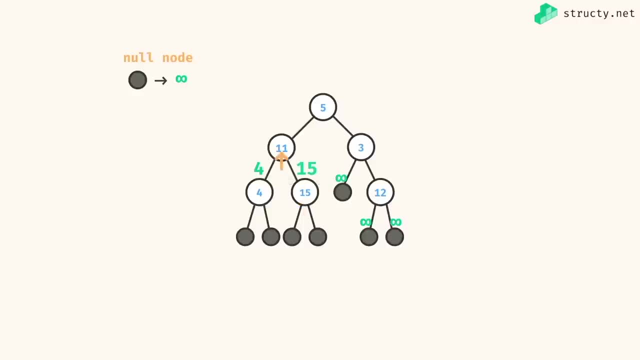 we're at evaluating this 11 node right Now. I have some actual numbers And so I do this comparison right. I compare my left subtree value, which is four, and my right subtree value, which is 15.. And also myself, which is 11.. So, among 411 and 15, what's the smallest? 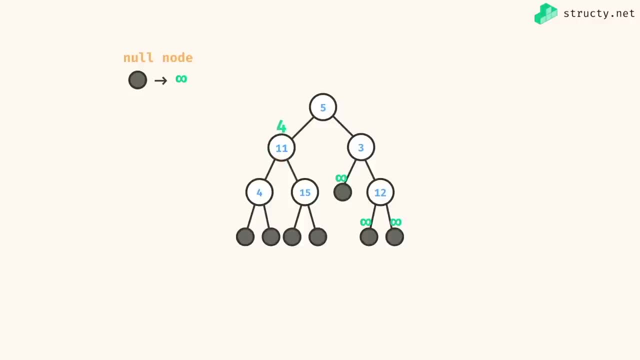 number. Well, that would just be the four right. So this node should return for- And if I do a quick spot check, this makes some sense because I have this answer for above the 11 node. So that's telling me. 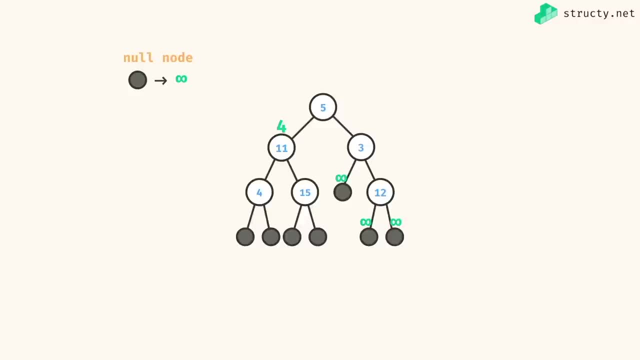 that within that subtree, rooted at 11,, the smallest value is four, which is totally correct. Now we'll just go ahead and evaluate the rest of this tree. Looking at this 12.. Over here, I know I can't evaluate the three because I need a value on the right hand side, right. 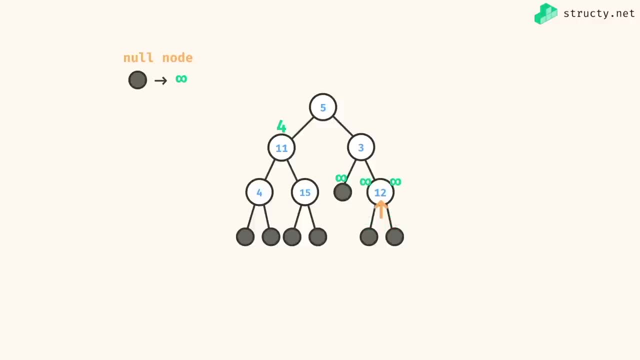 So I must evaluate this 12.. And I just do the comparison right. What's the minimum among infinity 12? And infinity 12?? What's the minimum among infinity 12 and infinity 12?? Well, that's just definitely 12.. Finally, at this three node, I take the minimum of. 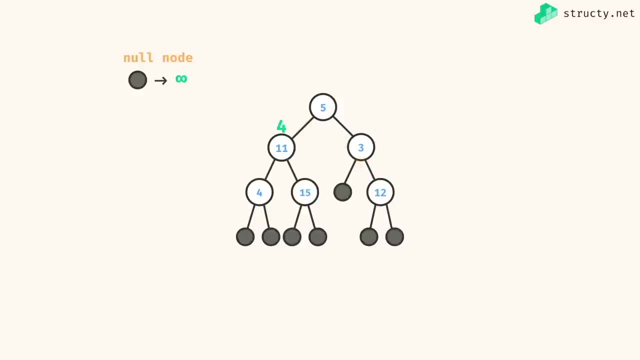 infinity: three and 12.. The minimum there is three. And finally, at the ultimate route, I do the comparison And I check what's the smallest among four, five and three, and the answer is going to be the three right, which is exactly what we expected. And so, just by 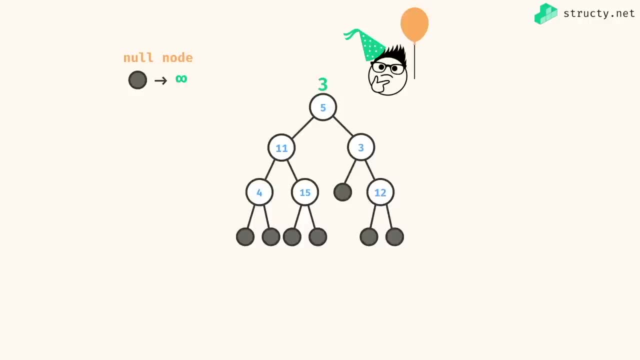 adding a little variation to our classic depth first recursion, we can totally solve this problem. So what we're going to do is we're going to define our child sub solutions into our main solution is to just do a comparison right. So, overall, at every point of this, 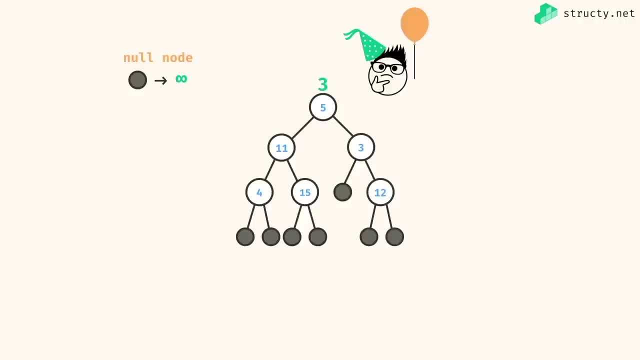 tree. we asked ourselves right, given the smallest value in the left subtree and given the smallest value in the right subtree, I compare those to myself and return the smallest among those three. And now, when it comes to the complexity of this, it's pretty straightforward. 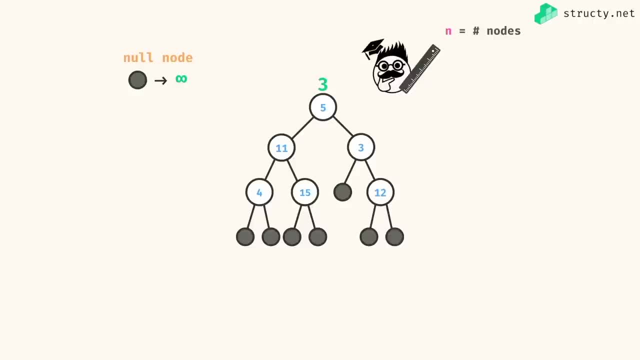 We'll go ahead and say that n is the number of nodes within our input tree, And we know that we're going to have a call for every node of this tree. So that seems to be, O of n time, in terms of the number of recursive calls, right And 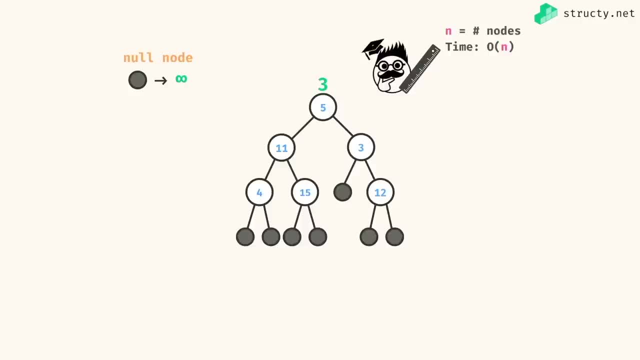 we know, within any particular recursive call. it sounds like we're just going to do some conditional logic right, just find the minimum among three things. Since three is a constant number, I'm pretty sure that we're going to have just an overall time complexity of O. 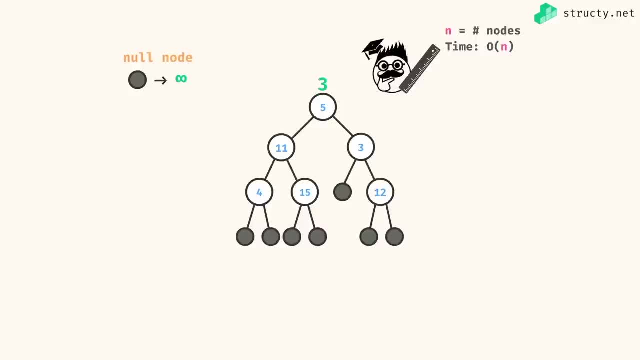 of n, considering the number of calls that we make. That being said, we will also have O of n space complexity just due to the call stack that we use for baseline depth first traversal. So that seems to be an optimal solution for this problem. is what we'll do. we'll go ahead. 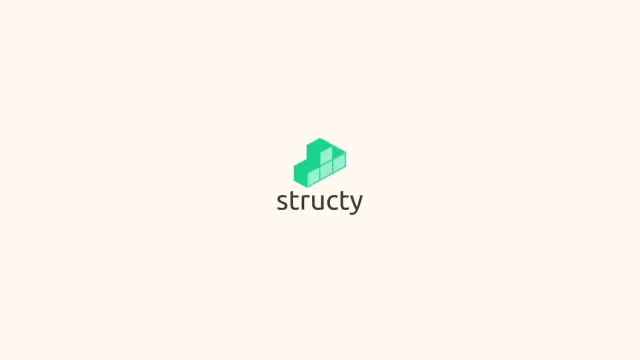 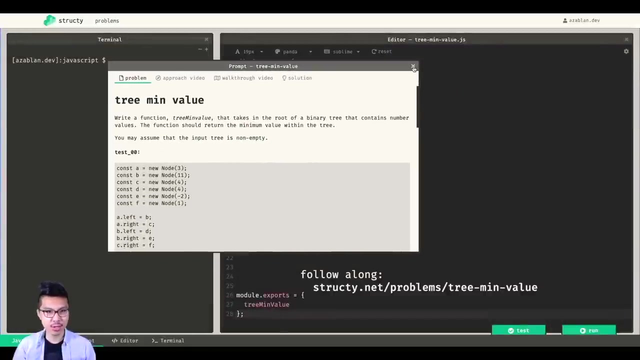 and code this one up And I'll catch you in the next one. Hey programmers, Alvin here. right now I want to go over a JavaScript solution for this tree min value problem And of course, we'll solve this one a few different ways, I think. 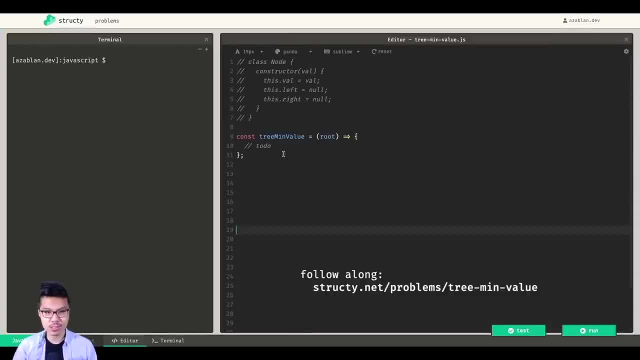 I'll start by showing y'all, maybe, some iterative solutions, And so we'll just do some classic depth first and also breadth first along the way, right? so you know you're going to need to iterate or hit every node, Okay, so we're going to go ahead and do that. So we're going to go ahead and do that, And 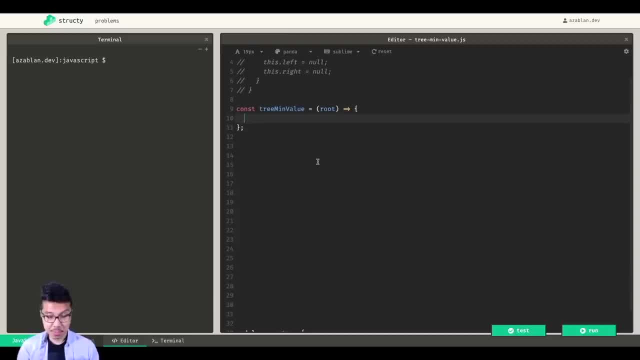 Okay, so we're going to go ahead and do that. Okay, so we're going to go ahead and do that. Okay, let's call g an t as a node within your binary tree. So just go ahead and set up either stack. 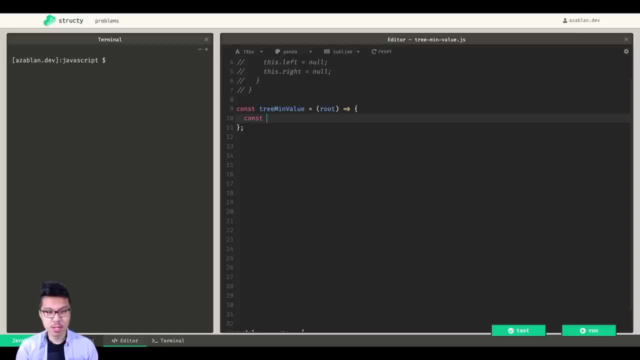 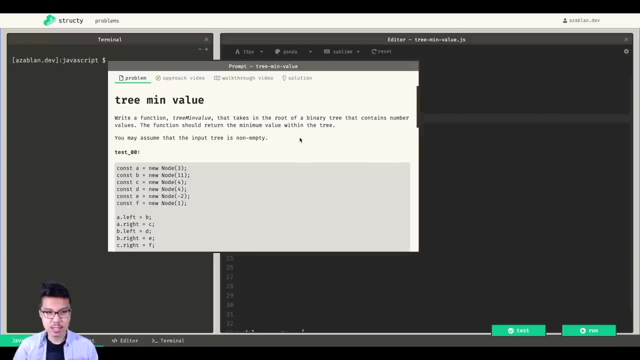 or queue, So I'll choose to start with a stack over here. So say: const stack equals empty, And one thing I'll have to be aware of is, looking at the assumptions in the problem, They tell us that we can assume that the input tree is not empty, And so that means I won't. 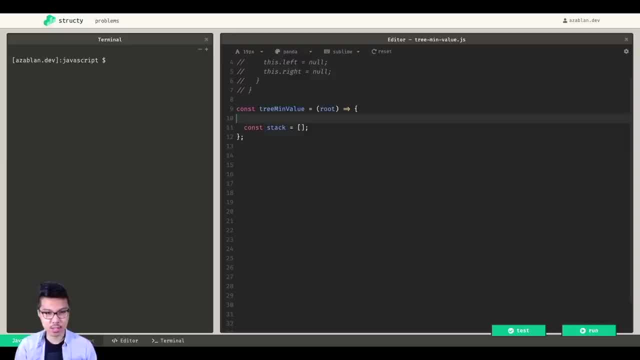 need to add a leading if statement checking if the top level root is not. so I can just go ahead and initialize my stack with the root node inside, Cool. Then from there you need your main a loop to iterate through the different nodes. So I'm going to loop while my stack is not. 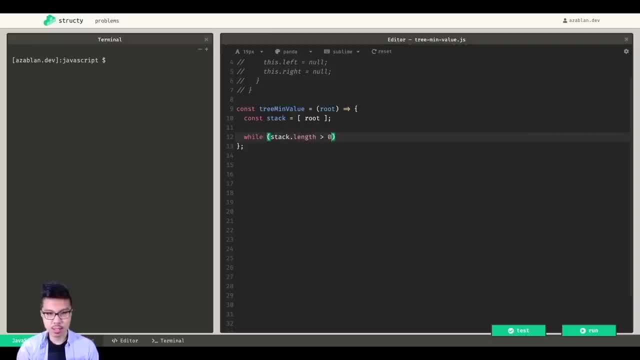 empty, So I'll stack. the length is bigger than zero, Cool. So if that's the case and there are still some nodes to visit, I begin a single iteration of this algorithm. let's say depth first, by doing stack dot pop. So I move the top of my stack. go ahead and call. 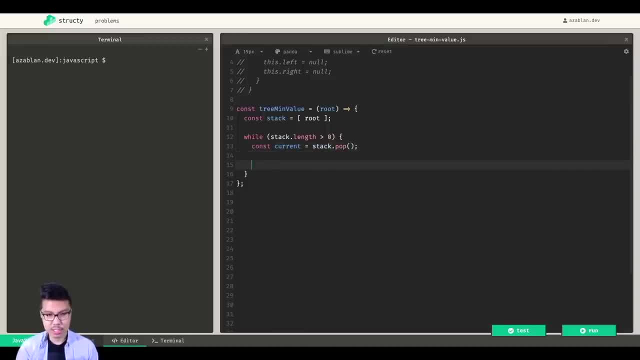 that my current, And then from there, of course, we need to check if our children exist, And if they do, I'll add them to the top of my stack, right. So I'll write a pattern like this. I'll say: if, let's say, current dot left that is not equal to null, then I can go ahead. 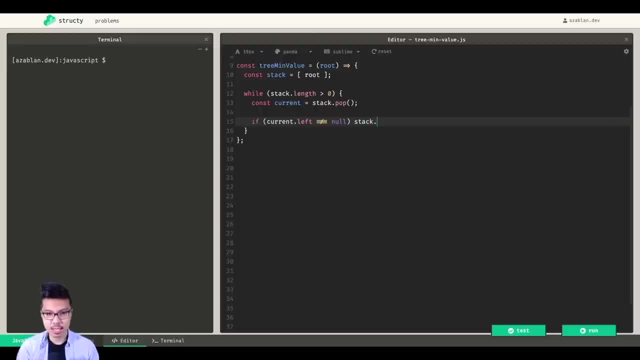 and push that existent child on the stack right. So stack dot push and I'll push current dot left. written this a few times by now should be second nature And I'll do some same code for the right hand side And this is kind of my baseline of a depth first reversal. 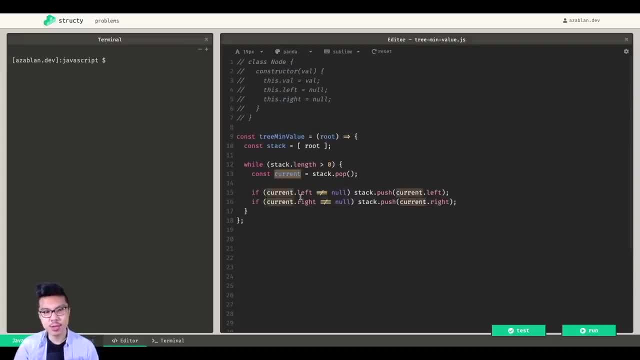 right, But as I look at this current node and its value, I want to, by the end of my loop, have access to the minimum value within the tree, And so, because I need to find the minimum value and this function, I'm going to use a variable that I'll update over time, right? 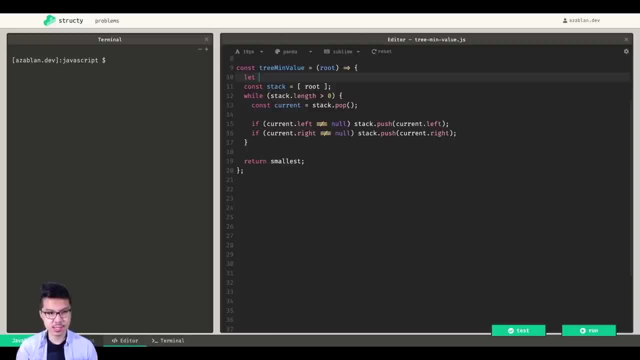 to track the current smallest thing I've seen, So I'll initialize this as let smallest. we have to think about a good default value for this, And so I'll go ahead and initialize this to actually positive infinity. So if you're unfamiliar with some JavaScript, infinity is basically just a number, as guaranteed. 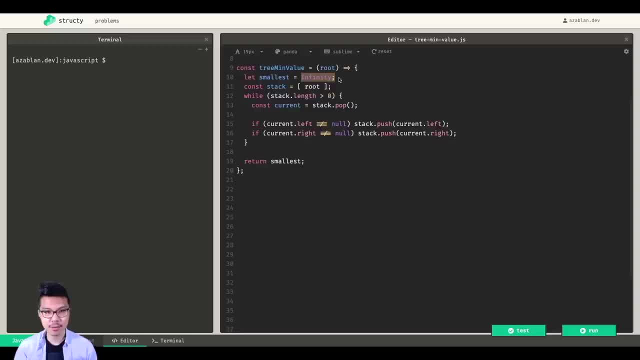 to be bigger than all other numbers except for itself: infinity right. And the reason I'm choosing a big number, like positive infinity for my default value for the smallest variable is because when I see any actual values of my tree, I know they're guaranteed to be less. 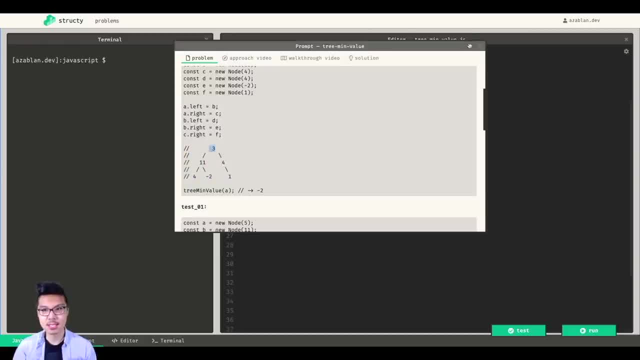 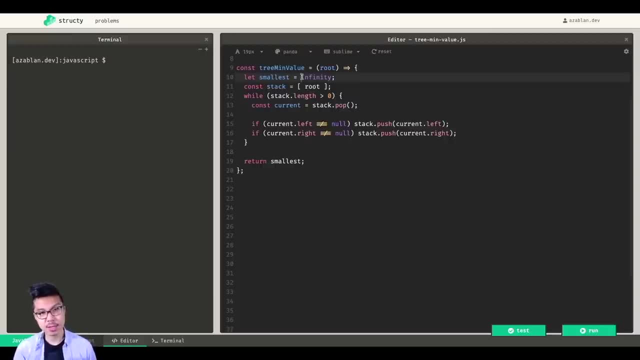 than infinity. So these numbers would replace my infinity. just gives me a good initial value, right? So if you're looking for a common pattern, right? if you're looking for the minimum thing, then typically your default value is positive infinity. If you're looking for a maximal, 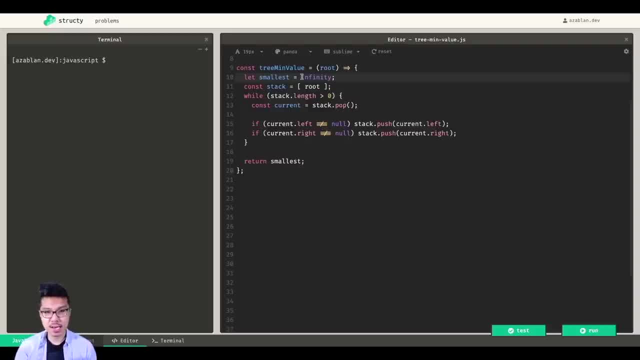 thing, then your default value might be zero or negative, infinity, depending on the problem you're trying to solve. And so, with that default value, or do I actually want to replace it? right, And I'll choose to do that right after something leaves my stack. That way, I only 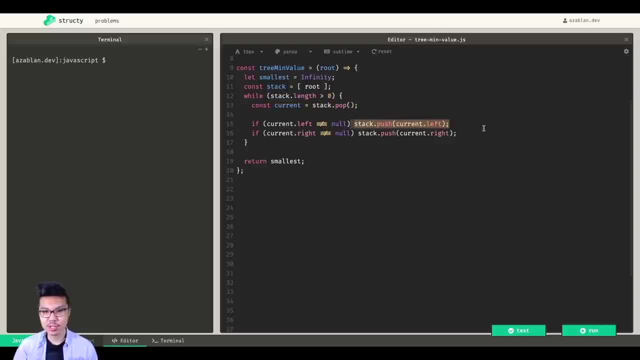 have to say it once. If I wrote it when I added my children into the stack, I have to say it twice, right, which is kind of annoying. So I'll just check. hey, if current value or the actual number value, current value is less than the smallest, then I've just 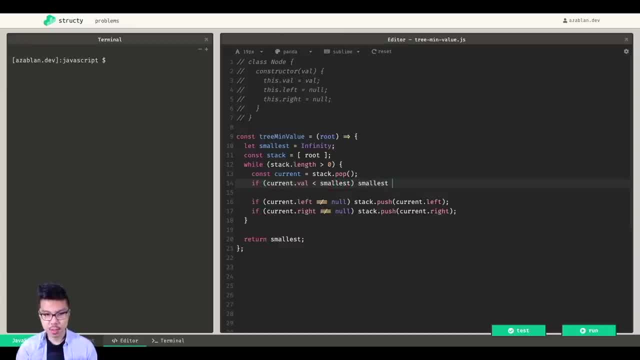 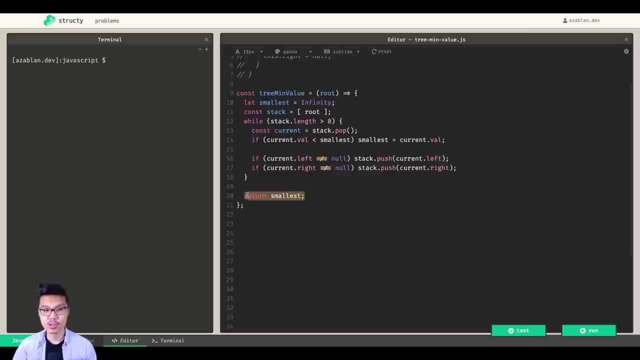 found a new, smallest right. So just replace that variable with current val. Of course, by the end of our while loop we should just return that variable right And we should have the true minimum. So let's give that a shot, run these test cases And this is. 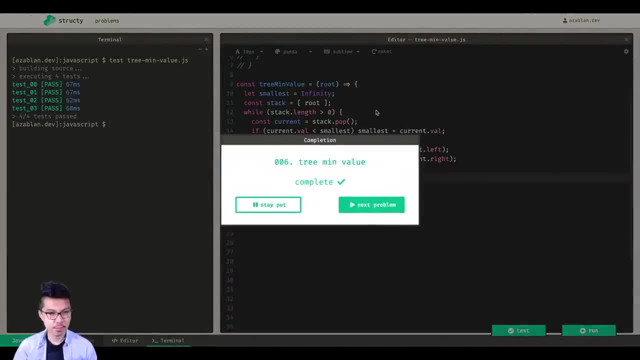 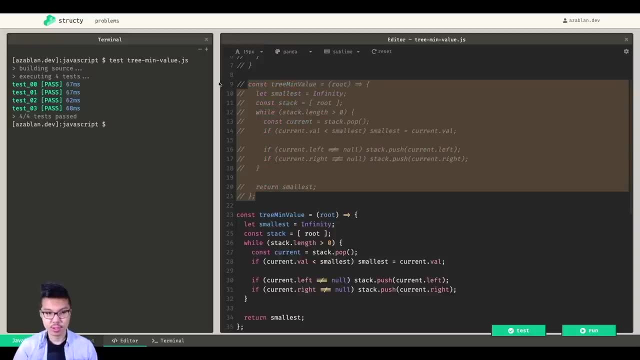 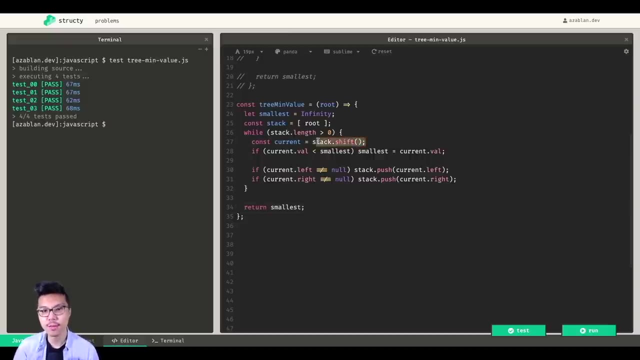 our rendition of an iterative depth first right. Awesome. So if you want to switch it up, You know writing the breadth first is super trivial in terms of the change we make. you can just make sure you do stack dot shift right because that would remove the front. 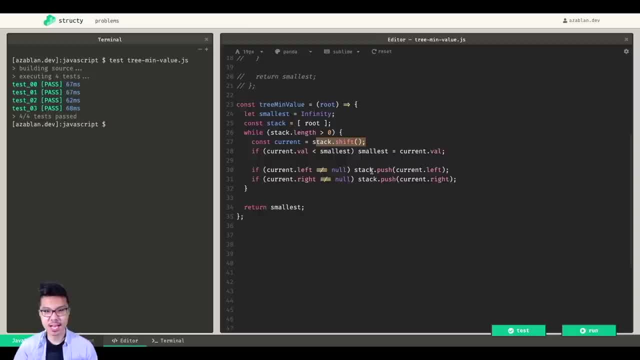 element of your queue now, And if you push and you're still adding it to the back and I guess you should probably rename this guy to queue, So very minute difference. Well, pass, that, Give that a go. Cool passes, all of them, Nice. And one thing to note So at: 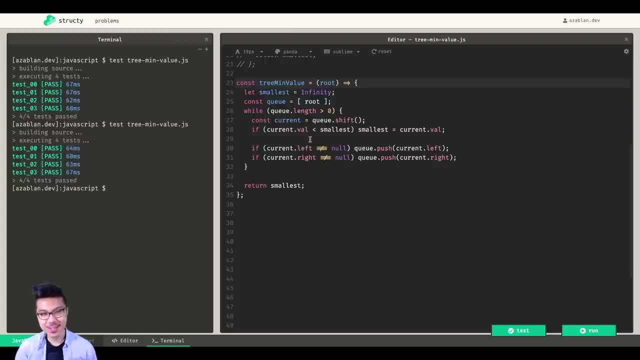 least in JavaScript. there is no immediate, at least when I recorded this video. there is no immediately available like optimal queue data structure just baked in. like you can't import it through a standard library And so when you actually do the array dot. 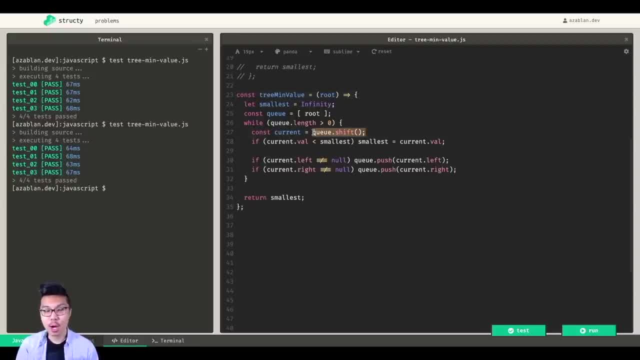 shift method, that line itself is going to run an O of n time right, Because if you remove the front element of an array in JavaScript, it will have to actually shift all the other elements over one position. In other words, index one becomes. 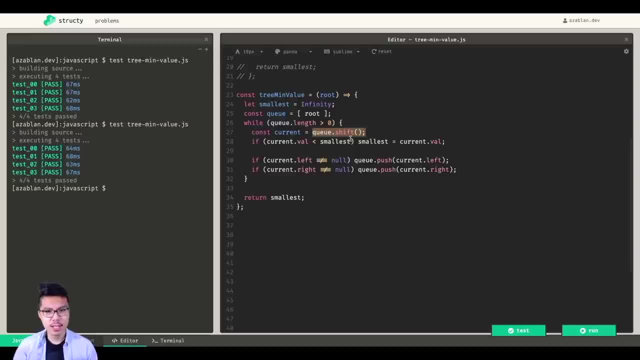 index zero, index two becomes index one, and so on. And so, technically, if you implemented your breadth first exactly like this, just using a regular array, and you shift out, then this would probably be technically like an O n squared solution, which isn't the fastest. 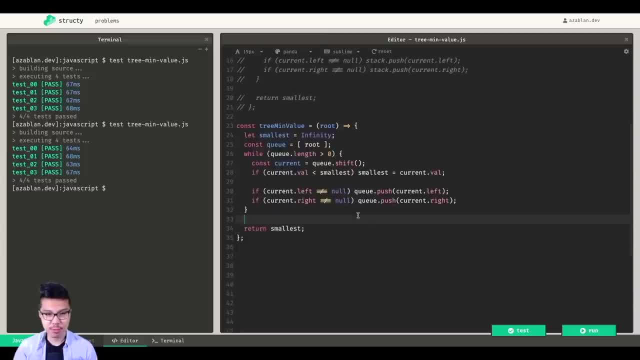 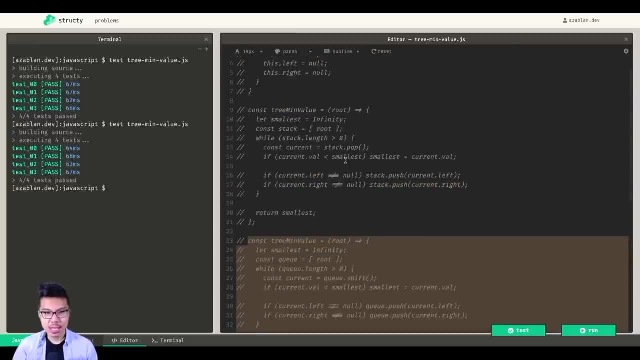 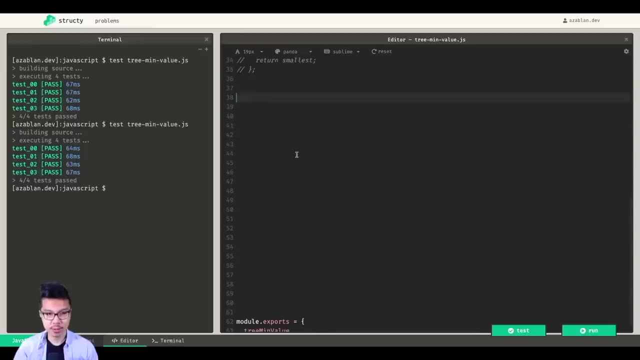 but we'll be able to pass the specs. typically, you know, n squared for most problems is kind of okay, But you can avoid it if you want to get the blazing fast solution. But now let's actually go ahead and implement my favorite version, which would be a recursive version, right, which is technically of the depth. first, 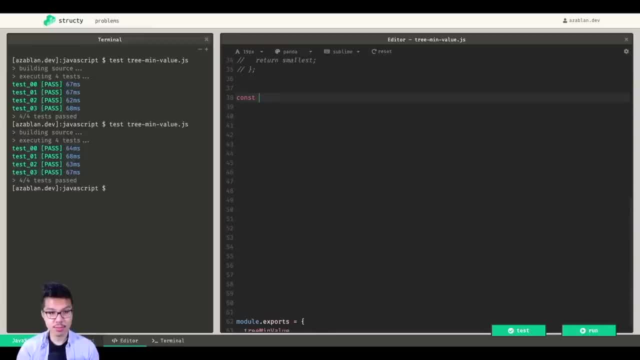 Right. So we'll say: const, is it treatment value? Yeah, treatment value, dream and value. And to establish this one recursively, we'll always start with our base case, right? So we need some of these curly guys. So I'll start with my base case. I'll say: if my roots 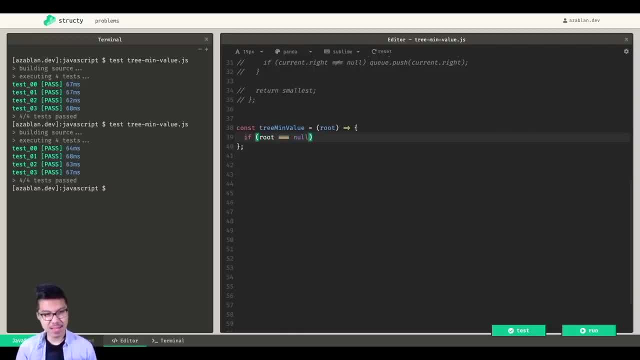 is equal to no, then that kind of means I have the empty tree. So what's like the minimum value in the empty tree? Well, that must be infinity, right. For the same reason, we chose infinity before right. It's just a good default value, because I'm going to minimize in the 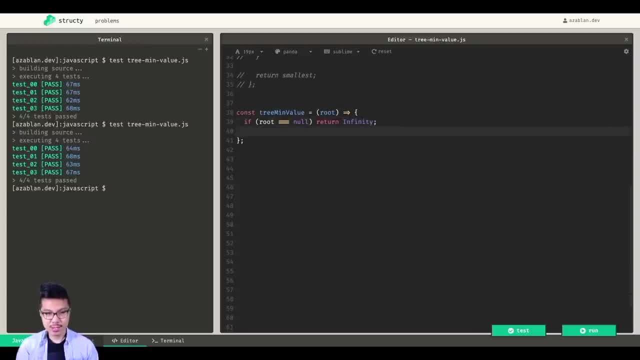 long run. Cool. And now what I want to do is I want to make my recursive call. So if I call tree min value on my left child and I call it on my right child, I'll just think about what these function calls return- right, although they were cursive- if these calls 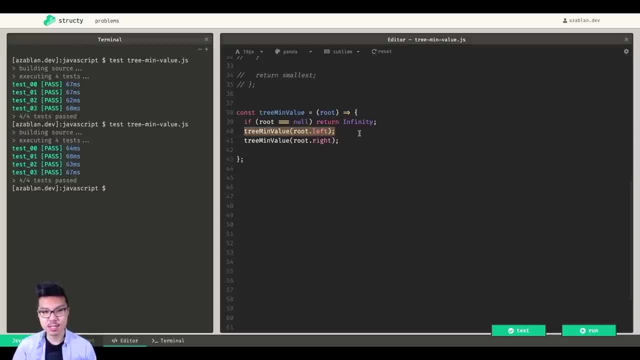 work. they should give me back the smallest value in the left subtree and the smallest value in the right subtree. So maybe, just to be clear, I'll go ahead and save these system variables. I'll say const, I'll say left min, And also this should be the right. 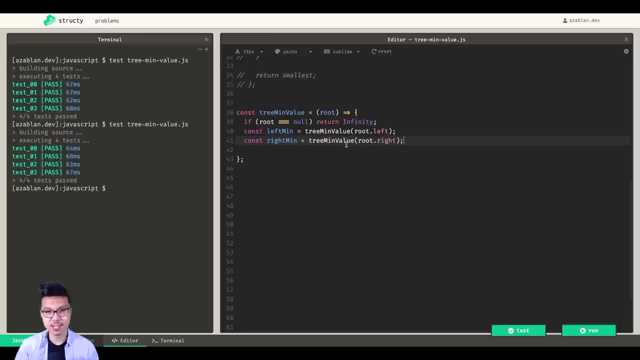 man right. So I found the smallest on the left and the smallest on the right. But I also need to think about myself. right, I am root dot val, So I need to choose the smallest of root val: left min and right min Right. 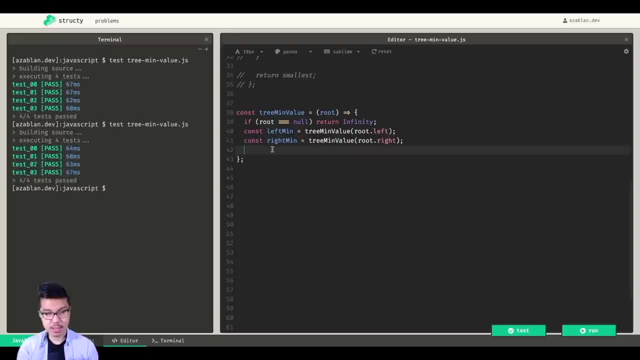 so you can write like a conditional. So just some if statements, if you want. I think the best way to implement this in JavaScript is just to use the math dot min function. So JavaScript you always have access to the global capital. math object has a few useful methods on it. One we're going to. 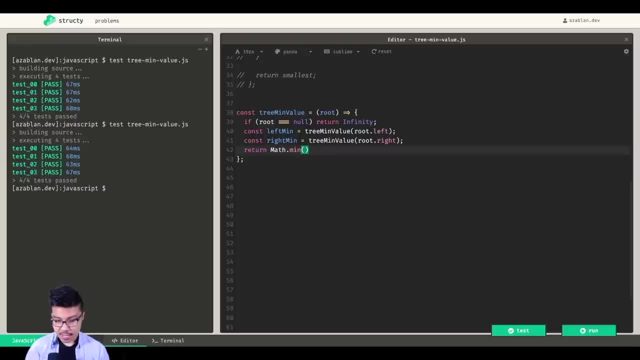 find useful right now is math dot min. And if you do that you can pass in some arguments and an arbitrary number of arguments. So give me the smallest between route dot val. be sure to access the value because you need to give numbers to min right. smallest between route dot val: my left min. 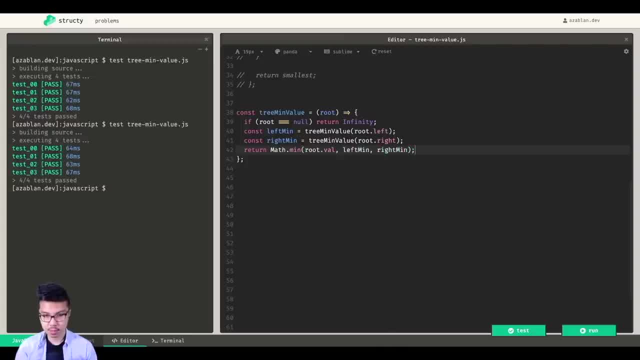 and my right man Cool. And this feels somewhat similar to the approach drawing we did right, Where we had to choose the smallest of these three numbers. So before we run it- maybe you're unfamiliar with math, dot man, I can quickly demo that for you- Let's say I had some numbers we had- 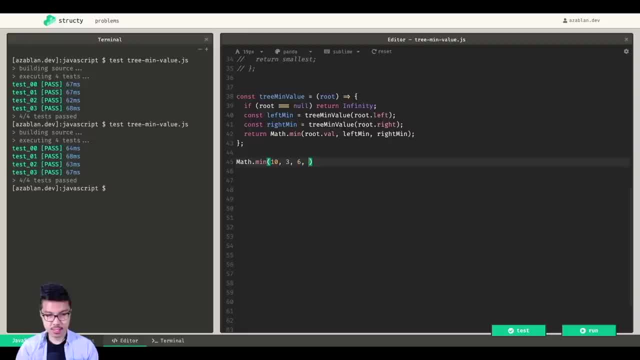 10,, we had 3,, we had 4,, we had 5,, we had 8,, we had 9,, we had 10,, we had 9,, we had 10,, we had 11,, we had had three, we had six and we had negative 12. And also 100.. And if I console log with: 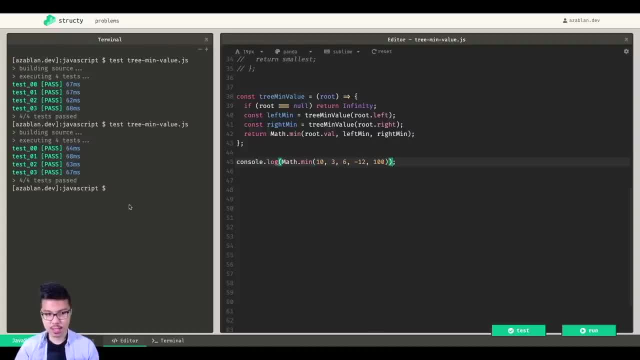 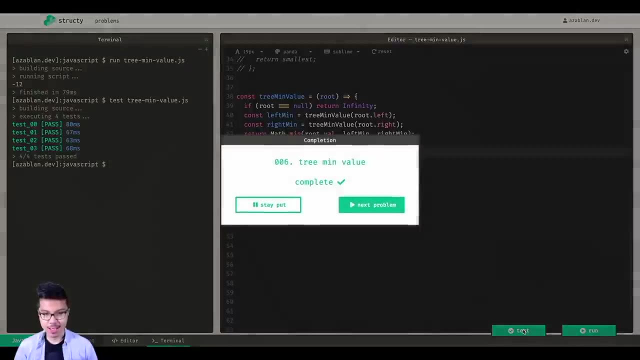 that returns. I'll just run this file as a script, So I'm not going to execute the test quite yet. So I should get negative 12. Because that's the smallest, perfect. And now I think we're ready to go ahead and test this. So our recursive version. there we have it, Cool. 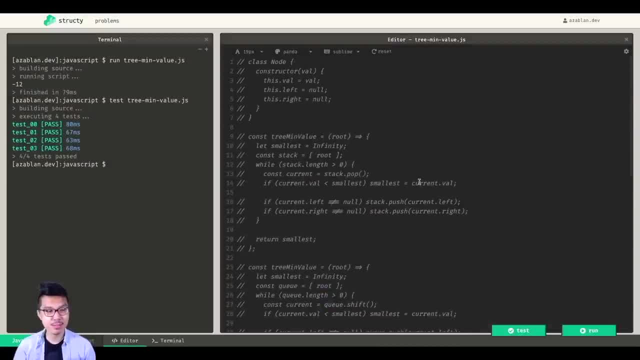 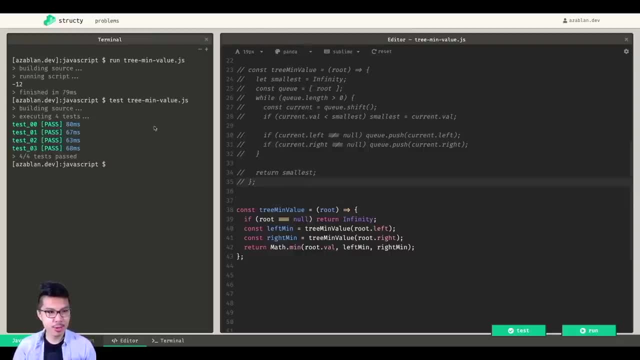 Alright, so there we have our JavaScript walkthrough for this tree min value problem. recommend you practice all of these different solutions and then pick a favorite maybe just have in your back pocket. That way you can always solve this problem in the future, right? So? 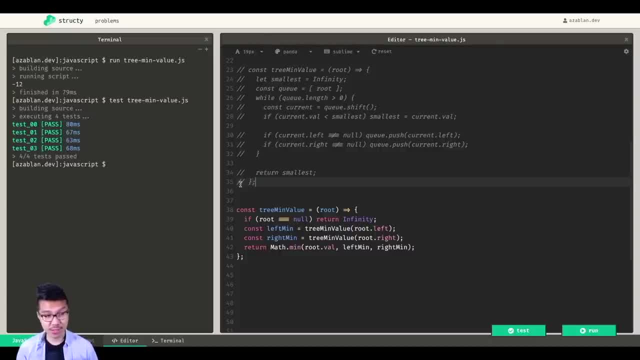 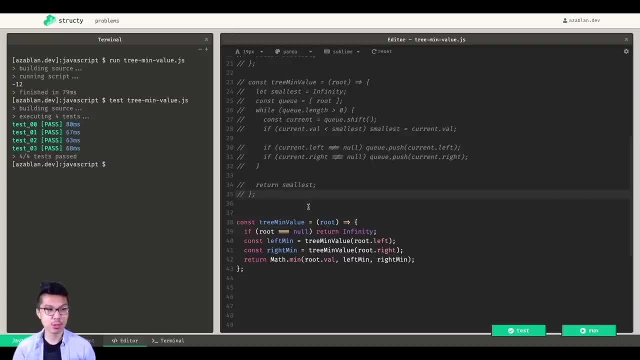 you should have no issue thinking about how to solve, like a tree, max value problem. And by now you know we're getting pretty comfortable with trees And typically we're always going to fall back to either a breadth first or a depth first, reversal, But in the next few 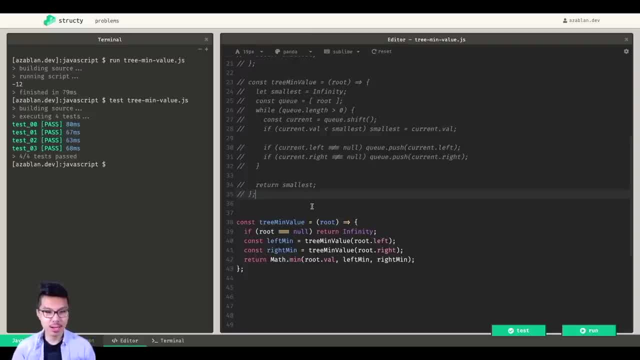 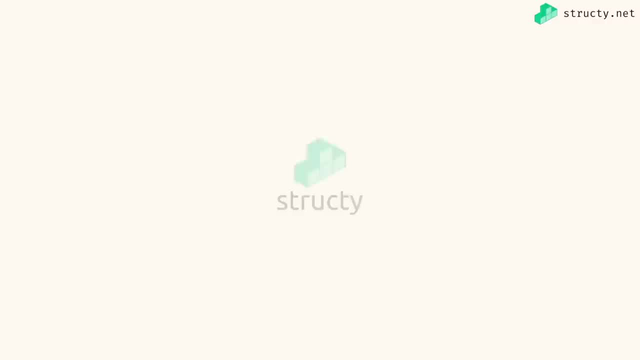 problems. we're definitely going to look at some spin offs and some variations on how we can accomplish more, More complex logic using these algorithms as our baseline. So I'll catch you in the next one. Hey, programmers, Alvin here, right now I want to go over this max root to leaf path. 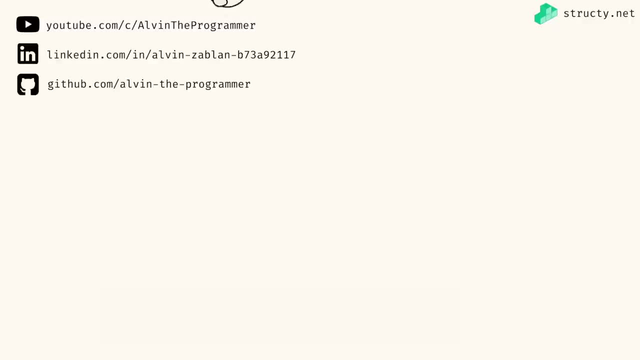 some problem, pretty wordy title. let's take a look at what this problem asks us to do. So we're going to be taking in a binary tree as input And we want to do is really talk about the paths within this tree, in particular root to leaf paths. So just to review, we 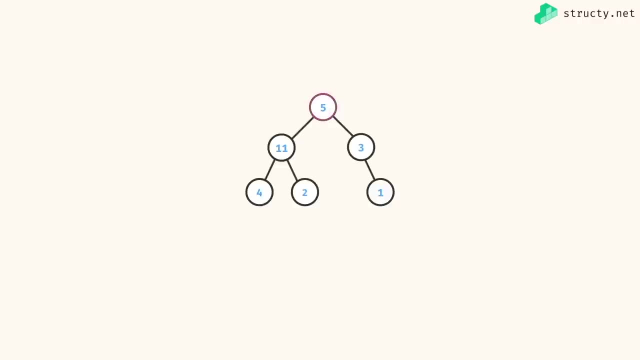 know that a binary tree, typically for us, has a single root And you can identify the root by just looking at the topmost node, that is the node with no parent right. And then also, given this tree, there are three leaves right A leaf is a node that has no children. So 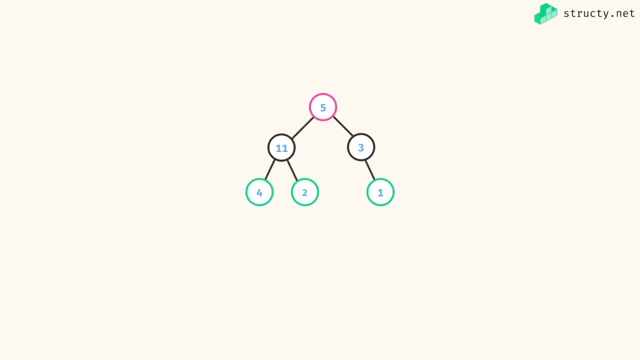 do bear in mind: right, a root has no parent. a leaf node has no children, something like 11.. And three: in this picture there are neither roots nor leaves, right, So it could be the case that a tree has many leaves, like this tree. right, it has three leaves, But 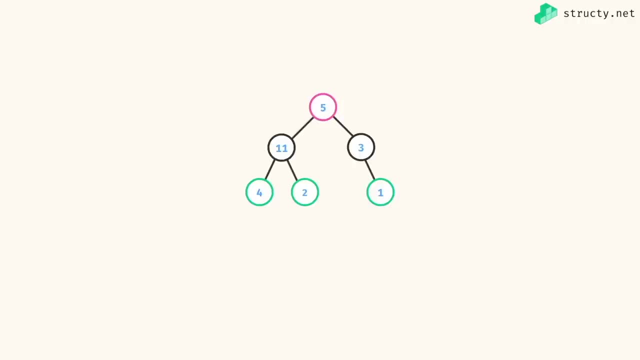 a tree for us typically only has a single root, And so what we want to do is consider all three of the different root to leaf paths right. so you must start at the root and you must terminate at a leaf, So one of those paths would just be this one right: 511.. 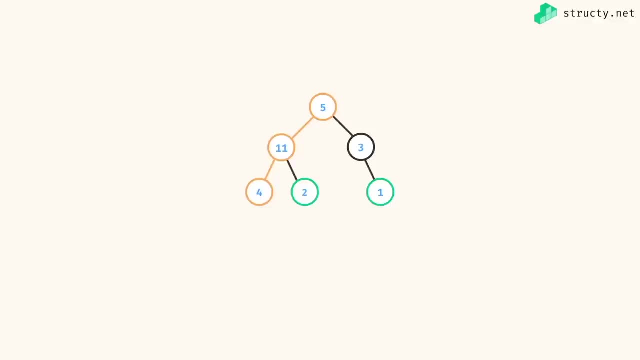 Four, And what we want to do is consider its total sum. So just summing the values within the nodes along that path, if I do five plus 11, plus four, that would give me a total sum of 20.. So that's just one of the possibilities. If I look at another path, I'm going to have 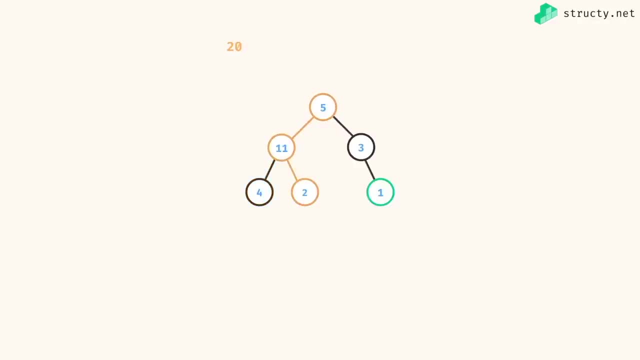 another path, let's say, this path of 511, 25 plus 11, plus two, would give me 18.. That's another option. And the only other option is this final path from five to one: by do five plus three plus one, that gives me a total sum of nine. right, And now, among those, 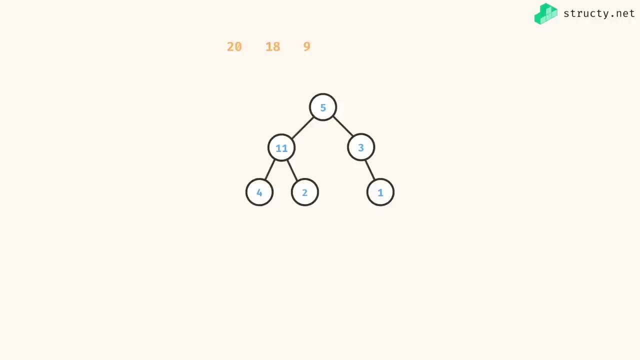 three options. I want to choose the maximal path sum, right, So that would be a final answer of 20.. So in the long run we need to come up with some code that computes the maximal path sum from the root to n. 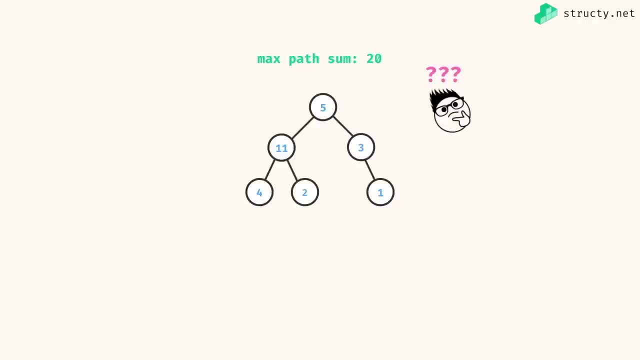 So for this example, I want to set it at s, because essentially we want to find the absolutamente least amount ofSave, And once we've had, we've got two headers And we'd change the interess to be relatively least two. So let's go ahead and do that. And now, 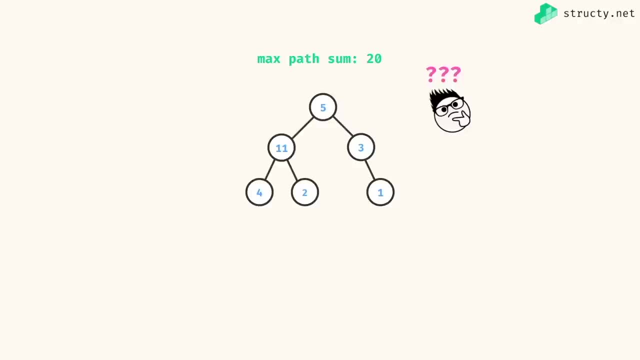 we have the optimal path sum of the'. Now, when we do that, I'm going to set the under the default value of one. please note that because I didn't write this out just once. Two front も튼: One certain value of the default value. right, if you're using a default. 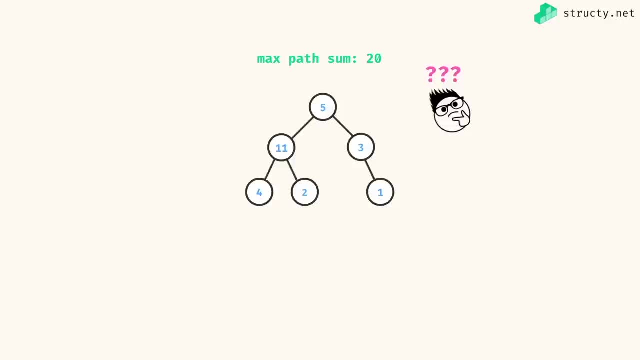 value. So I should be able to do all of these and I should, you know, be able to count all of to come up with a pretty novel solution. But it's okay to rely heavily on our previous experiences, right? And so let's start with something classic. I think we're going to solve this one recursively. 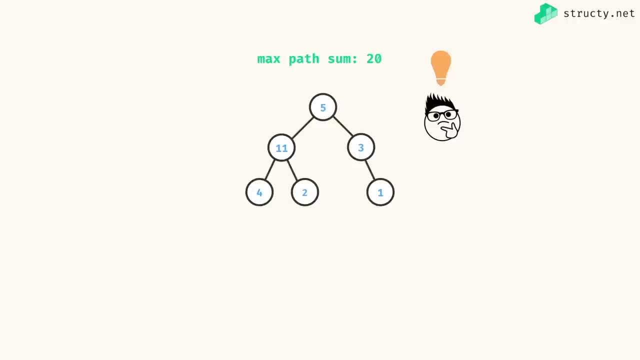 And in the grand scheme of things, typically for tree problems, that is, a recursive code is usually your best bet when it comes to like pathfinding things right and building paths and determining paths, And so we'll take a look at what we should have our base cases be if we're going to frame. 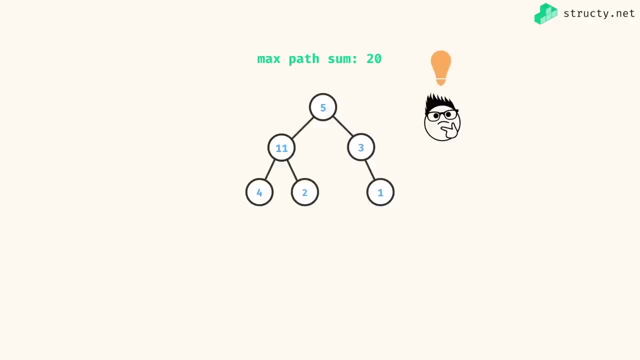 this one recursively. So they tell us that, all right, you need to consider paths, but not just any paths. right, You always want to end at a leaf node, So the leaf nodes like the ending point. the leaf node is the base case. So my base case is going to be literally about a leaf node And 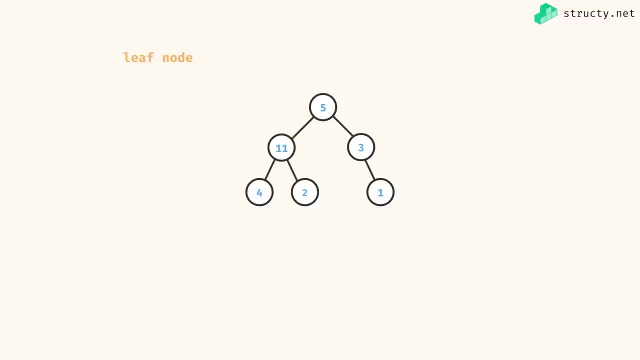 recall that that's a node with no children. So, for example, let's say we had a node as input that had no children, then what's the total sum of that leaf node? Well, it would just be its inner value. n right. 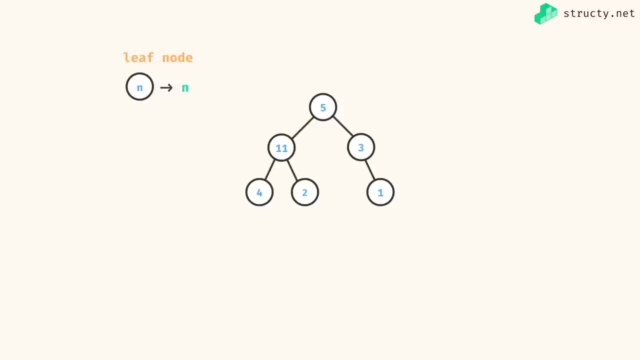 So kind of think about your base cases as if they're their own inputs, right, As a quick aside, right? so a totally separate scenario right now. let's say, I gave you a tree that contains only one node and its value was 42. And I asked you to: Alright, tell me. 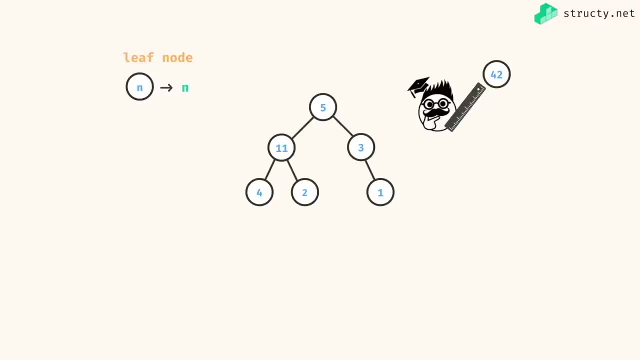 what's the maximum path sum of this tree? this tree is very small, right? If you identify the root in this tree, it's just the 42 node. right Because it has no parent. And I also asked you for the leaves. there's only one leaf here And it's also the 42,. right Because it has no children. 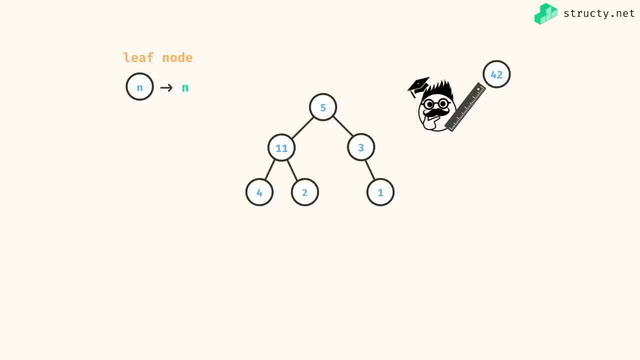 right. So the single node of 42, in this example is the root and the leaf, which means that the maximal path sum would just be 42.. Cool, So I'm thinking about my base cases as if they're their own inputs. Nice, And what you'll probably recognize here is: in this scenario we're kind. 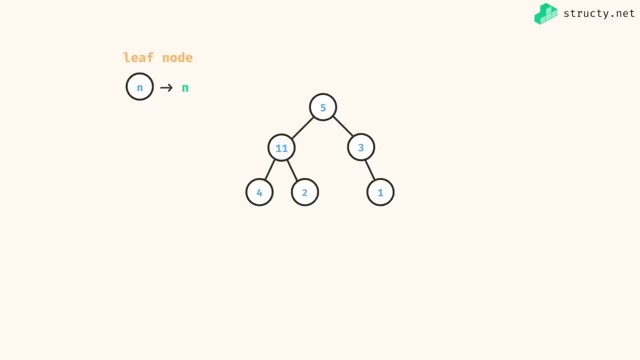 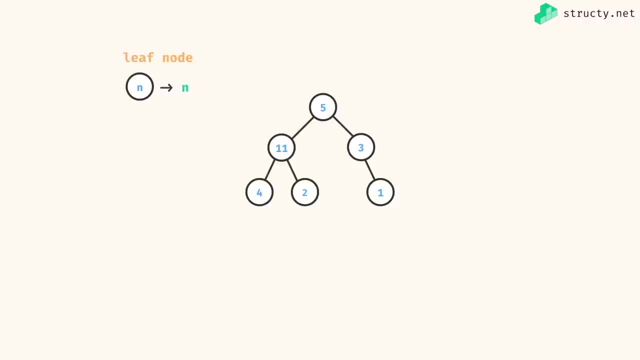 the problem, right? They say root to leaf path- Awesome. So if that's the case, I'm just going to locate all of my leaf nodes in this diagram And I know that they're going to return the values within them. So just plugging those in right, And now I can start reconstructing on my higher level. 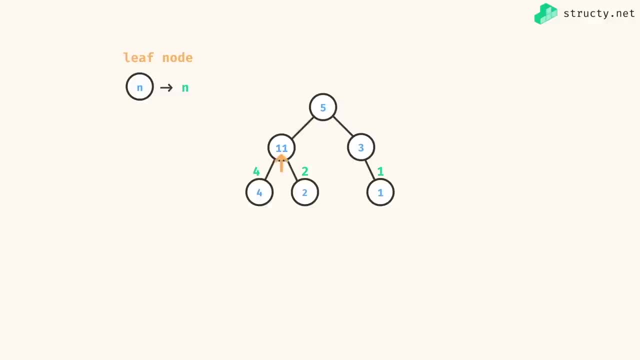 solutions right. So, given this 11 node, what decision does this 11 node have to make to compute its answer, right? So let's read ourselves at this 11 node, And we have to consider our left and right values, right. And so, if I root myself at 11, the four represents my max path. sum through my left. 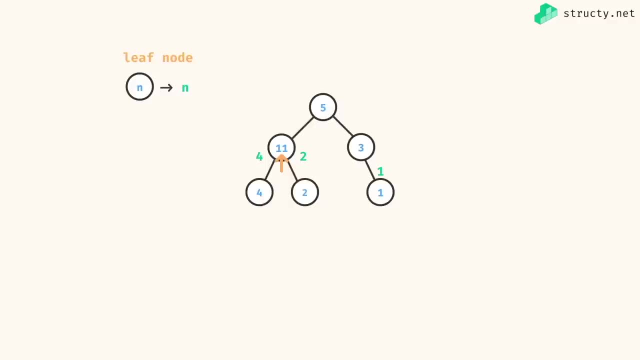 sub tree and the right hand side to now represents the max path sum through my right sub tree. Since I want to maximize here, the key is to just choose between four and two. right, I choose the bigger of them, right. So four is bigger than two, So I must use the four And 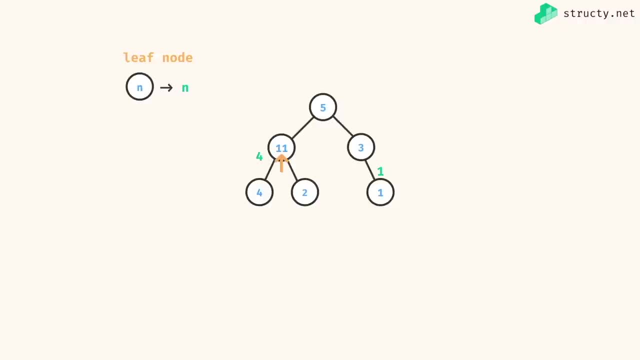 what I do is I take that four and I add my current value of 11 into it, And that gives me 15.. And now I can actually be the answer for this subtree. In other words, I can check for correctness right now. 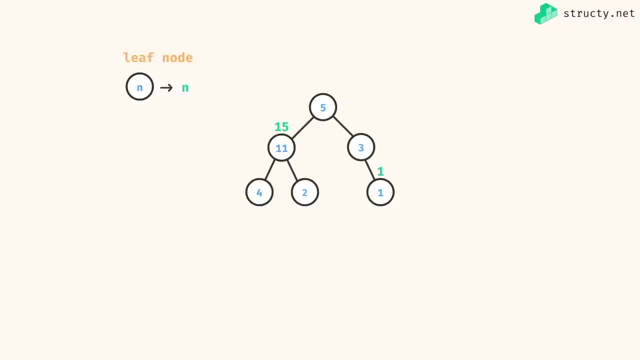 if I root myself at 11, I'm returning 15 to represent this path. right, I can either do 11 plus four, which is 15.. Or I can do 11 plus two, which is 13.. Right, And that 13 is smaller. 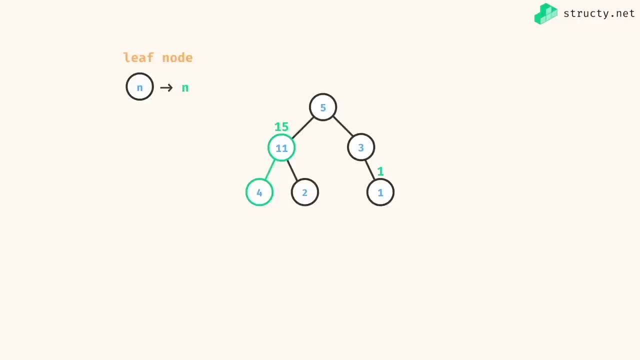 so I won't prefer it here. Cool, So so far it seems like we're in good shape. Now let's take a look at another node we need to evaluate. So get this three node So it has a value on its right hand side. right, it's receiving a one from its right child. 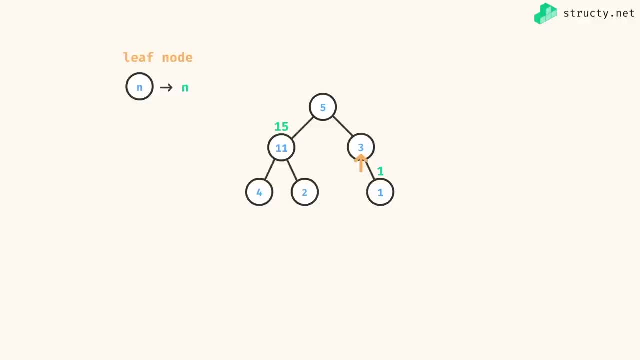 but the left child doesn't exist, right. And if you want to be a little more explicit, we know that the left child, or three dot left, is going to be a null pointer, Alright. so kind of plug that in here And here's where we should work in possibly another base case. sometimes it's very 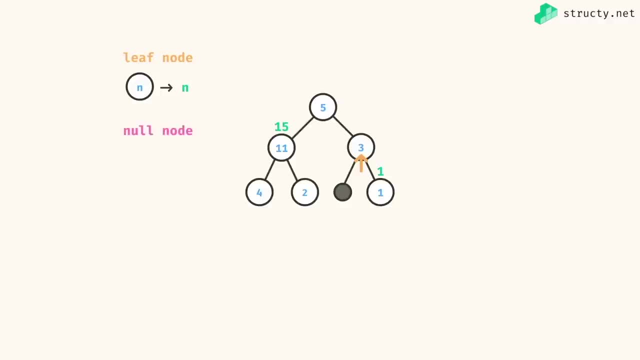 natural, just course, correct as we go. And so, for a null node, what should we return? Well, we know that whenever we have a null node, it should never contribute to our final answer. we can kind of just ignore it, I guess. But we want to make sure that it's compatible with the rest of our internal 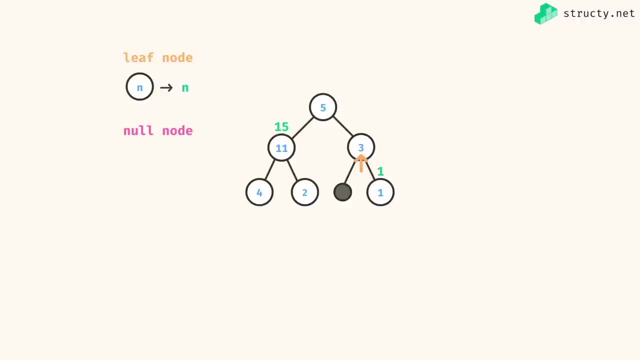 logic. So bear in mind: in this problem I want to take the maximum right Recall from our previous problem right, the min value problem. we want to take the minimum And so we made our null nodes return infinity right. Because if I want to find the minimum and my null nodes return infinity by 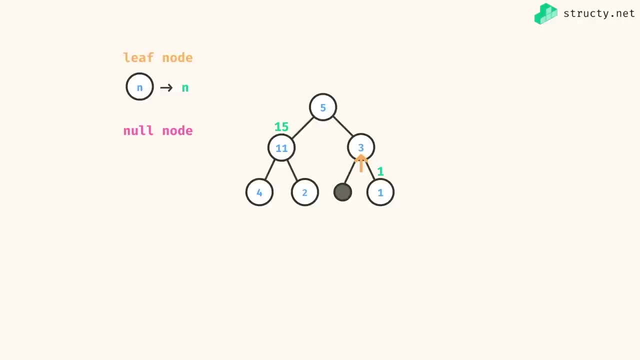 default. I know that infinity is never going to win a comparison. right, Because infinity is very large And we just want to flip that logic over here. right? So because in the long run I want to find the maximum, I'll make my base case for the null nodes return negative infinity. right, Because I? 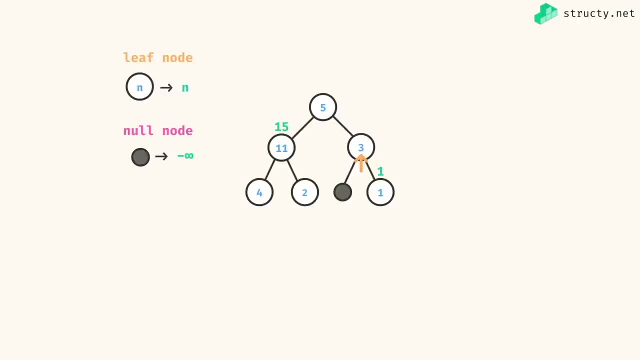 know, negative infinity is never going to win any contest where we compare things, looking for the larger of the values, right? So for this null node I'll plug in that negative infinity. And now I should be able to do the same business logic as before. right, So I'm rooting myself at the three. 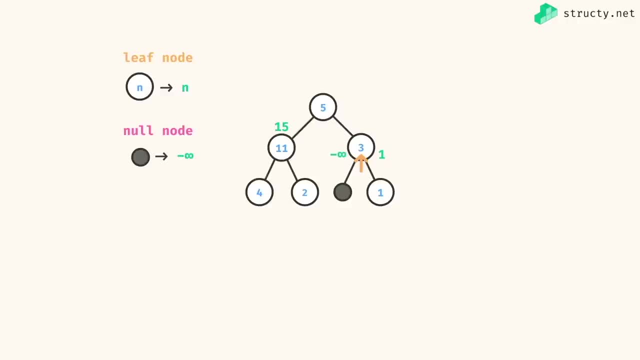 node And I can look at the results I get from my children. right, So between my two children in my left path I get a negative infinity. right So between my two children in my left path I get a negative infinity. or in my right path I get a one and I choose the maximum between them. right? 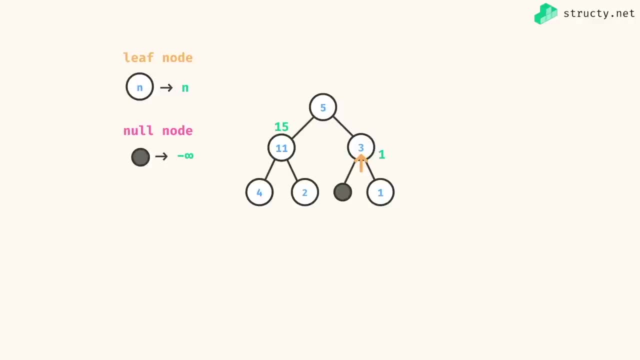 One is bigger than negative infinity, So I should use the one right. And what I do with that one is I add my current value of three to it. So three plus one gives me four right. And that makes some sense Because if I look at that small subtree, a rooted in three, the biggest path from 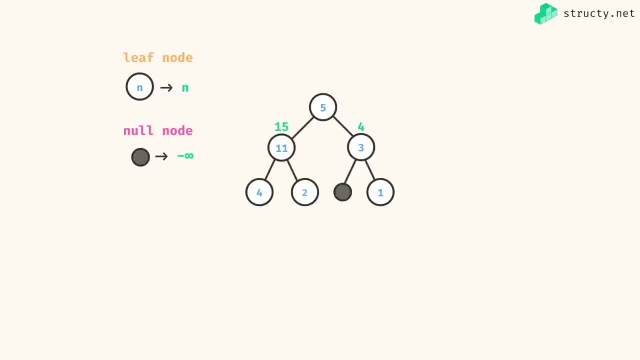 root to leaf or sub root to leaf, I would indeed be a four, Nice. And now we have ourselves at the ultimate root over here And I just want to make sure that I have the right value. So I'm going to do that similar comparison. right, I check the bigger of my two children, So I'm going to keep. 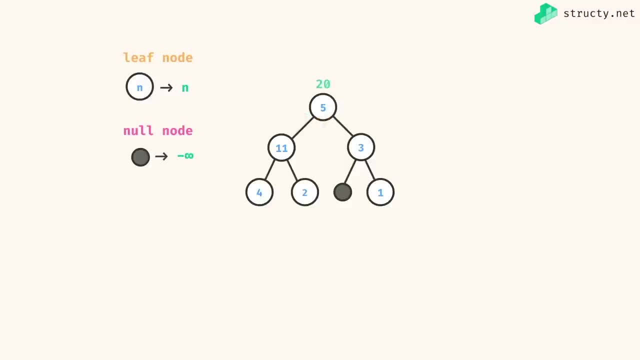 the 15. But then I add myself to it, giving 20.. Like we said before, this 20 logically represents this path of five plus 11 plus four. Cool, So there we have it, And if we want to take a look, 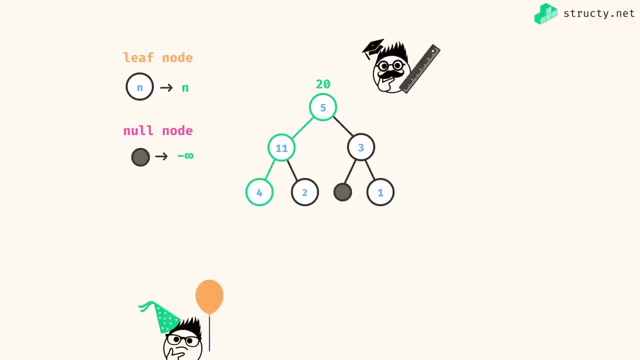 at the complexity of this, seems nothing unusual. So we're going to have n as the number of nodes. we're going to have O of n runtime because we're gonna have to make a call, a recursive call, that is, we're going to have a node within the tree And if I think about any particular call, we're going to 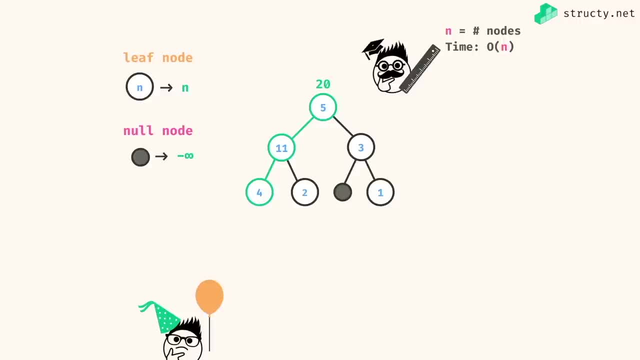 make a for a node. we're just going to do a comparison, right, I just choose the bigger of my two children, So we're not going to have any any loops within our calls, I believe. Cool. So it just seems to be O of n time And, like we always say, space complexity is O of n. 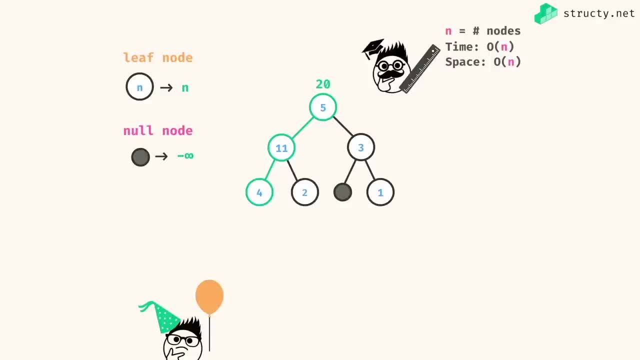 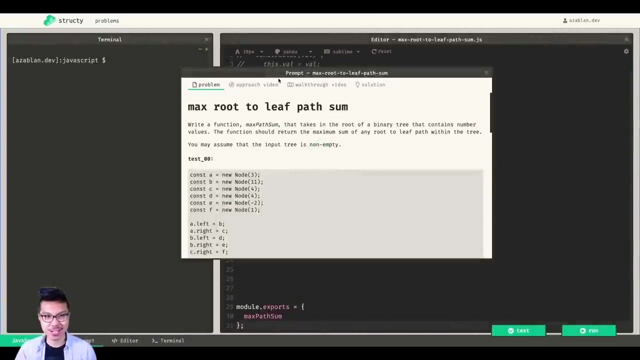 just due to the call stack, Nice. So let's go ahead and code this one up And it should feel like a combination of our previous tree. some problems, as well as some min value, max value, Logic. Hey programmers, welcome back. Right now I want to go over a JavaScript solution for this. 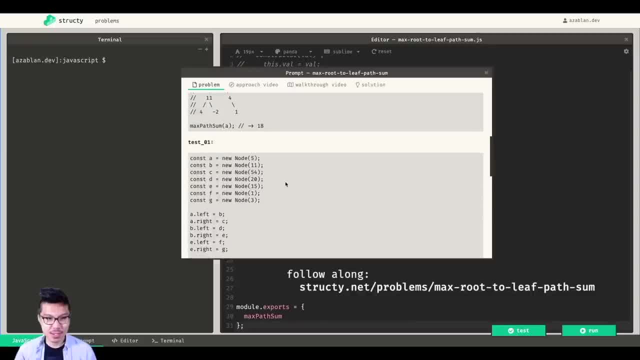 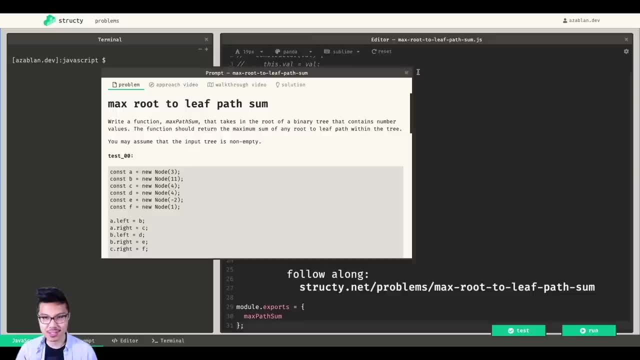 max root to leaf path some problem. So this is going to be a pretty interesting tree problem And we'll jump right into the code. please make sure you watch the approach video before this, So I think should be all primed up with the logic that we want to implement here, right And so. 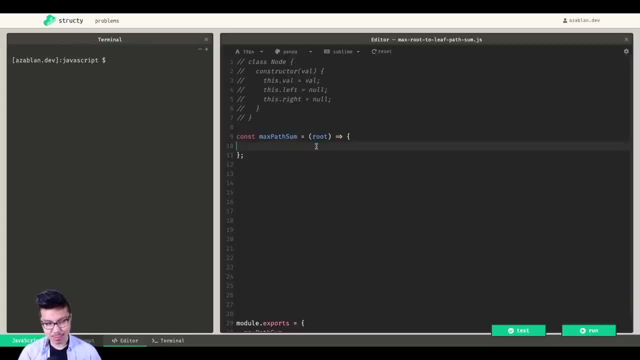 we'll start by doing this recursively, And I'd say that's probably the best way to solve this one. So I think it's the only way I'll show you, And what I want to do is start with a base case, right? So we said we want to figure out our root to leaf paths, So our base case should be about: 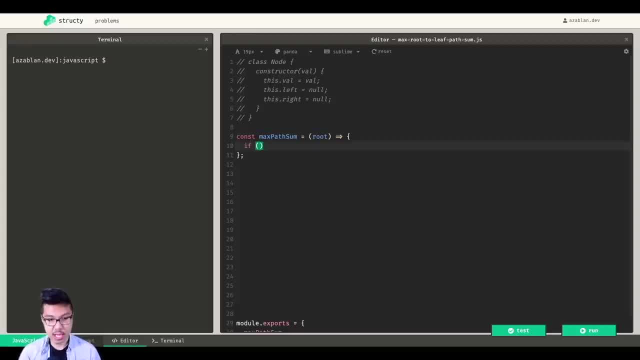 whether I have a leaf right. So I'm going to go ahead and check. let's say, if my root left is equal to null right and root right is equal to null right. that's the definition of a leaf. So if I have no left child and I have no right child, then I 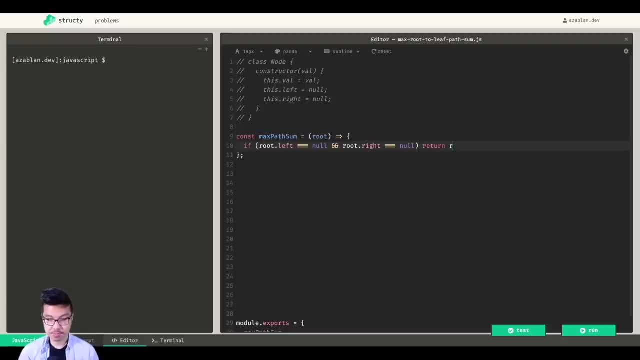 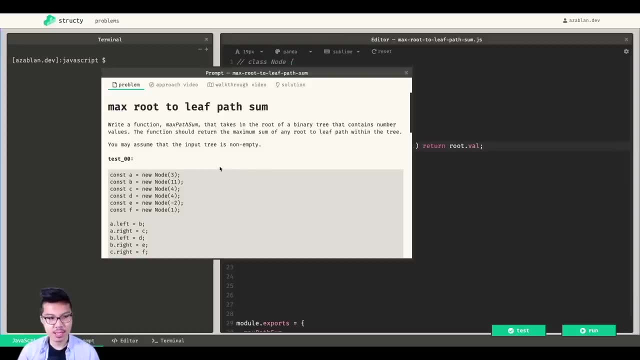 return the value stored at this node right. So root dot val, Nice. So again, what we're kind of emphasizing here is that base case catches a scenario if we're at like four right, we have no children, Nice, And we will need another base case in the long run. For now, let's say we left. 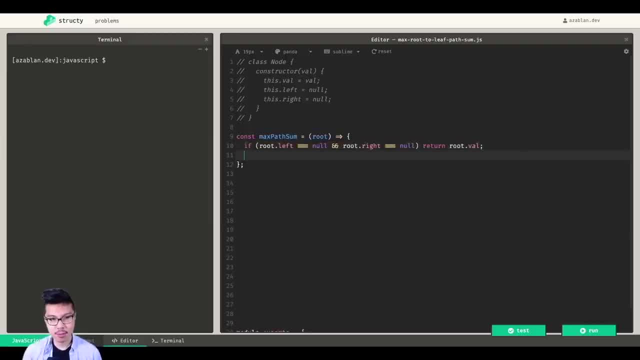 it like this, right. So we said that, in the context of solving this one recursively, the decision we make at every node is: I choose the bigger result from my left column, my right call, and then I add myself to it. right? So I know I'm going to. 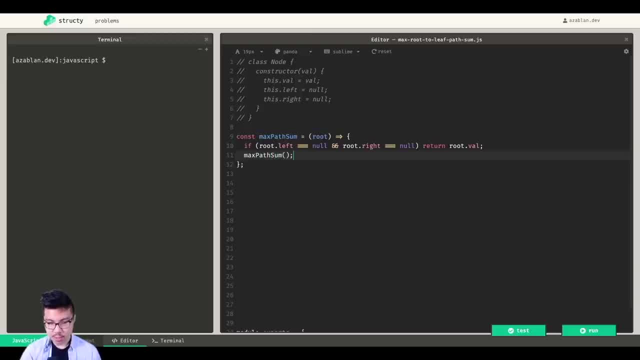 do this recursively. So I'm going to call the same function And by now you should be familiar with all. right, you call your function on root left and also root right. that I think about what those calls return. right, they give me back the max. pass some through my left subtree. 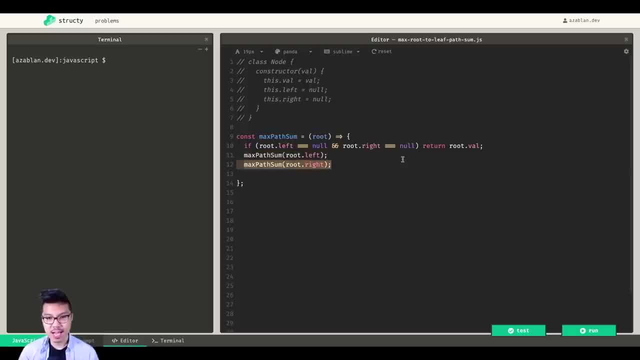 and the max path, some through my right subtree. I just want to choose the bigger results between those two. So in the last video you saw me use the math dot min function. here I'll use the math dot max function And I know that these calls these expressions evaluates. 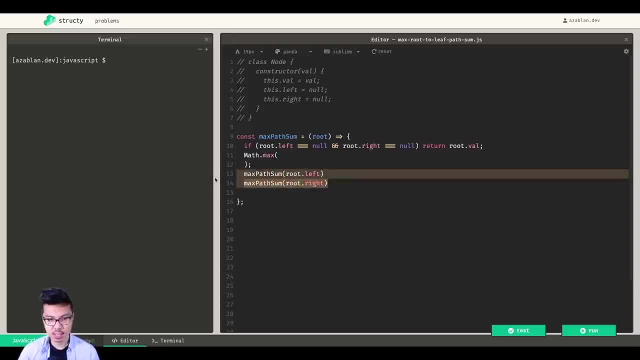 to numbers so I can actually just pass these guys in in line. So we'll just move this up like that. So I'm finding the max between these two results And I'll go ahead and call that. we'll say the max child, right? Maybe I'll write this all in line, if you prefer, And then from there 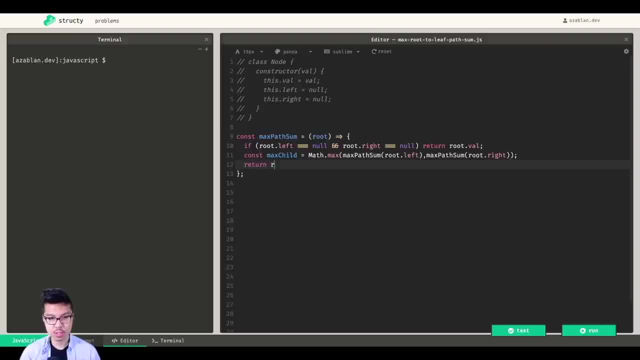 I just add myself to that max child, right? So I'm going to return root dot val, that's myself plus max child, And we'll call that max child path some. And that should be it, except for one thing we're forgetting. So take a moment, see if you can read between the lines here, And what. 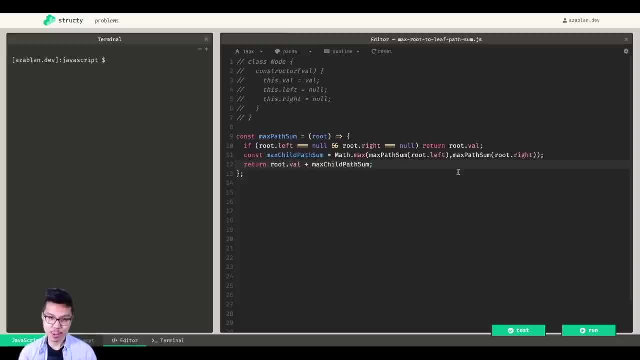 scenario am I missing? We did mention it in the approach video, So can you spot what is not present here? And that's something I find I do Often right If I'm able to really come up with a nice, meaningful and consistent picture. 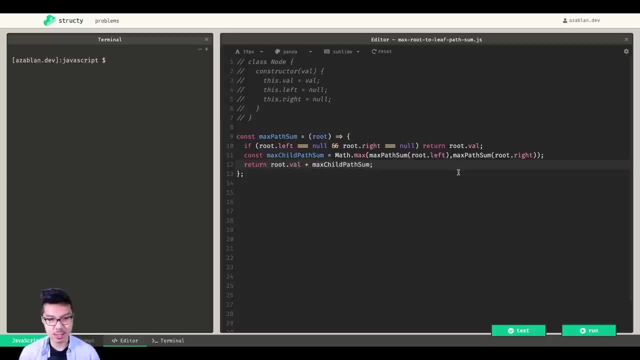 then everything I drew in the picture should translate into some piece of code over here To give it a shot. expect to fail this one. See what we get. Yeah, so we're getting an error. cannot read property left of null right. I'm failing on the very first example, So I'll. 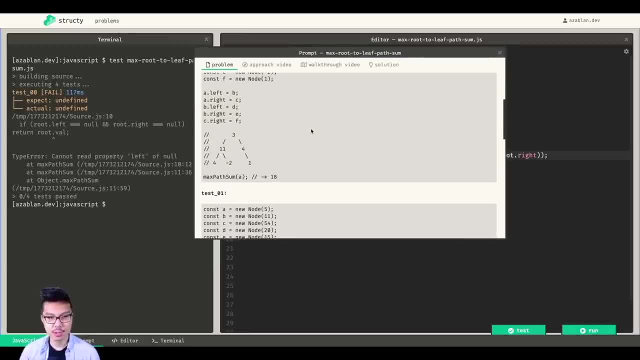 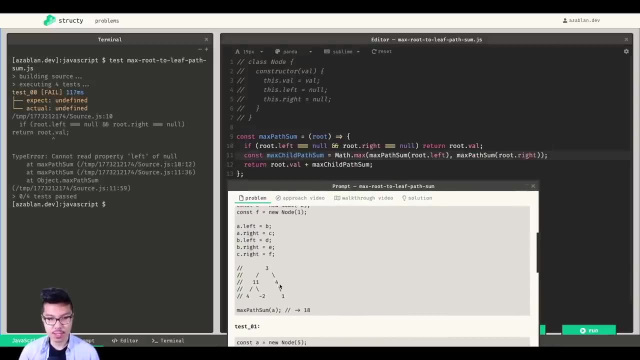 tell you that this is caused by an asymmetric node like this for over here, right, This for over here, And we're going to call this a right child And we're going to call this a left child, Right. So if we're evaluating this code, we know that our root is going to be this for node And 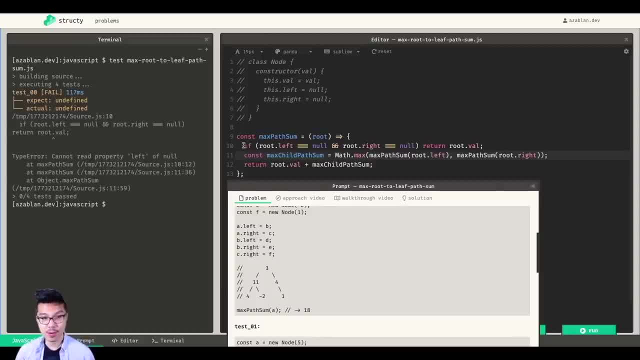 this: if statement on line 10 is not hit right Because four is not a leaf right Because it has a right child, its right child is not null, So instead it's going to run into line 11. And it's. 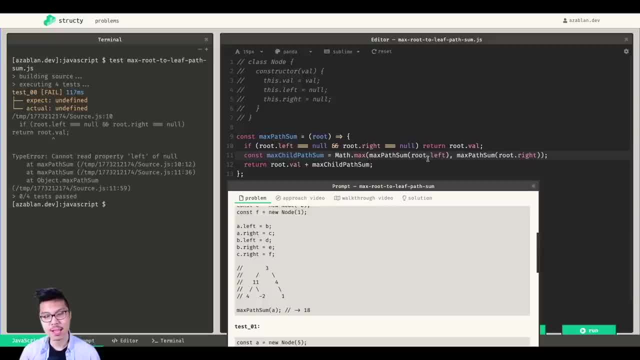 going to try to execute Max path: sum of root dot left. root dot left is null, And so when we evaluate that call now, we're seeing root is null And we're going to check null dot left over here And that's going to break right. It's exactly the line that's broken, And so, in addition to this, 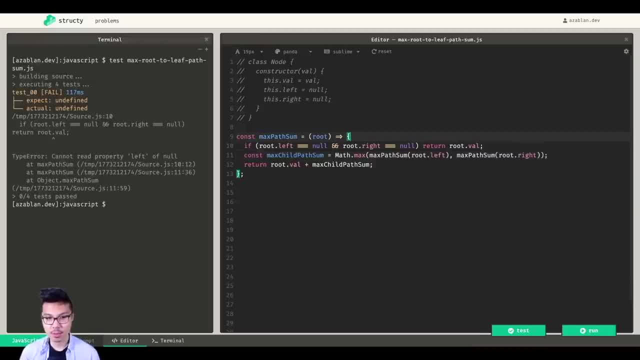 base case right, when we bought them out at a leaf node. what if we just end up at a null node? so if root is null, then we said that a good value to return would be negative infinity. right, Because I'm choosing to in the long run. do you like maximal logic? I'm going to want to pick. 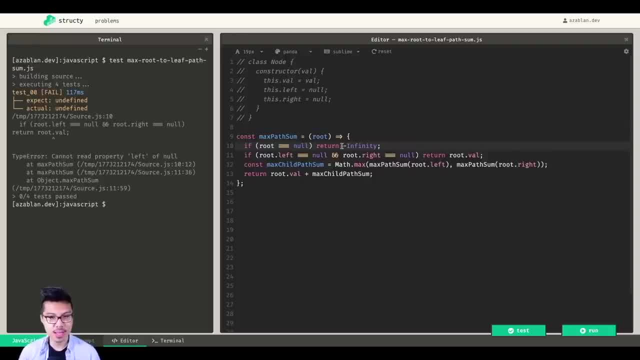 max. So if I choose a negative infinity, that won't interfere with any of us taking a max right, Because imagine that this thing was negative infinity and I would just prefer the right hand side if it was not infinity right, negative infinity that is. And so with 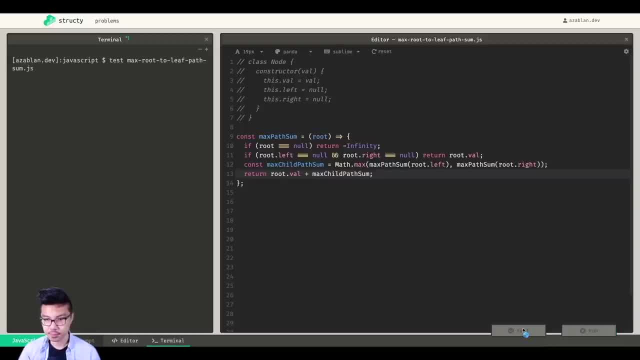 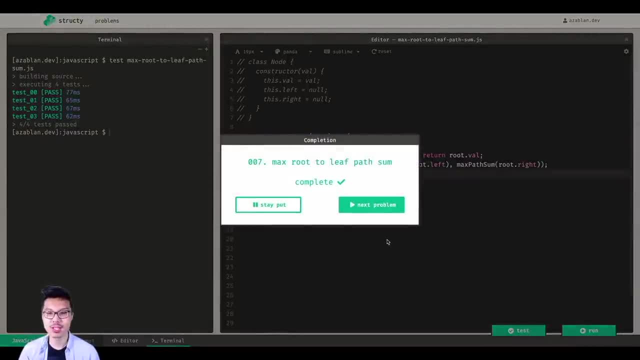 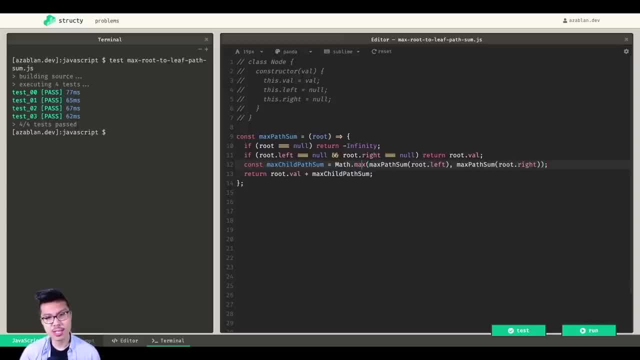 it's okay if it feels a little tough, But do understand how we have some familiar patterns right. I still have those two recursive calls right over here And we typically only vary in how we take those recursive calls or the results from them and combine them into our higher level. 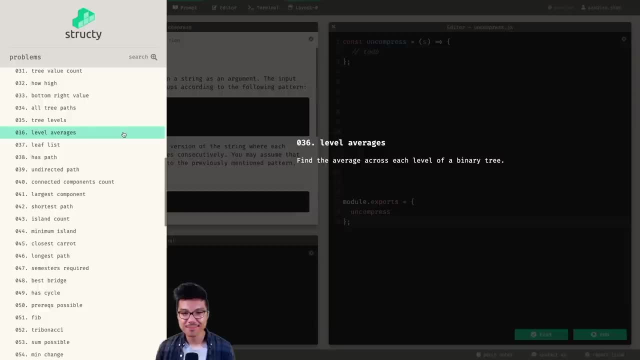 answer. So keep practicing this problem and I'll catch you in the next one. Alright, programmers. that wraps up our course on the introduction to binary trees. If you want to explore this binary tree topic, or really any other data structure and algorithm topic, more deeply, be sure to head.